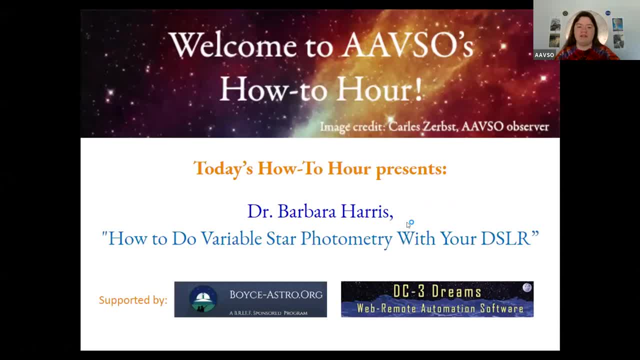 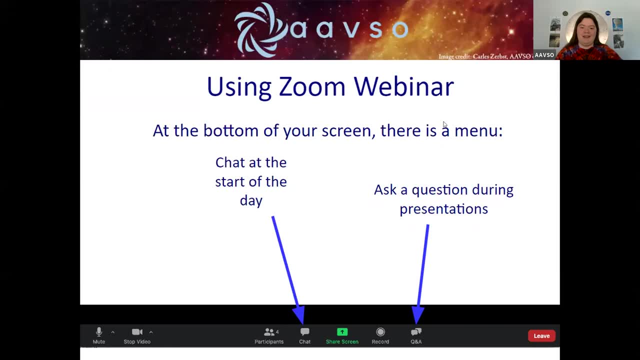 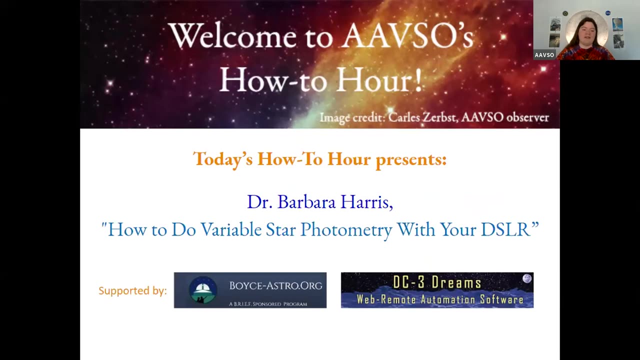 Welcome everyone. It is now 2 pm in Eastern Time, so let's go ahead and get started. So hello and welcome. as I've been saying, My name is Lauren Harrington and it is my great pleasure to welcome you all to today's How-To Hour. Now, before we get started, I have a few quick 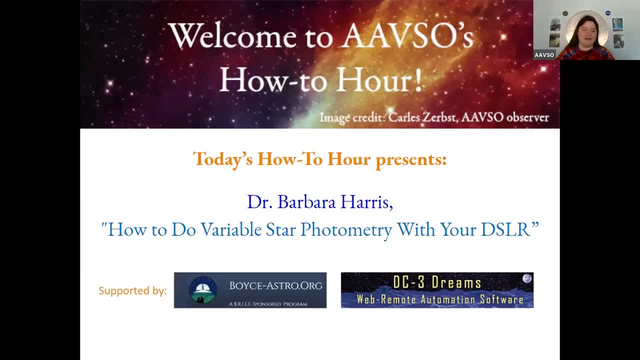 announcements to make. First of all, today's webinar will follow the How-To Hour format, which means that the first part of the session will consist of a presentation that's coming to you from one of our very own experts in the AAVSO, and after that we will have an extended 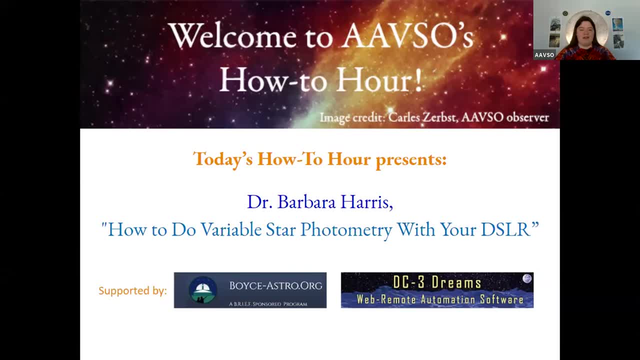 Q&A session. During that time, we'll try to address all of the questions from the audience. So if you are interested in DSLR photometry and you have some questions that you've always wanted to ask an expert, today's your lucky day. All you have to do is click on the little icon at. 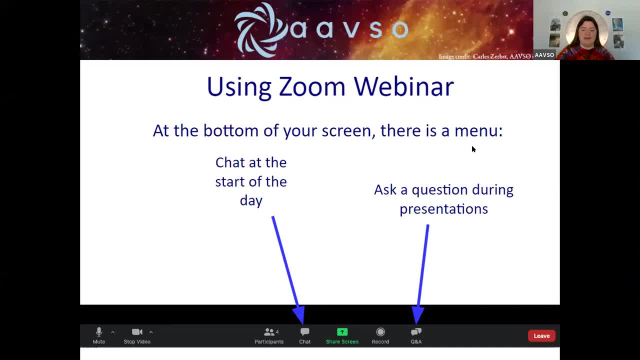 the bottom of your screen that says Q&A. type your question into the box that appears and hit submit. You can submit as many questions as you want at any point during the How-To Hour. Don't worry, it's not going to interrupt the presentation if you do so during the presentation. 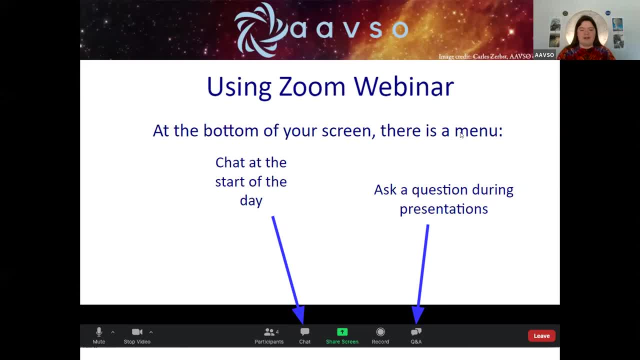 Next, if at some point during the webinar you experience technical difficulties with audio, we are unfortunately not able to help from here. However, you might be able to fix your audio yourself by clicking on that little up arrow button that's next to the mute icon in the bottom. 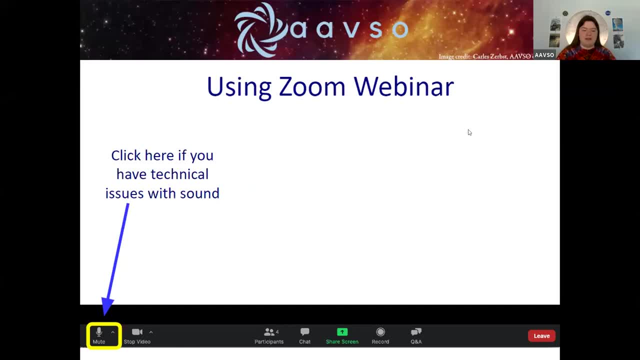 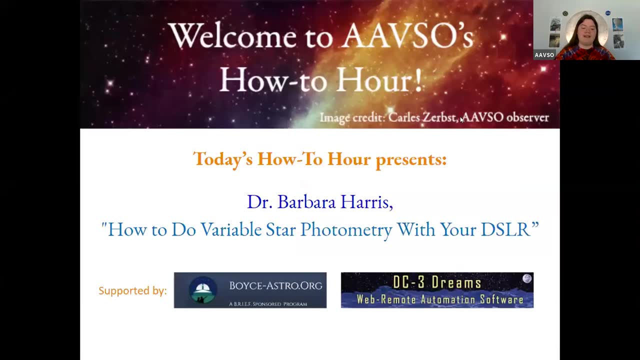 left of your Zoom window. Finally, we would like to thank and acknowledge our sponsors DC3Dreams and VoiceAstro. DC3Dreams provides high-end observatory automation and web-based multi-user remote imaging. The AAVSO Net Observatories use DC3Dreams, ACP Expert for the Bright Star Monitors and other. 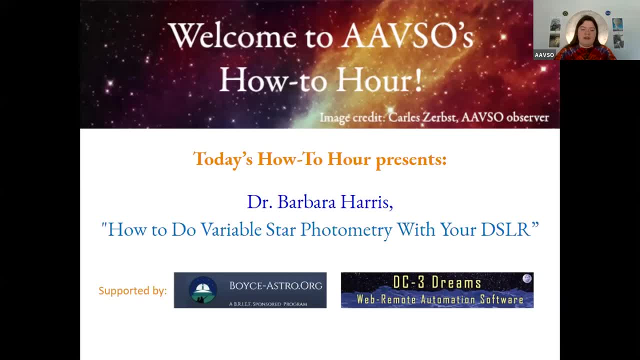 programs. The AAVSO Photometric All-Sky Survey provides high-end observatory automation and web-based multi-user project, also known as APAS, has used ACP Expert's AI scheduler to automatically acquire over 500,000 star fields hands-off at a rate of 1,000 square degrees per night. This has resulted in 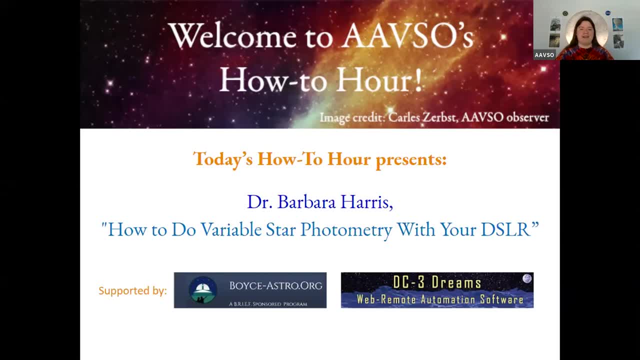 photometry for over 128 million objects in about 99% of the sky. The Boyce Research Initiative and Education Foundation provides online astronomy education, observatory resources and research experiences to students, student teams and schools in order to learn how to perform observations, conduct research and publish their results in. 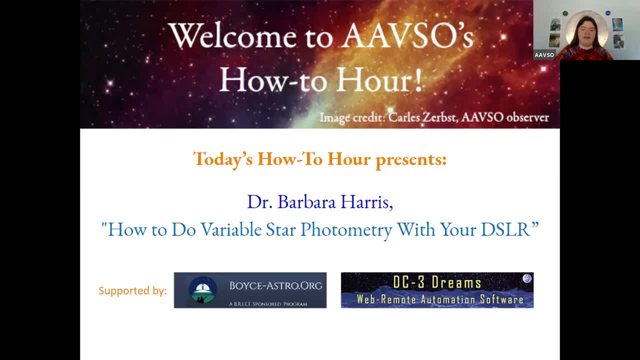 scientific journals such as the Journal of the AAVSO. Please check out their webpage to learn more about their work. All right, without any further ado. ladies and gentlemen, please allow me to introduce your instructor for the next hour. She's a retired physician with an interest in astronomy. that. 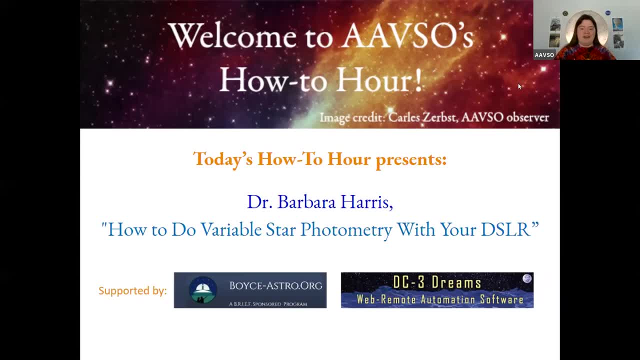 dates back to her days in high school. She got her first CCD camera in 1999, and decided she wanted to put it to good use doing some real science. so she learned how to do photometry. Six years ago, she added a DSLR to her photometric toolkit. 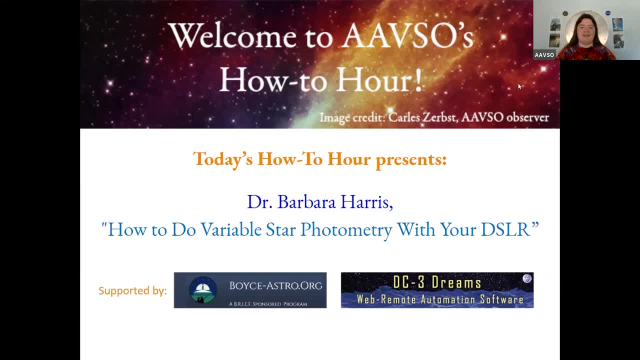 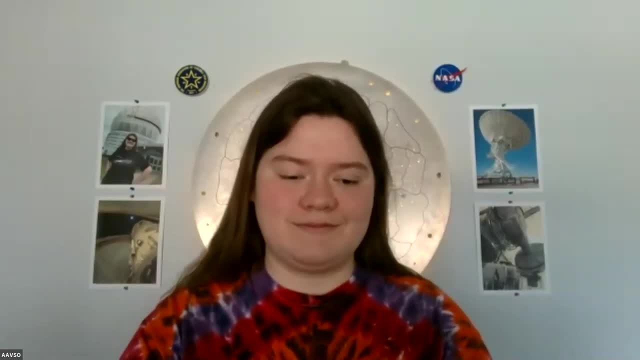 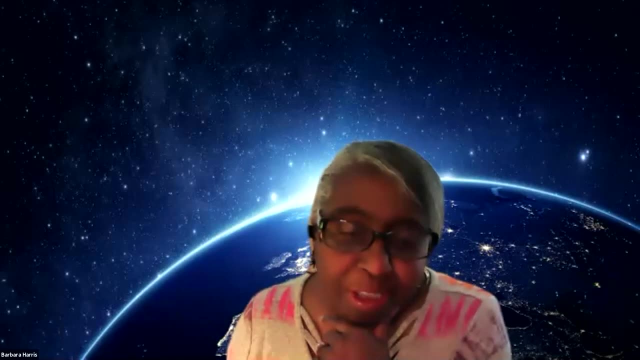 and today she'll be teaching us all about the ins and outs of DSLR photometry. Ladies and gentlemen, please give a warm welcome to Dr Barbara Harris. Hi everyone, I noticed a few names in the participant list were some of my. 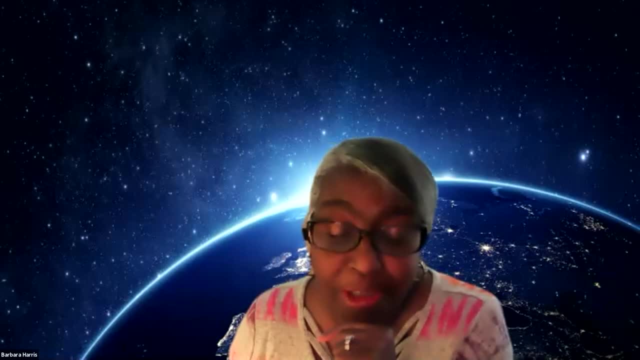 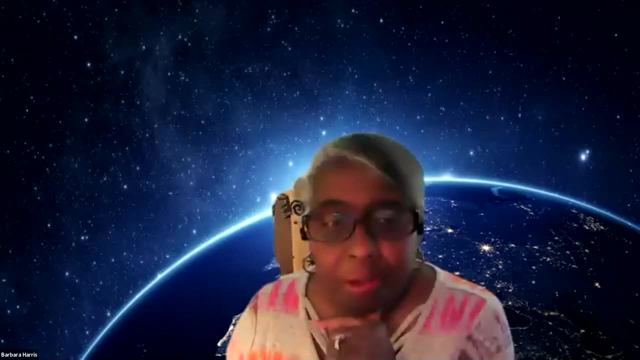 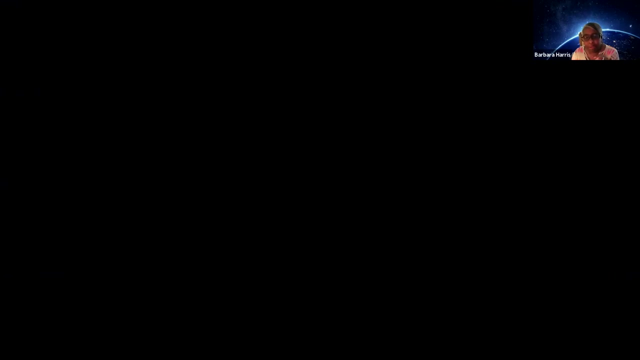 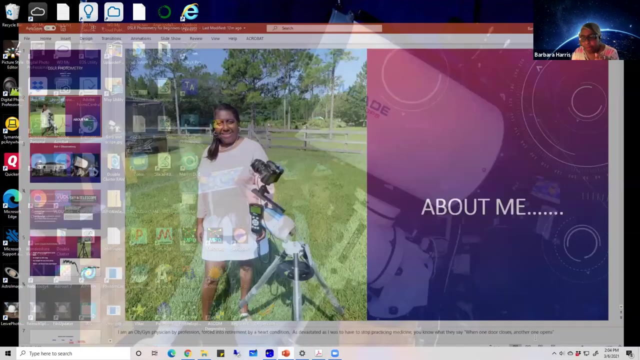 students that I was mentoring, so it's kind of nice to see some familiar faces participating. So today I'm going to talk about DSLR photometry and I'm going to basically hit on the key points, because everything I talk about is going to be available in the DSLR manual that you can. 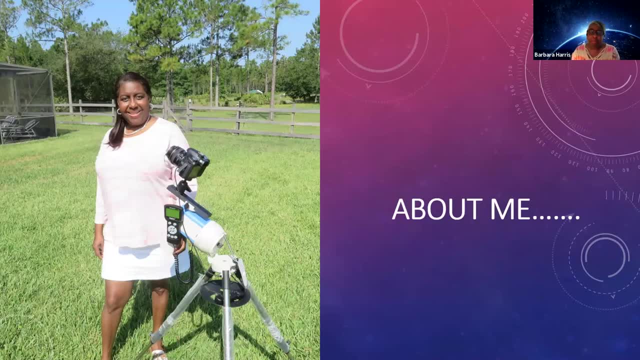 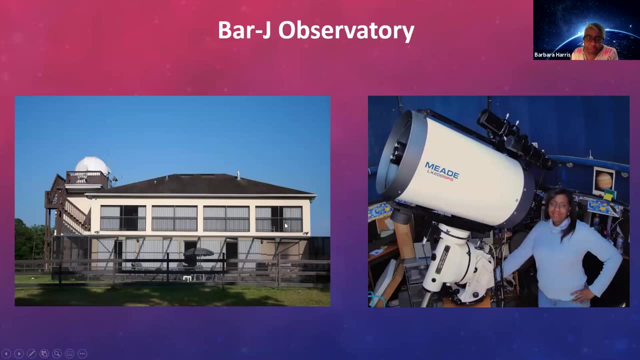 download from the the AAVSO website. So Lauren has given a great introduction of who I am. I'm a retired physician. I live in Central Florida, halfway between Orlando and Daytona Beach. I have a third story observatory. that's a 10-foot dome. 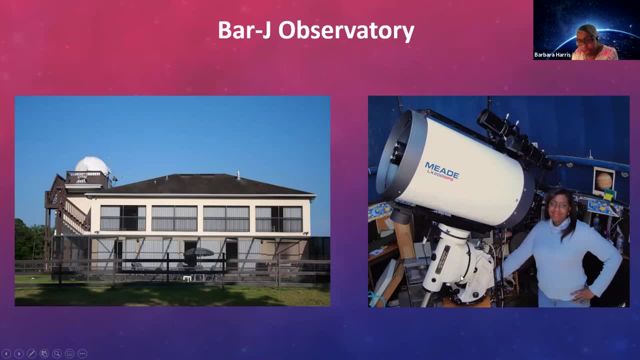 housing a 16-inch Schmidt-Cassegrain on a 1200 astrophysics mount. This has a proline CCD attached to it and this is how I do my CCD photometry. I also have a 80-millimeter refractor on top of that, with the Canon 40D attached to that. 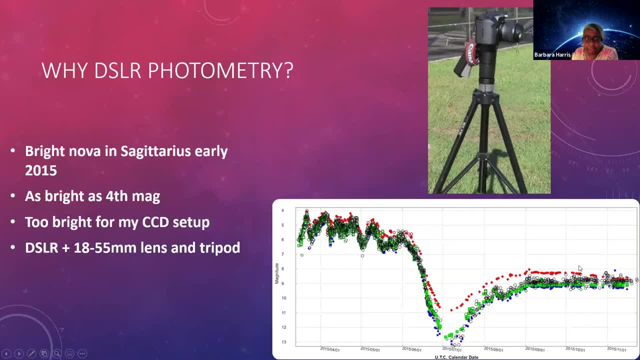 and I do some DSLR photometry with that set up. So I've been doing CCD photometry for about 20 years. so why did I add DSLR photometry to my my toolbox In 2015,? there was a bright nose in Sagittarius. It became really bright. 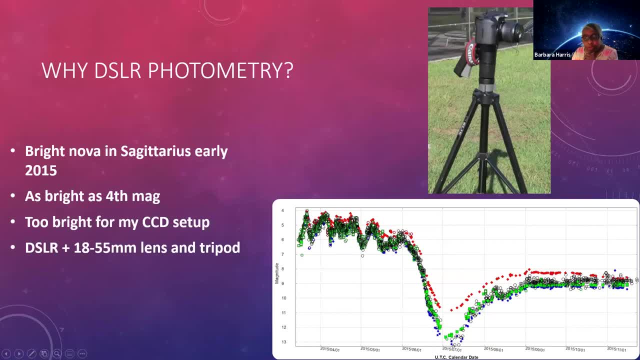 as bright as fourth magnitude and I wanted to be able to do photometry on it, But it was too bright for my CCD and 16-inch telescope setup, So I decided to put my DSLR to good use, because there had been a lot of activity. 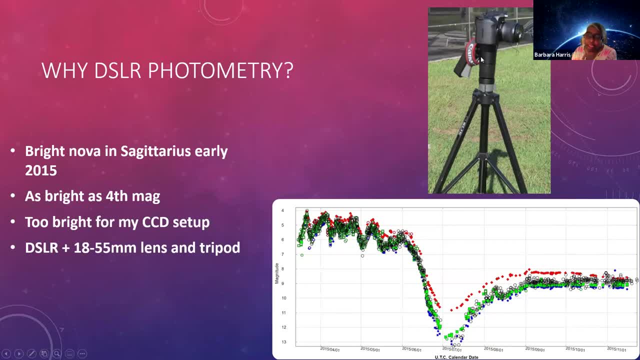 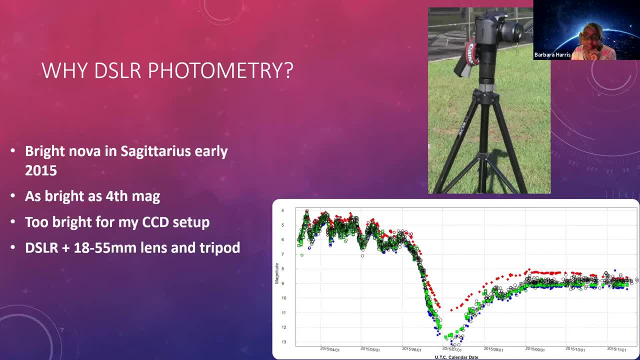 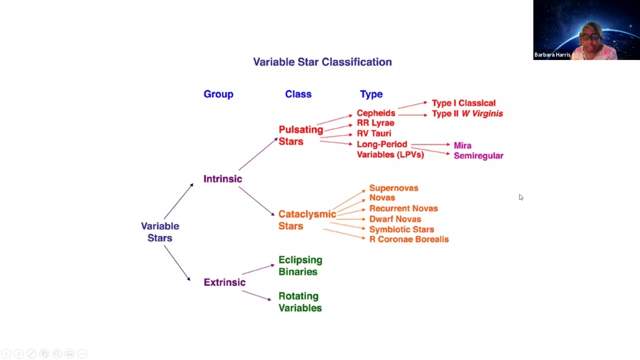 where they instructed people on how to do DSLR photometry. So I put my Canon 40D and an 18 to 55 millimeter kit lens on a tripod to good use obtaining data on this particular Nova. So what class of variable stars are amenable to DSLR photometry? 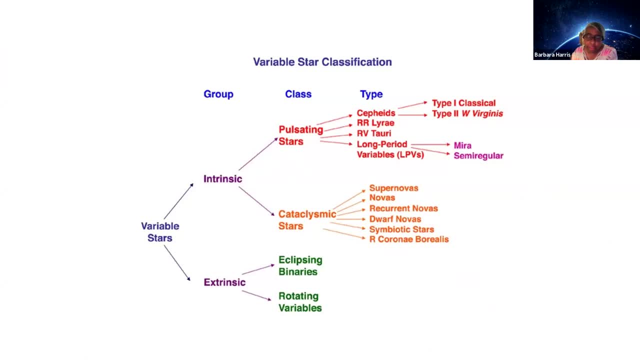 Theoretically, any variable star can be amenable to DSLR photometry as long as it's in the magnitude range of your equipment. I love to do eclipsing binaries and I've done light curves of eclipsing binaries with DSLR photometry. 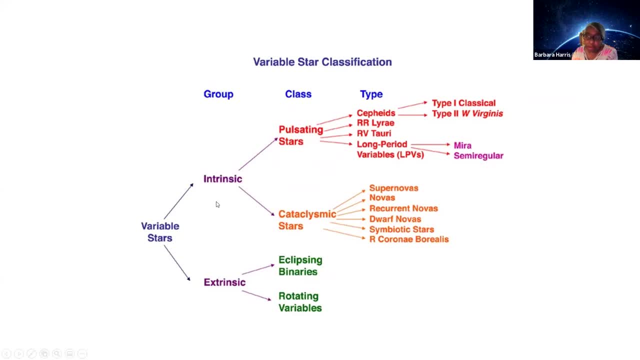 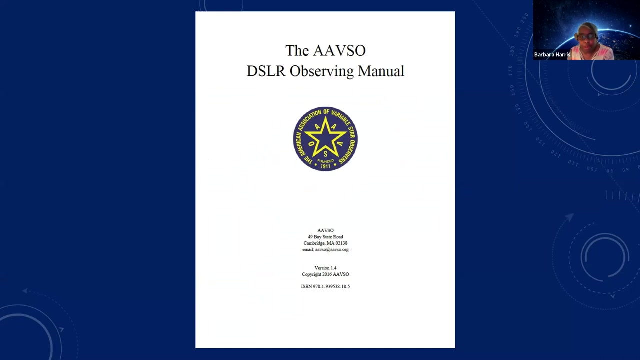 I like to monitor very bright variables like Betelgeuse, especially last year when Betelgeuse underwent that unusual dimming period. I was able to monitor it with DSLR. So, like I said, everything I'm going to talk about today is in the AAVSO DSLR observing. 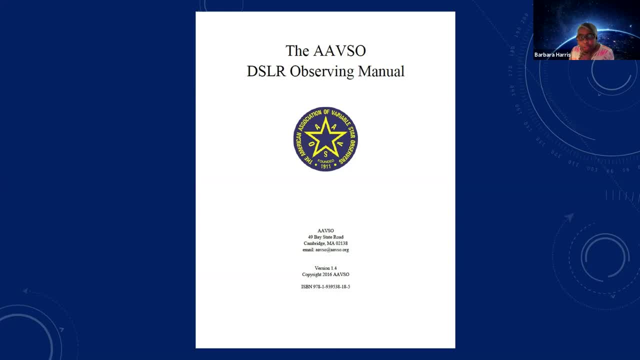 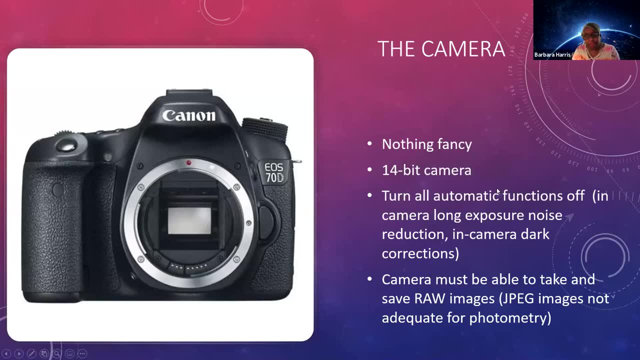 manual, And you can download this for free from the AAVSO website. Let's talk about our equipment. The first thing you're going to need is a DSLR camera, And many of you may have a DSLR that you use for general photography or pretty picture. 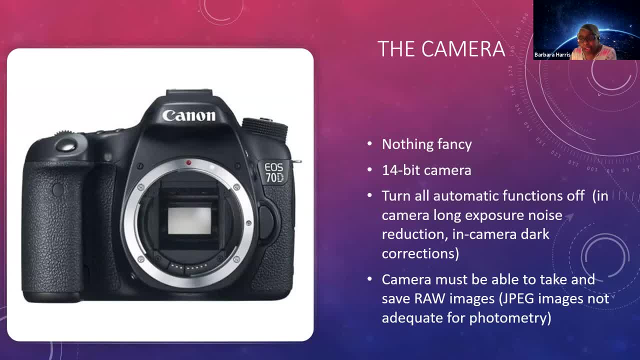 astrophotography. If you don't have a DSLR and you're thinking of buying one, you don't need to go out and buy the fanciest DSLR out there. In fact, we want something that's very basic. Um, most of today's DSLR cameras are very basic. 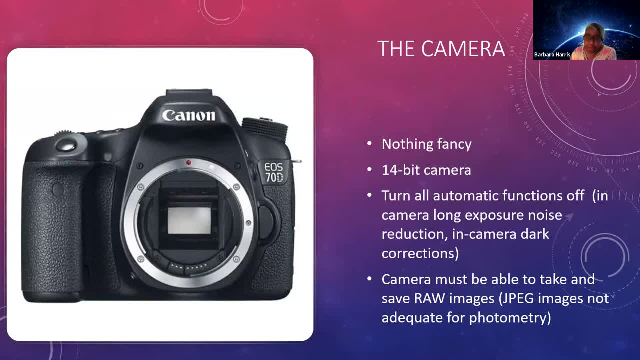 Most of today's DSLR cameras are very basic. Most of today's DSLR cameras are very basic. Most of today's DSLR cameras are 14 bit cameras. but even if you have an older 12-bit camera, you can still do photometry with that camera. 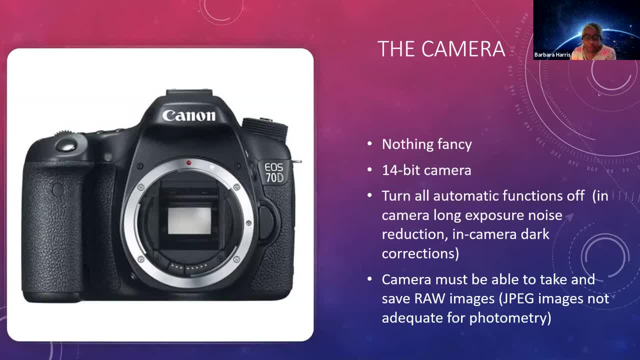 The thing that you're going to have to do with doing photometry is you want to turn off all the automatic functions that that are involved in your, your camera, and we're talking about things like long exposure, noise reduction or in-camera dark correction. 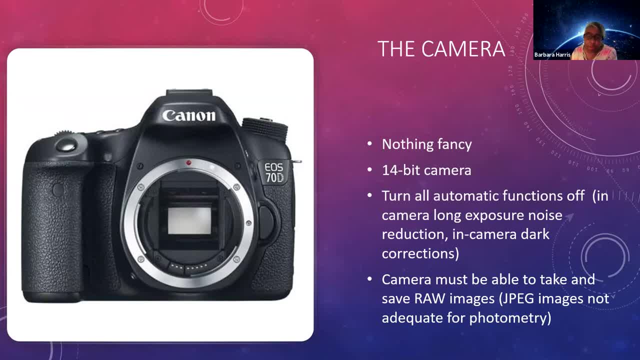 You don't want any of that on when you're capturing your your images. The big key to your DSLR is that it must be able to save the images in a raw format. JPEG images are not amenable to photometry, so you need to save. 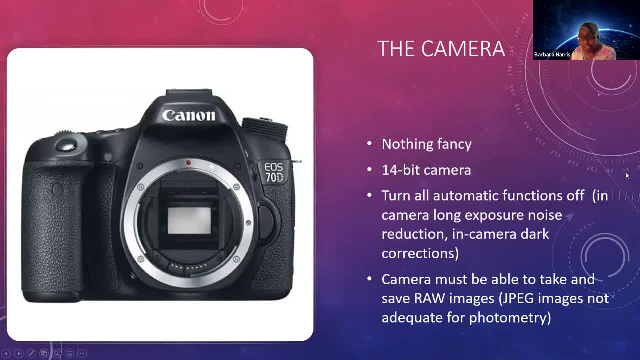 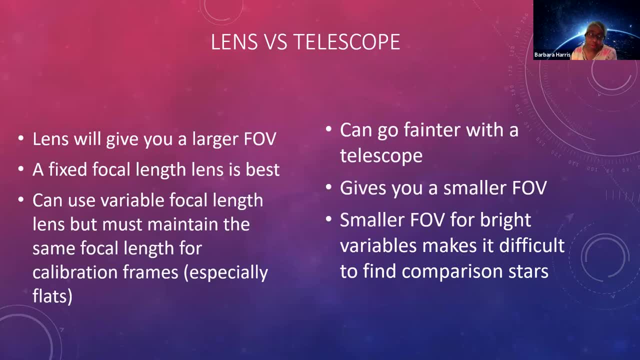 your data and be able to to, your camera needs to be able to save it in a raw format. So, now that you have your camera, you have to decide what to attach the camera to. Is it going to be a lens or a telescope? One of the advantages of having a lens attached to the camera. 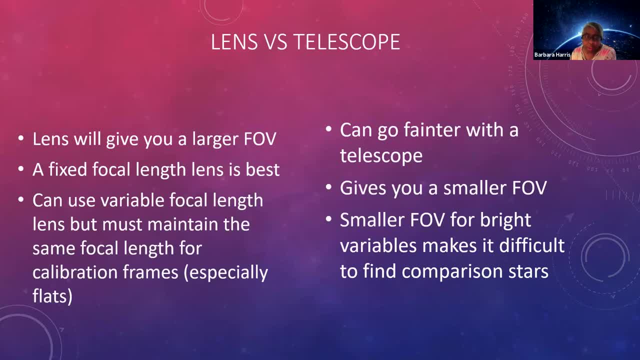 is that a lens will give you a larger field of view. When you have a larger field of view, you have a better choice, a larger choice of comparison stars to measure your variable width. If you're going to use the lens, ideally a fixed focal length lens is best, but even with care you could use a variable focal length lens, like when: 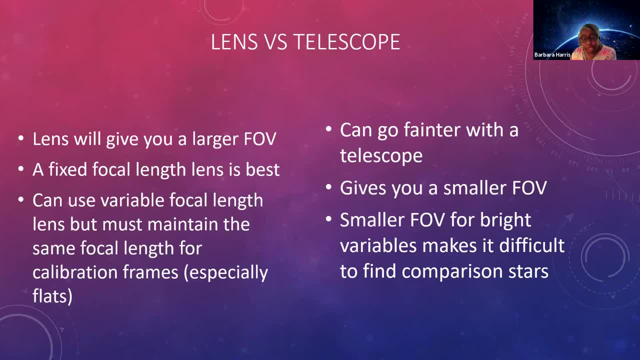 I first started with DSLR photometry. I used an 18 to 55 millimeter variable focal length lens. When you use a variable focal length lens, you have to be careful to make sure that you don't change the the focal length or the focus position, because when you take your flat fill, 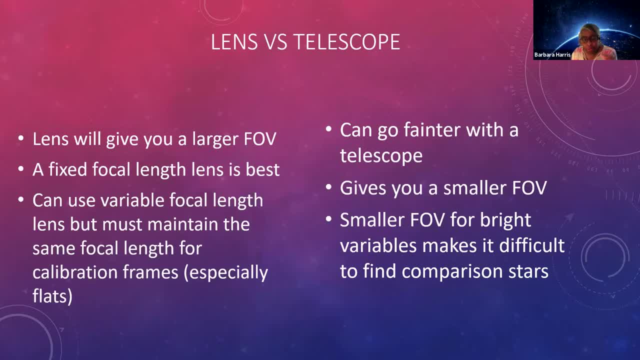 calibration images, your, your focus and your focal length. everything needs to be the same setup as your science images. The advantages of having a telescope attached to your camera is that you can have fainter stars to work with. With the telescope, you can, you can, you could expose for a longer period of time. The 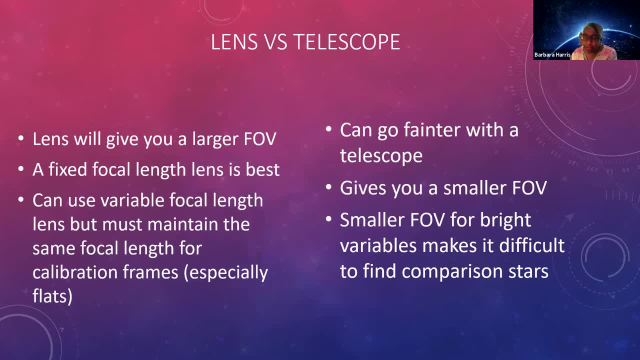 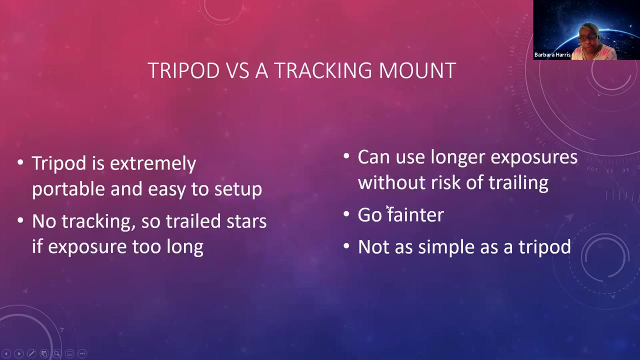 advantage of having a telescope is that it's a smaller field of view. so if you have a very bright variable with a telescope, it's going to be hard because you need very bright stars for a comparison star. Now, once you have your camera and your lens or telescope, what are you going to put it on A? 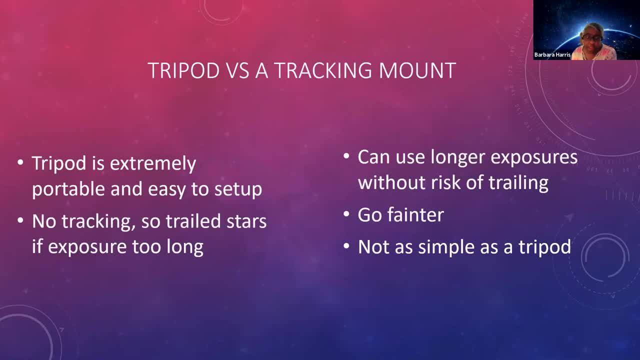 a tripod or a tracking mount. Tripod is extremely portable and very easy to set up. When I was monitoring Betelgeuse last year, it was easy for me to just take my tripod outside, point it at Betelgeuse, collect my images. 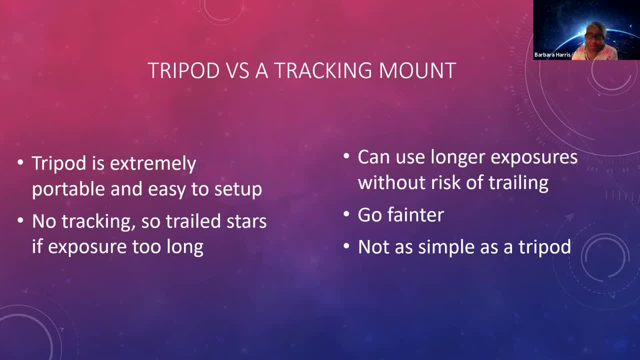 and I was back in the house within 10 minutes because it's very easy to set up. The disadvantage of a tripod is that there is no tracking, so you're limited to how long of an exposure you can get with the camera on a tripod. 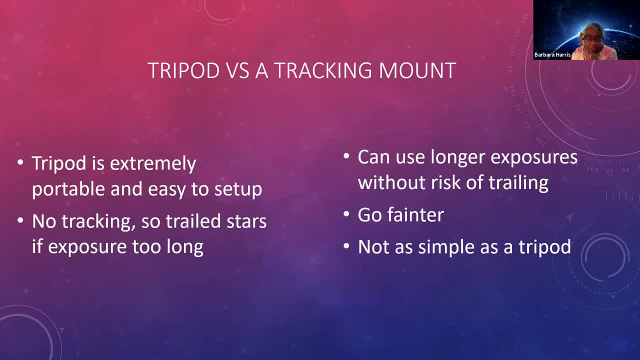 With Betelgeuse I was only doing 10-second exposure so I didn't have to worry about trailing. But you probably can't go more than 20 to 30 seconds without getting significant trailing, So in a tripod you're limited. 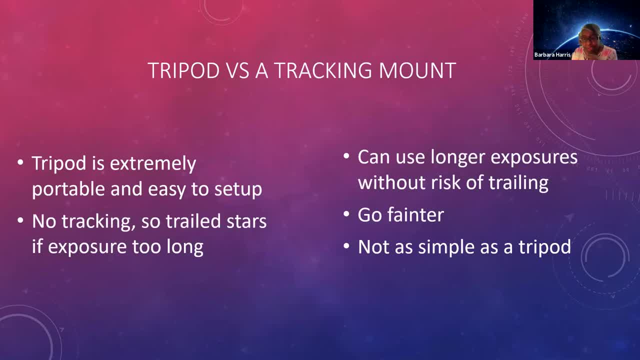 by the to the, the very bright stars. The tracking mount is great because you can track your target and that means that you can go longer with your exposures. It also means that because you're going longer, you could- you could- avoid trailing. 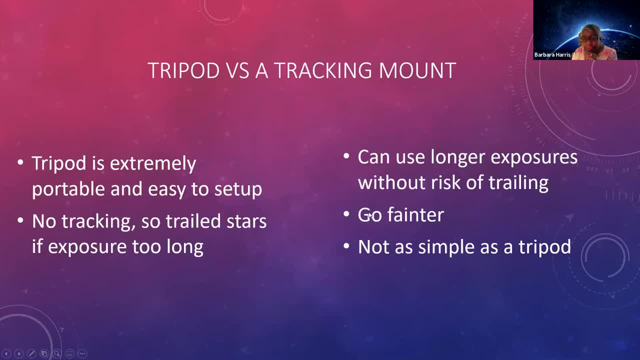 And because you can go longer in your exposure, you can go fainter and have a target, a lot more stars to select from. as far as doing photometry with, The disadvantages of having a mount is that it's not as simple as a tripod. 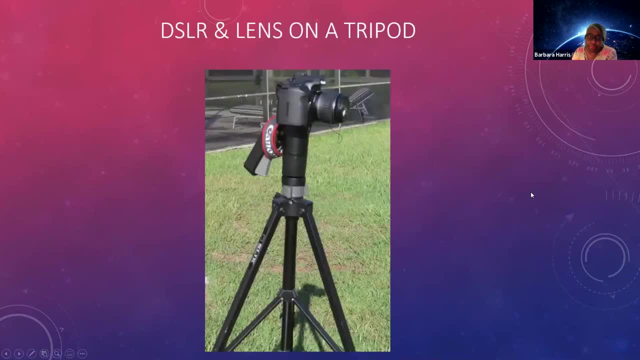 So it it requires a little bit more effort in setup. So, like I said, this was my first DSLR setup and I still use a tripod today for very bright stars, except for instead of an 18 to 55 millimeter lens. 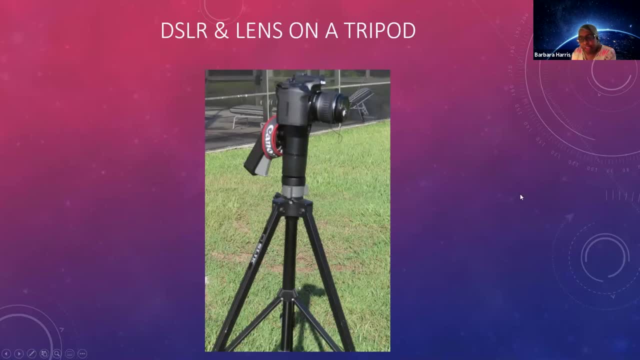 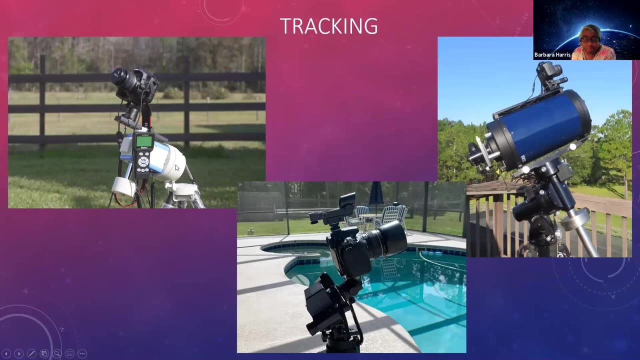 I use a 85 millimeter fixed lens And as far as tracking, I use this little smart Ioptron SmartStar mount. I also have an Ioptron SkyTracker Pro and sometimes I just set my telescope up, my camera, up on top of my telescope. 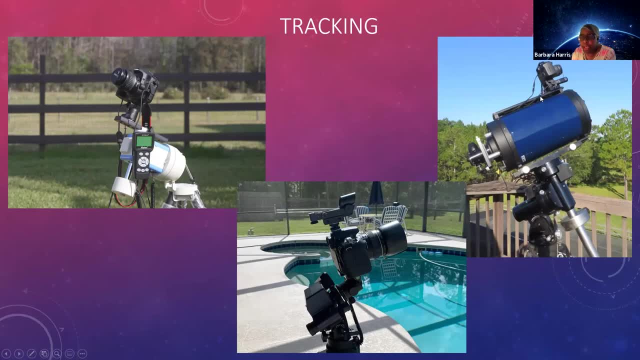 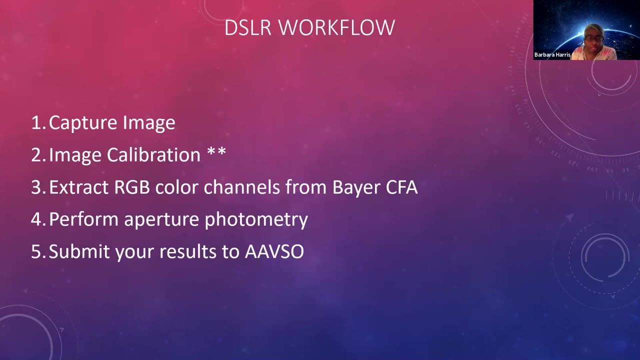 On my deck I have a Meade on a Mach 1 mount And sometimes I just put my lens in and camera on that and just use the mount for tracking. So as far as the workflow of DSLR, first you're gonna capture your image. 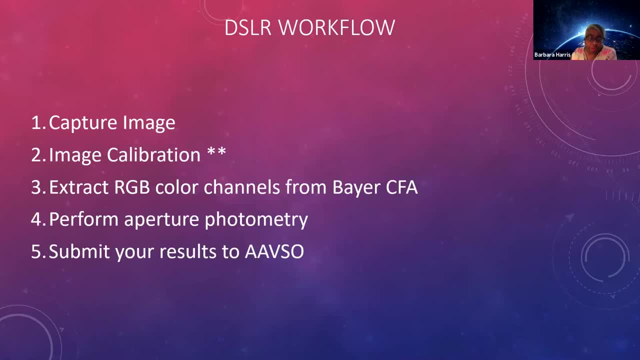 Once you capture your image, you also are going to capture calibration frames, which are bias, dark and flat field frames, And if you're used to doing pretty picture astrophotography, you may not worry about doing complete image calibration. 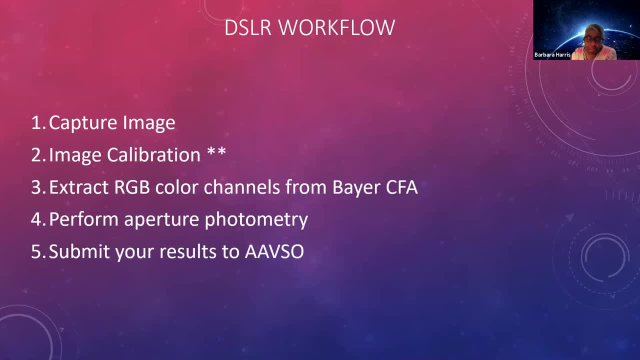 especially flat fields. but it's important when you're doing science images, to do complete image calibration, including flat field. Once you've captured your images and you've collected your calibration images, the next thing you're going to do is you're gonna take your raw image and extract the color. 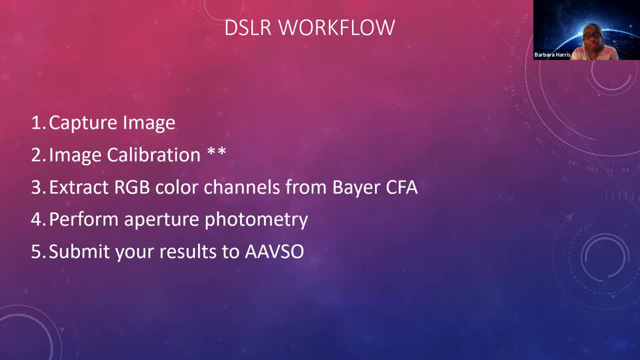 channels from it And then you're gonna do photometry on those color channels And we'll go into a lot more detail for this- And then you submit your photometry results to the AAVSO. One reason that I have an asterisk by image calibration. 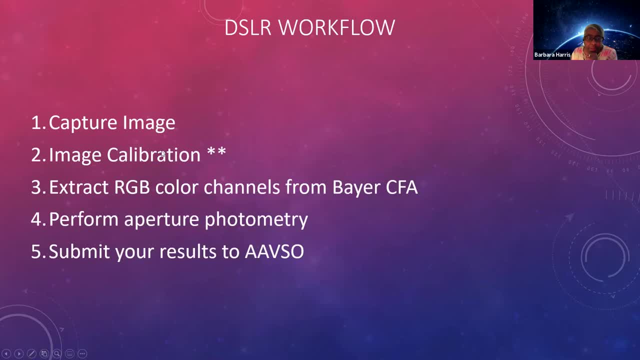 is that, depending on your software, some software packages may require you to extract your color channels And then apply image calibration to each color channel separately, So the number two and number three may be switched depending on what software package you use. Most of what I use is in this order. 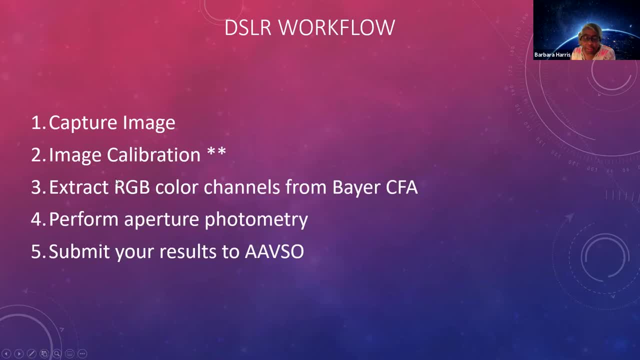 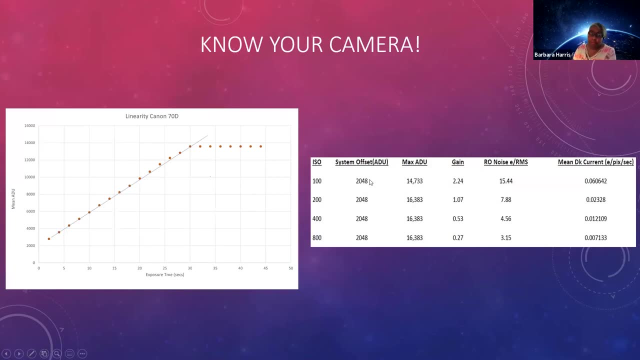 in that you do image calibration and then you separate out your color channels after you calibrate your image. Now, also, before you go out and take your images, one thing that I recommend is look in appendix A of the DSLR manual and on page 93 of the DSLR manual. 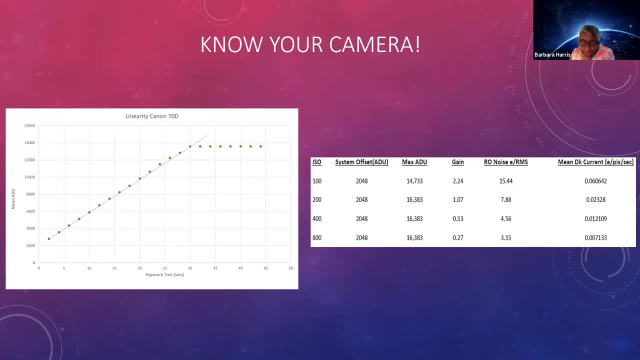 it's called DSLR camera testing, And what you're going to do here is basically determine one: what the system offset is for your camera. Every camera has a has a system offset, meaning that for a 14 bit camera, you have a shade of going from zero to 16,384.. 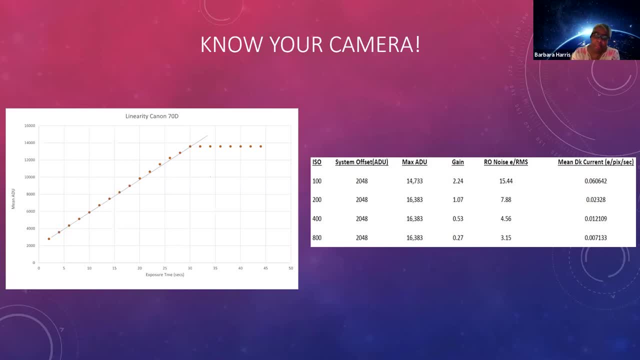 But there's a system offset. instead of it starting at zero, it starts at a certain number above zero. So for my Canon 70D my system offset is 2,000.. So the lowest your ADU reading is going to go is 2,048.. 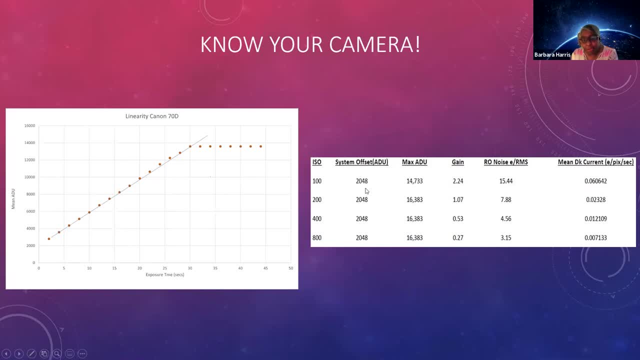 For my Canon 40D the system offset is 1,024.. So in your DSLR camera testing in appendix A you're going to determine the system offset of your camera. The other thing you're going to do is to measure the maximum ADU. 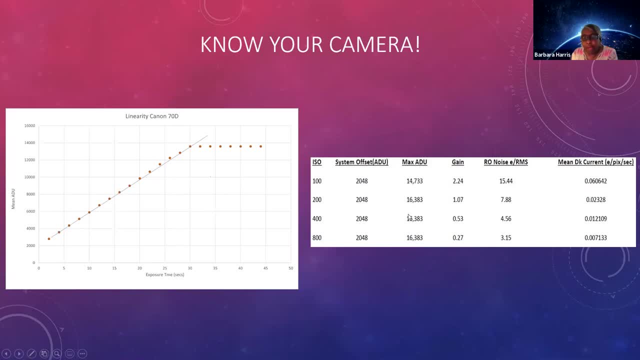 The other thing you're going to do is to measure the maximum ADU. The other thing you're going to do is to measure the maximum ADU of your camera, Like what? what is the maximum value that you could obtain? And it actually is different at ISO 100,. 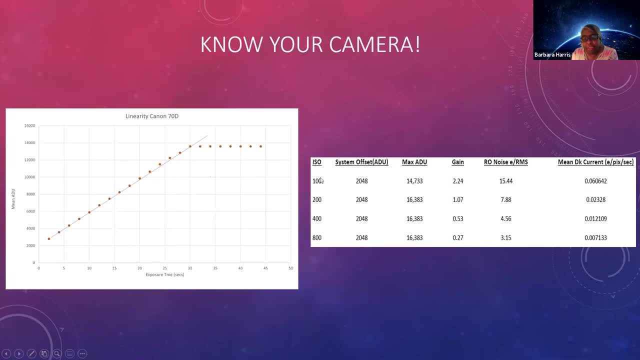 compared to the other ISO levels. Now I've tested ISO 100 to ISO 800.. And for photometry you're probably not going to go over 800 ISO, So just going from 100 to 800 in your testing it's adequate. 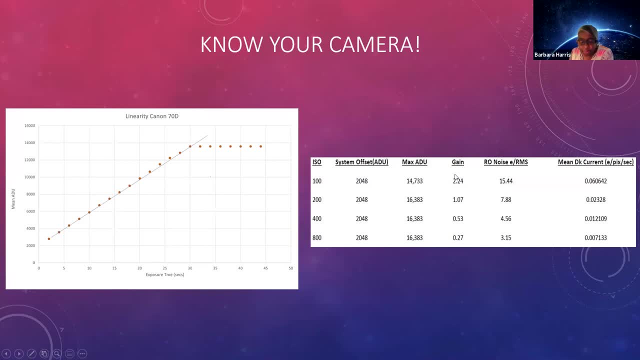 The other thing that you're going to test in appendix A is the gain, And the gain is basically: how many electrons does it take to move one ADU in your, in your image? And this is different depending on the ISO level. So by changing the ISO level, 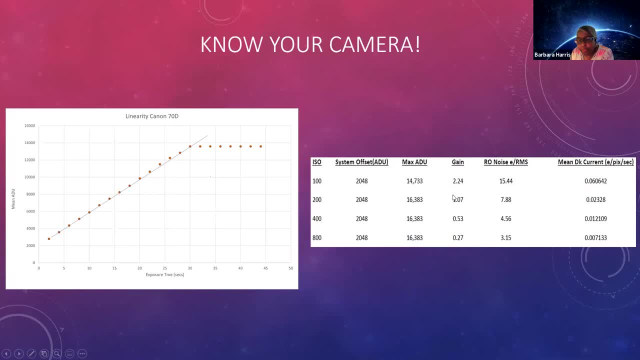 you're basically changing the gain of your, your camera, And what you want to do for photometry is select a gain that's closest to one. So for my Canon 70D, ISO of 200 gives me a gain of 1.07.. So most of my photometry is done here at ISO 200. 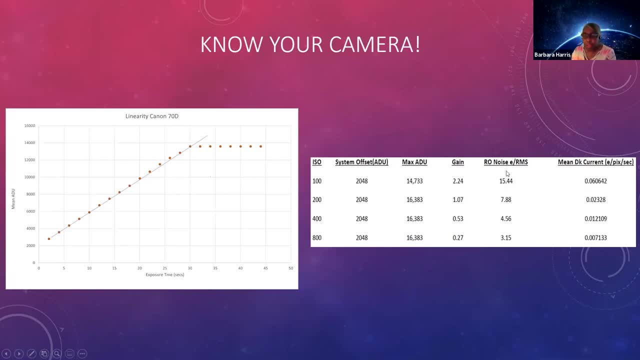 So those also in the appendix. it has you checking readout noise for each ISO level also. But the most important thing in that appendix is the system offset the maximum ADU and the gain at each ISO setting. Now the other appendix item you should do before you start taking images is- I think it's- 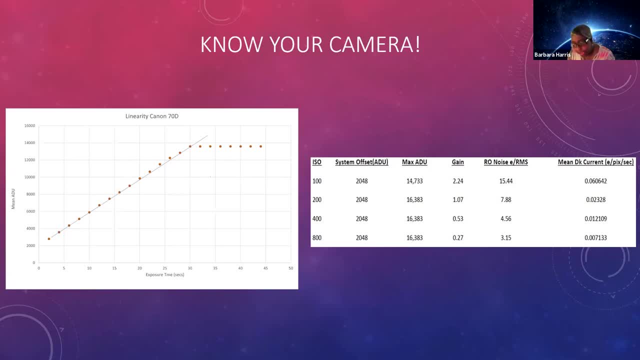 appendix- I think it's E in the DSLR manual, And basically what it's telling you to do is to check the linearity of your camera. Photometry works because digital cameras are linear, meaning that for a certain exposure time it's going to increase the ADU value a certain amount And you can plot this. 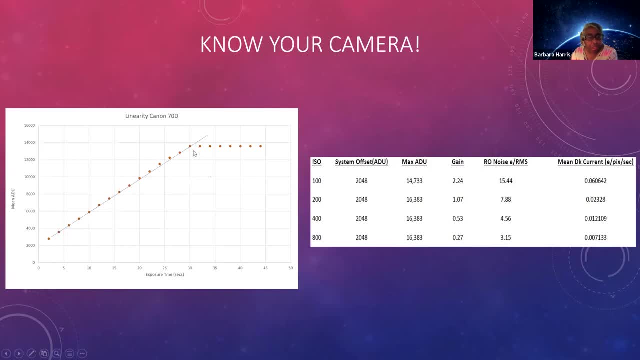 away and then rub it in so you can Su crease the blurb on the queues And it should give you a linear curve up to a certain point. And I've done the linearity curve for my Canon 70D And this was done. 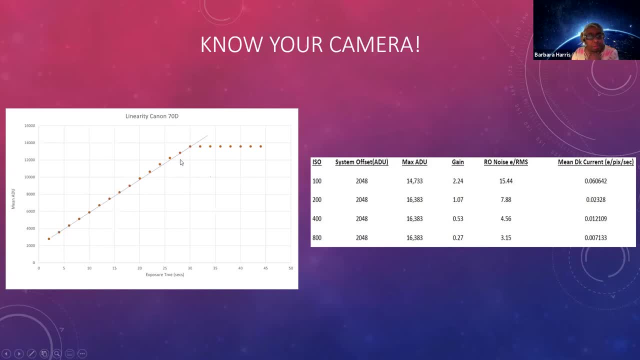 at ISO 100. So it's going to saturate at about 14,000 for my ISO 100.. If I had done it at 200 or 400, it would saturate closer to 16,000.. So, like with that kind of situation, you could get there. but you're ending up with a issues of taking images of just 40,000 Transform or 15,000 JapanWorld tapi formats, which is that in rочно or anywhere else, So for just about everybody else, we'd do it at. 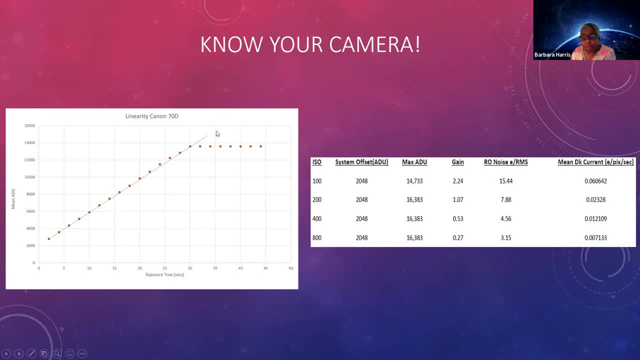 50%江 black, or as great as that value in theẩm, the thes, or, as I would do it, by taking isto 너 ADU. But these are important items that you should do before you start taking your images to know what ISO setting to use and to make sure that you stay in the linear region of your camera. 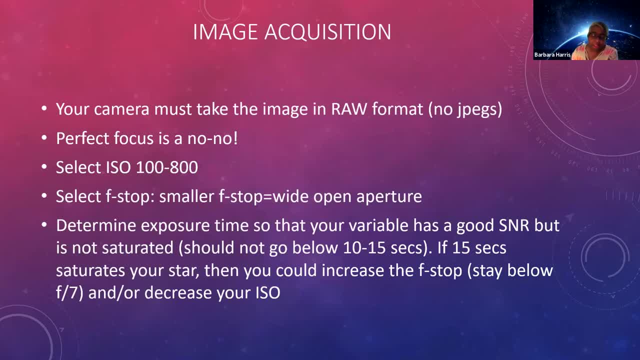 But once you've done that and you want to go out and take your images, you figure out what your target is going to be And you set your ISO value depending on the previous slide. Like for my Canon 70D, my ideal ISO setting is going to be 200.. For my Canon 40D, my ideal ISO level is going to be: 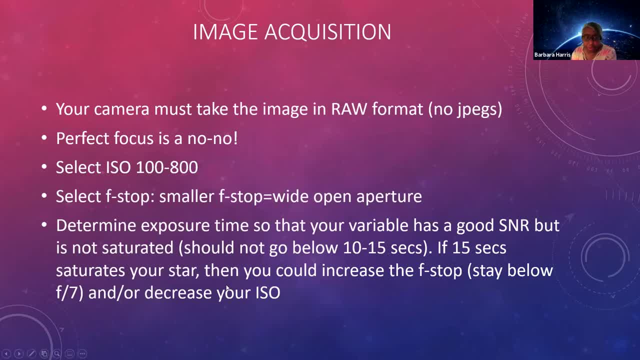 400.. So you set your ISO to one of those values. The other thing that you concentrate on in pretty picture astrophotography and general photography is that you want the best focus possible In DSLR photography. you don't want perfect focus. You actually are going to. 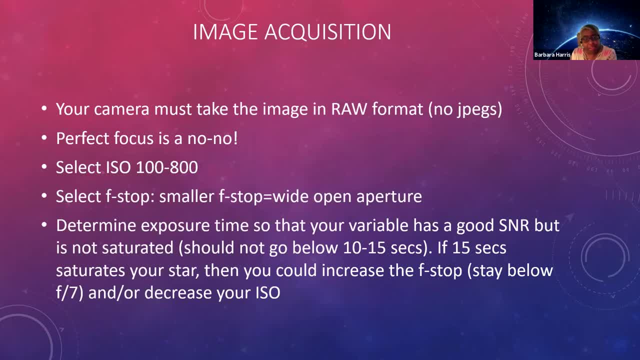 defocus your image so that your starlight is spread out over several pixels. So it's contrary to what most of you have been doing, If you've been doing astrophotography. So we'll talk about it a little bit in software. But 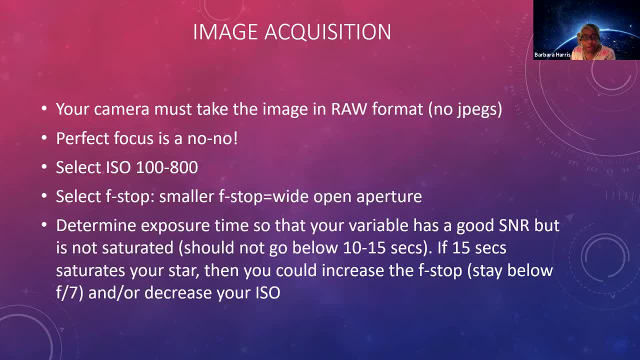 in your software. you have to be able to measure how wide your star image is to make sure that it's spread out over enough pixels, Because if it's finely focused, if it's too focused, your photometry may suffer because you're under sampling your star. 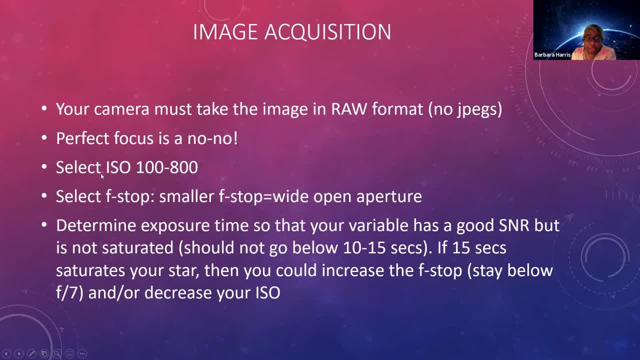 image, So you want to be able to measure how much you can focus, and you want to be able to make a product that is one step further than the average, And so that's pretty much all of it. And then the last thing that I wanted to talk about is how to set the aperture on the lens. 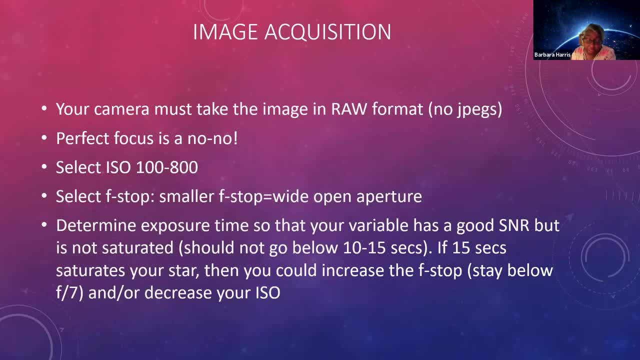 And for the reason I mentioned just in the video. this is a very popular question, but it's very common And the reason I mentioned this is because it would be easier to see in the video, even if you've got the camera with you. but if you want to set the 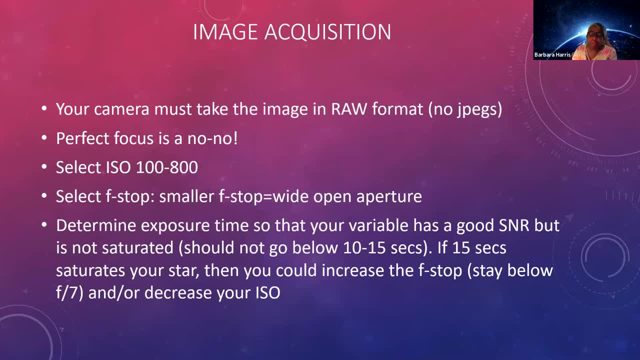 aperture. with a smaller lens you would have to set it like if you're pointing the lens at a certain angle, you'll have to set the aperture a little bit farther. And if you have a very wide open aperture, saturate really quick. So for very bright targets usually you increase the f-stop but you want to. 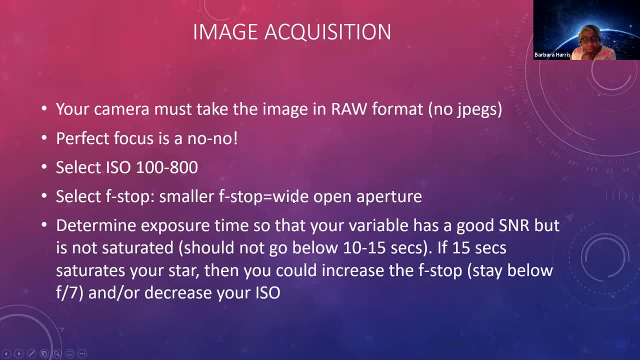 stay below f7. So you don't want to go higher than that. So, with a very bright star, you want a higher f-stop than a wide open aperture. The other thing you need to do is you want to determine what exposure time you need, And this takes some practice and after some practice you can get an. 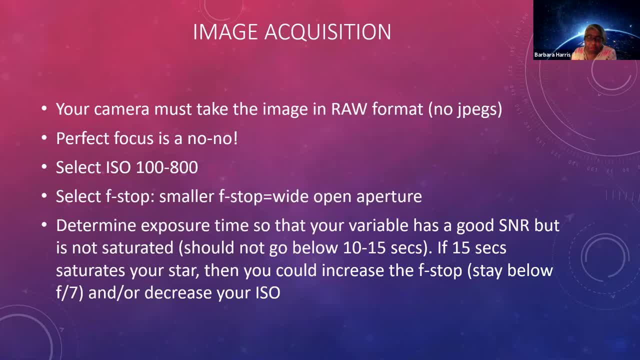 idea of you know it looks like the variable is about seventh magnitude, So you have an idea of how much time it takes to expose to get a good signal to noise ratio of your target. And you want a good signal to noise ratio of your target but you don't want to saturate your target and not 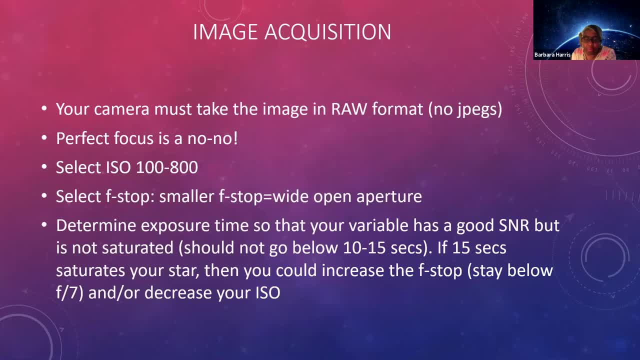 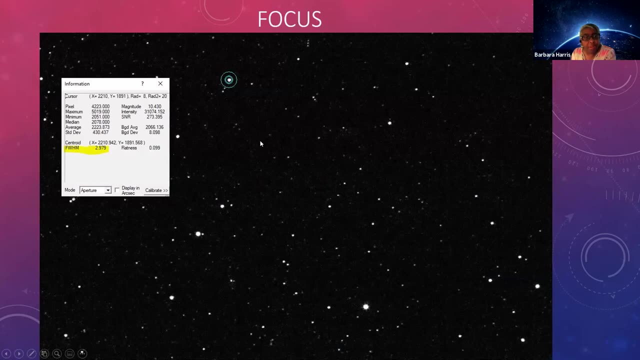 just your target. You want to saturate your target, So you want to saturate your target. But you should have an idea of what stars you're going to use in your field so that you don't saturate your comp stars also. So this is one of my images of Delta Cephei. I follow this star pretty. 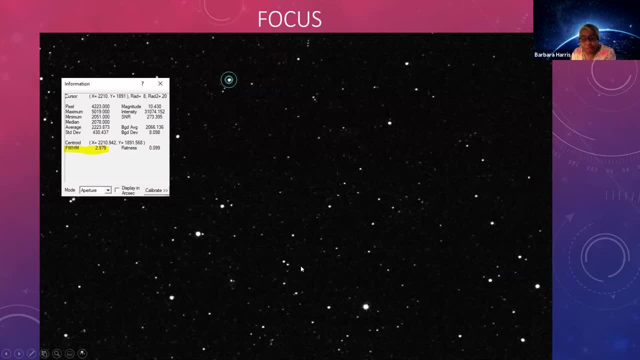 regularly, And this is actually a very focused image of the field. The star that you see here is very nice and focused, And I usually do my photometry in maximum DL. So what I do is when I look at my target and I have aperture rings around my target, which is Delta Cephei, and we measure. 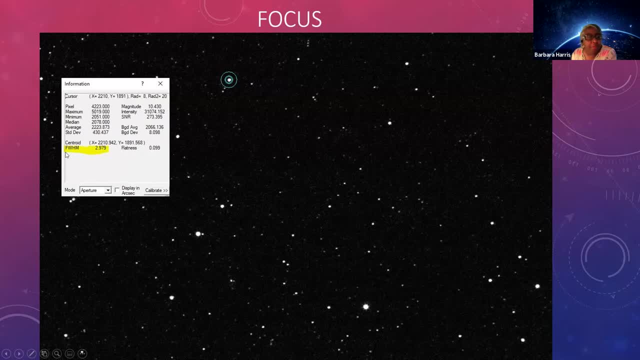 something called the full width at half max, FWHM, And it stands for full width, half maximum, And I'm if matching the measured part to each성이, And what it's doing is that it's measuring how wide the star is at half of its maximum brightness, And this says that it's 2.979 pixels. Now, this is. 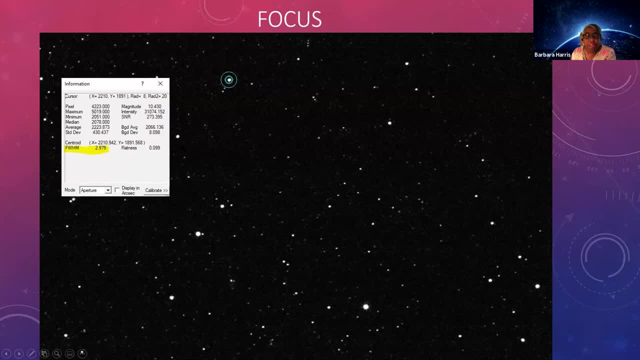 inadequate for photometry. This is under sampling for photometry. for DSLR photometry, We want our star image to have a full width, half max of at least 8 to 10 pixels, So we could put the star Ling and we can put夢 video as a sample here on this screen, which allows us to give a few of these Marin. 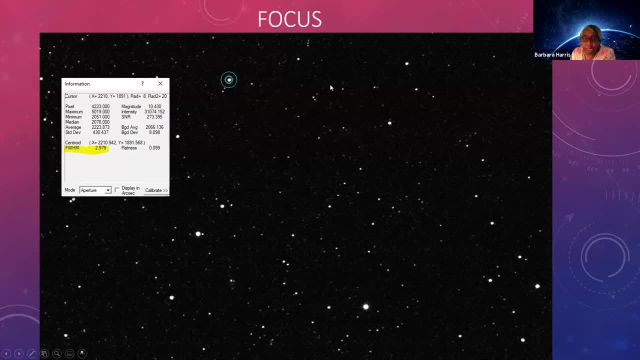 So what I usually do is I go and actually focus as well as I can of my field, just so that one I know that my target and comparison stars are in the field and also get an idea of what the field looks like, Because sometimes when you're defocusing, it's a lot harder to determine. 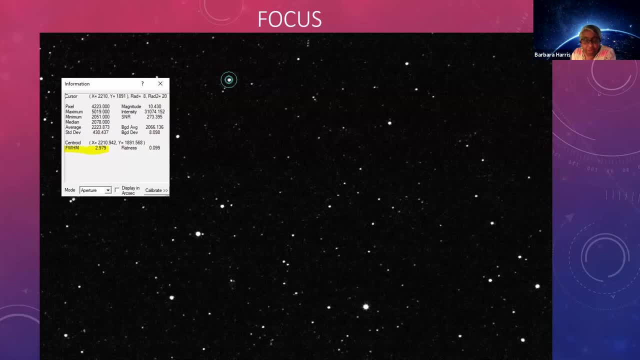 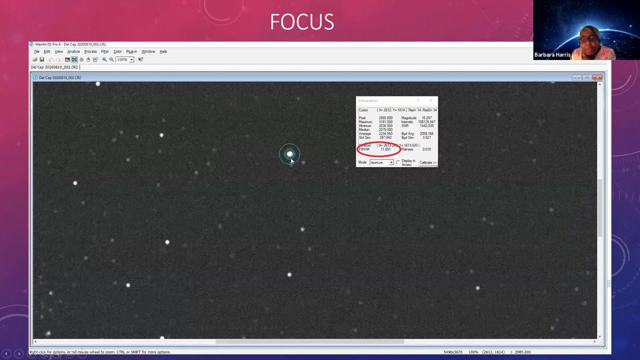 where you, where you're pointing and if you're in the correct place. So I usually take a perfectly focused image first, to make sure I can identify my target and the comparison stars I'm going to use. So this is also an image of delta cpi and this is delta cpi right here. 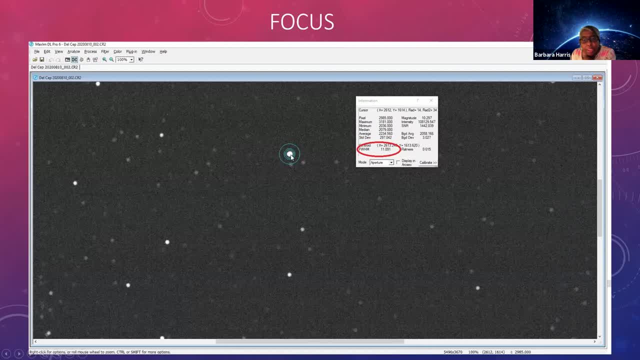 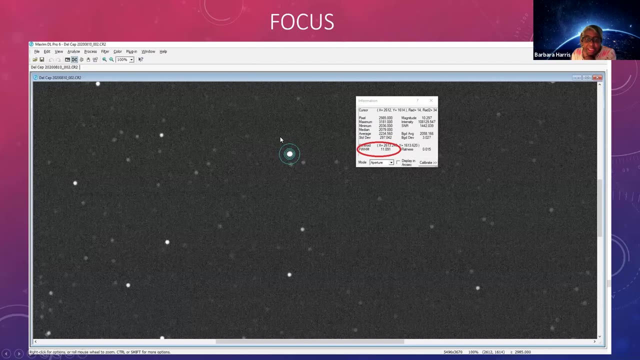 and I have the aperture rings around it and it's measuring the full width, half max of it, and it's 11.091 pixels. So that's perfectly fine for photometry. Like I said, you want about 8 to 10.. You can go higher. you probably don't want to go like. 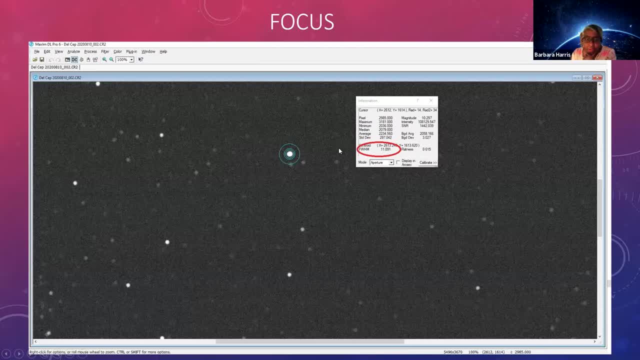 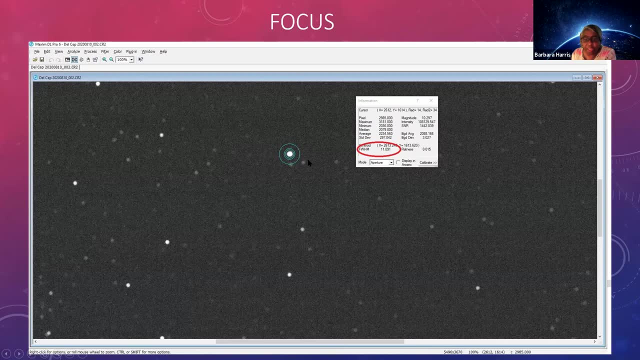 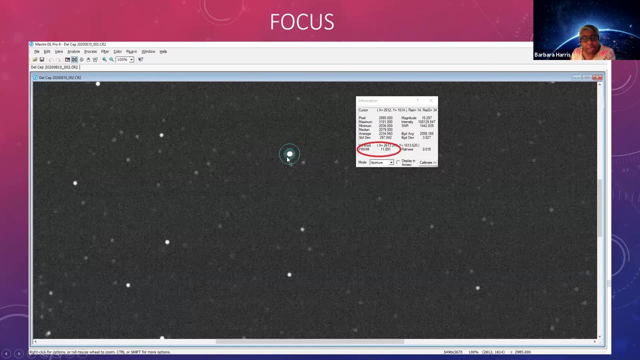 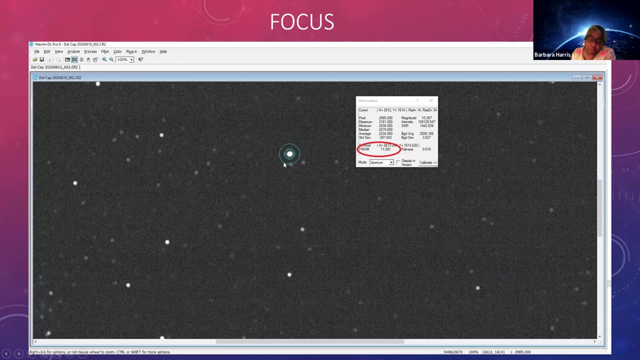 to 30,. you're probably going to lose some accuracy going that high. you don't want it that defocused, But 11 is fine for photometry, So then I have adequate amount of defocus. so I basically take a minimum of about three or four images of my target, and I'll explain why later. 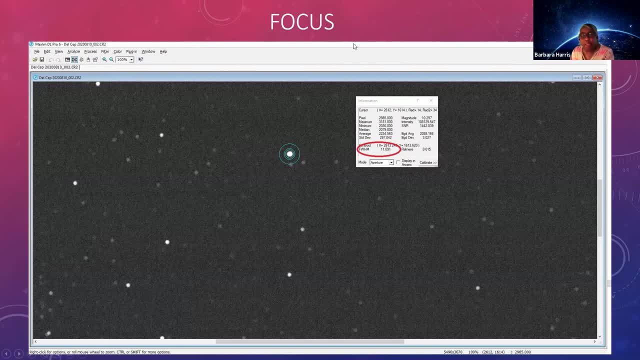 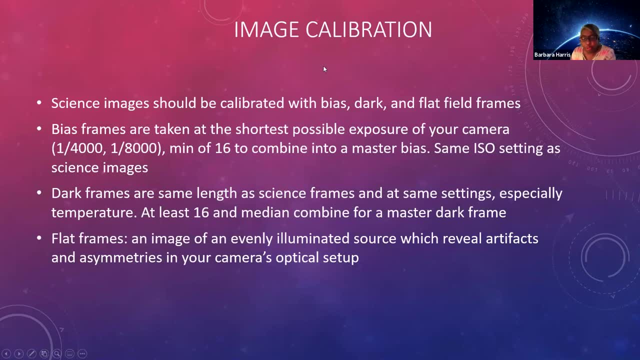 So, once you've captured your image and you like, like I said, I take about three, a minimum of about three or four images of my target And I've made sure that my pixel, that my target star, is spread over at least 8 to 10 pixels. I've made sure that there's a good signal to noise ratio. I've made 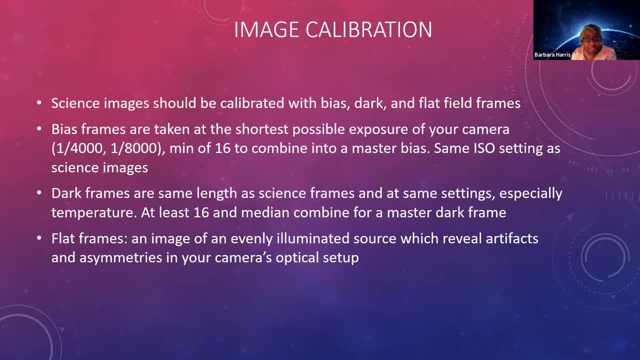 sure that my target isn't saturated, because if your target is saturated, it's worthless. You can't do anything with that. Now, if there's not a good signal to noise ratio, you can go back, and if you have a tracking mount, go for longer exposures, or you could take longer. you could. 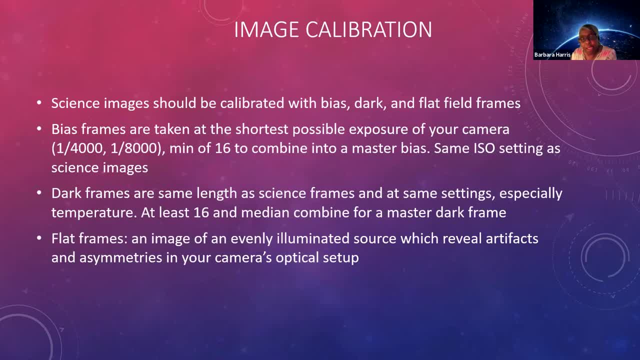 take the same length of images and then you can stack several of them to get a higher signal to noise ratio. So once you've captured your target, you want to, you want to to do your calibration images And unfortunately I don't have a whole lot of time to go into how 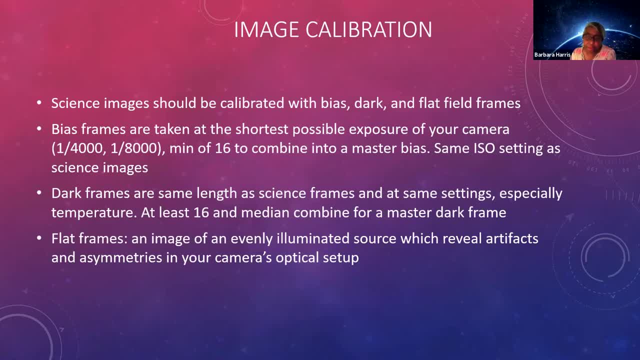 how to do calibration images, But quickly. a bias frame is basically the shortest possible exposure of your camera And most DSLR cameras the shortest exposure is either 1 4000 or 1 8000 of a second, And you want to collect a minimum of about 16 of these and then combine them. 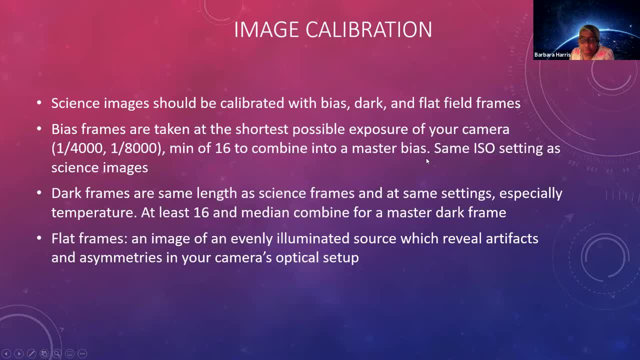 to get a master bias frame. These also should be the same ISO setting as your, your science images. The next calibration image is: you want to capture a dark frame to decrease the noise in the image. Dark frames are taken at the same length as your science frame and at the same settings as far as 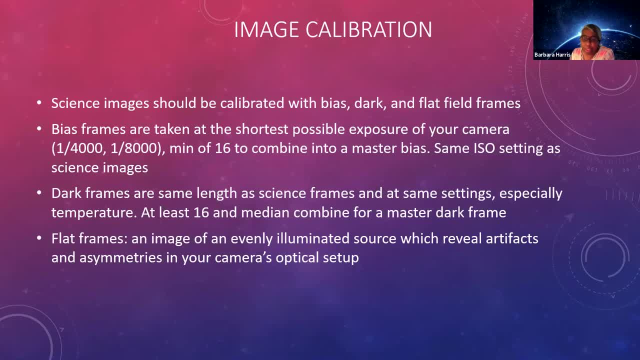 same ISO settings, same f stop. Everything else is the same And especially for DSLR at the same temperature. You want to do at least 16 of those and median combine those for master dark frame. The flat frames are some of the hardest frames for people to to kind of get an understanding. 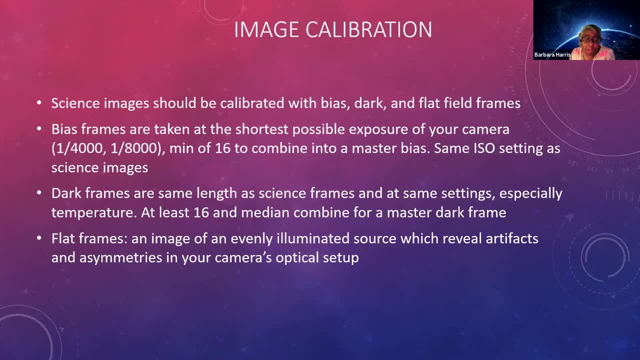 of and and and to do. flat frames basically are edges that take an image of an evenly illuminated source. and and and to do. flat frames basically are edges that take an image of an evenly illuminated source And what it does is that it reveals any artifacts or asymmetries in your camera's optical. 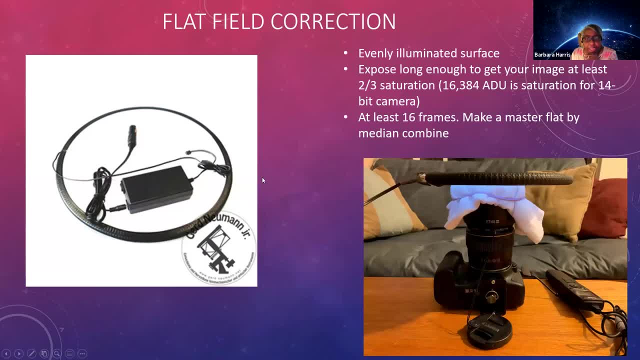 screen. For my DSLR camera I use a Gerd Neumann EL panel. I usually use a cloth over my lens and fold it several times so that in an exposure of about 1.5 to 2 seconds I get about two-thirds of saturation. So I usually shoot for about 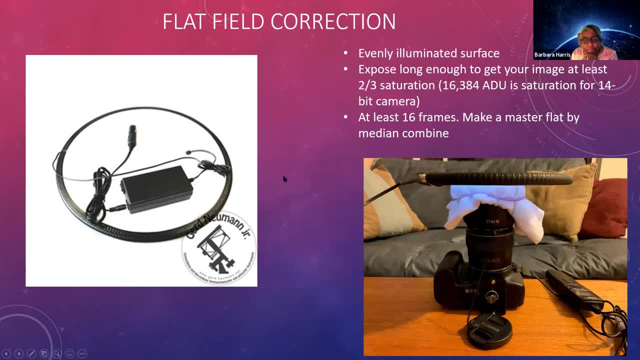 10,000 ADU for my flats and I try to do no more than two seconds for my flats And I usually take about 16 flat frames and combine them to get a master flat. One of the things I don't like about this particular EL panel is that it's just one intensity. 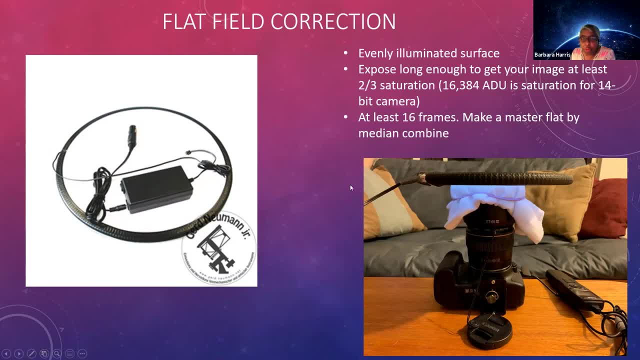 So if it's too bright, the way you're going to decrease the brightness is basically like you can use a t-shirt and fold it over several times over your lens to decrease the brightness. For my large telescope, for CCD, the flat panel that I use for that has adjustable. 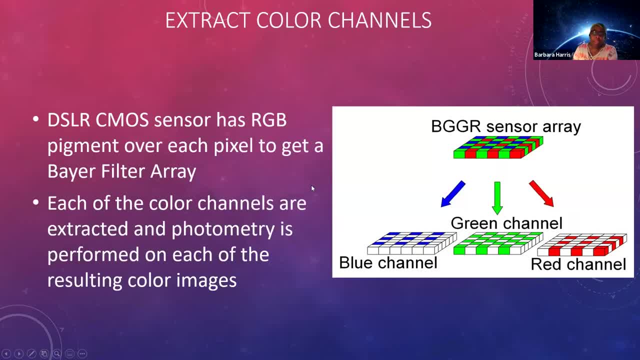 brightness for the flat panel. Now the DSLR CBOF sensor has red, green and blue pigments over them, So you have a monochrome filter, and then you have what's called a Bayer filter array of red, blue and green filters painted over each pixel. 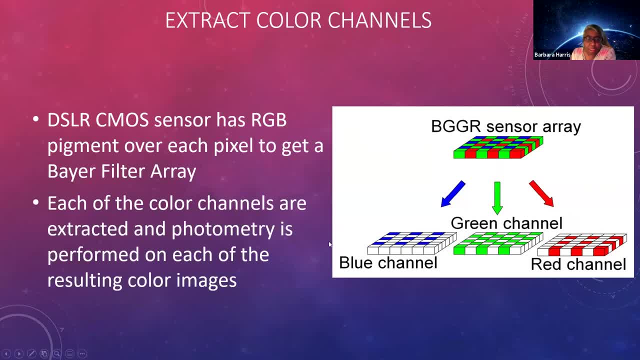 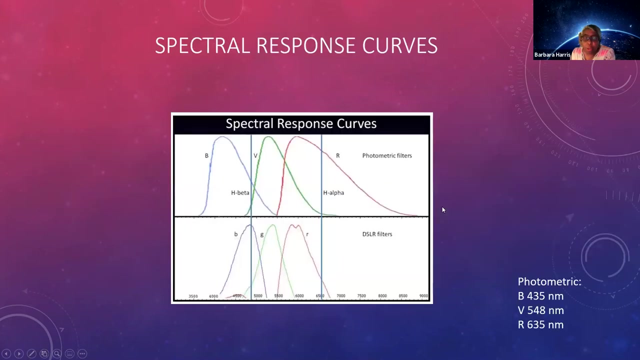 And there are two green pixels for every blue pixel And a Bayer filter array, And when we take an image, what we're doing is the light is hitting each of those filters and each pixel is only going to measure, obtain the light for one color. So what we're going to do is we're going to 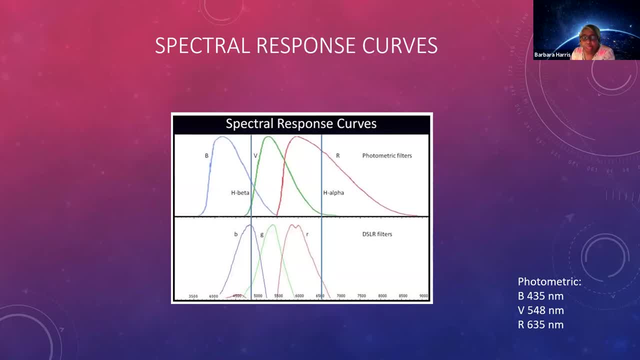 extract those colors to do photometry on them. And when we do photometry- whether it's CCD photometry or DSLR photometry- we're doing it on color filters. We're not just taking a black and white image, We're taking an image through a color filter, And for CCD cameras we use 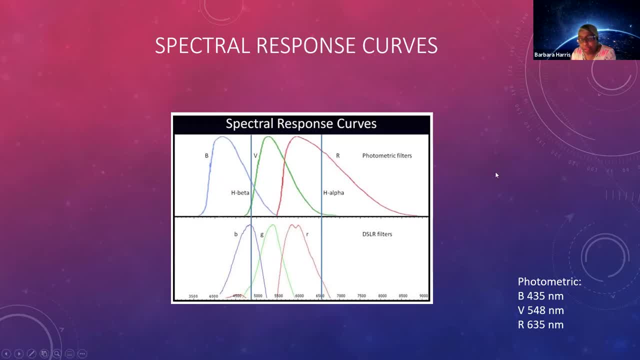 photometric filters, And the most common photometric system is called the Johnson-Cousin photometric system And it basically designates a peak wavelength and a bandwidth for each color filter. So for a beef filter, for the Johnson-Cousin system, it usually peaks at 435 nanometers. For V, which is equivalent to green, it peaks at 548. 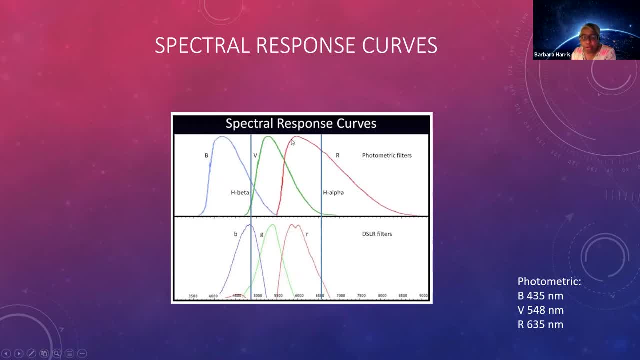 nanometers And red peaks at 635 nanometers And then Johnson-Cousin, it peaks at 635 nanometers. If you look at the spectral response of DSLR filters separated out for each color, the blue doesn't quite line up with the blue of the Johnson-Cousin. 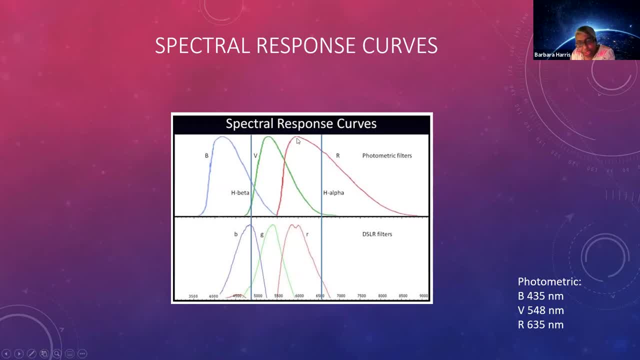 system And the red, the peak is close to the Johnson-Cousin system, but the width is a lot narrower compared to the Cousin's R photometric filter. So what I'm going to do is I'm going to take a look at the blue of the Johnson-Cousin system. 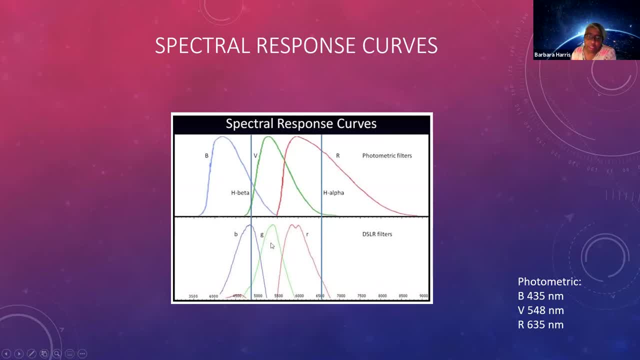 and we're going to take it to the red of the Johnson-Cousin system. And when I do photometry I only work with the green channel of the DSLR Bayer filter because it closely matches the V or green photometric system And this is another comparison of the 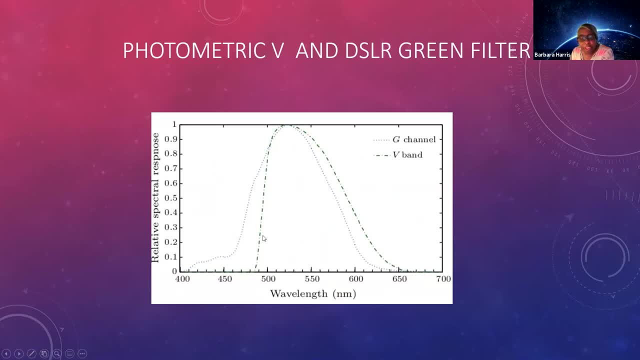 wavelength of the V. the green dotted line, that's the green photometric graph for the Johnson Cousins system, And this blue dotted line is the green channel from a DSLR camera. So the peak is almost pretty much identical. The width of the band: 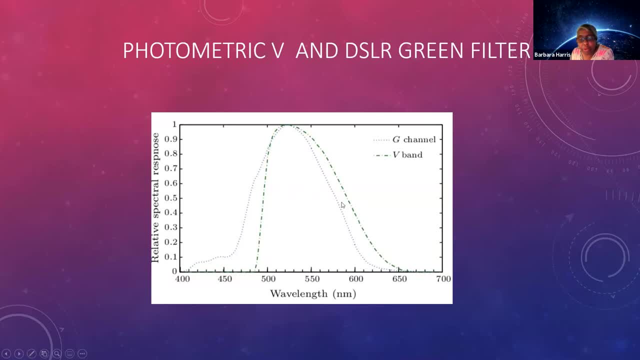 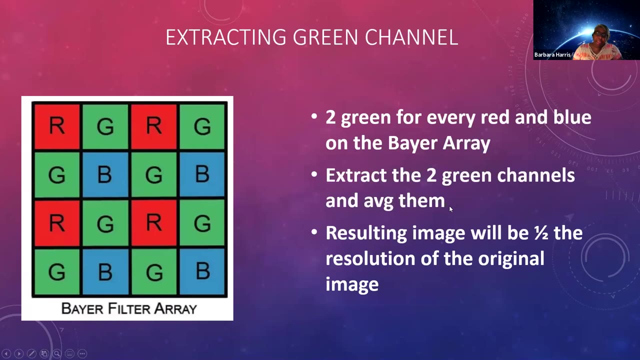 path is a little bit wider, But they're they're pretty close. So I only work with the green channel of the DSLR camera. So, like I said, the Bayer filter array has two greens for every blue and red array And what I do is I have software like in Maxim. you can. 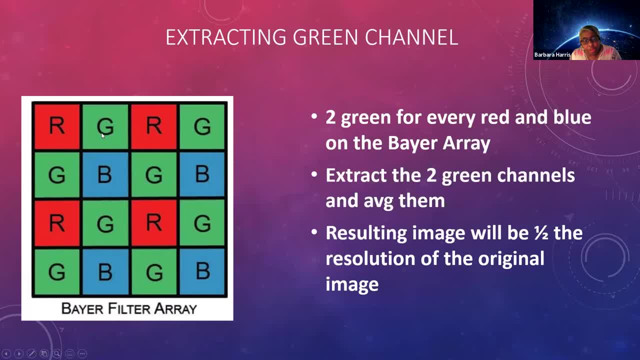 extract the color channels that you're interested in from your raw, your raw camera images. Once you do this, once you subtract either the red, blue or the two greens, the resulting image is going to be half the resolution of the original image. 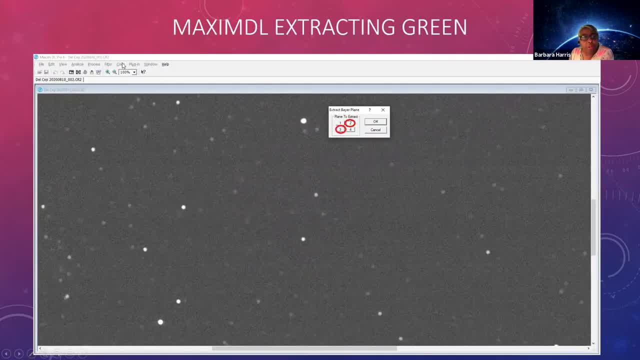 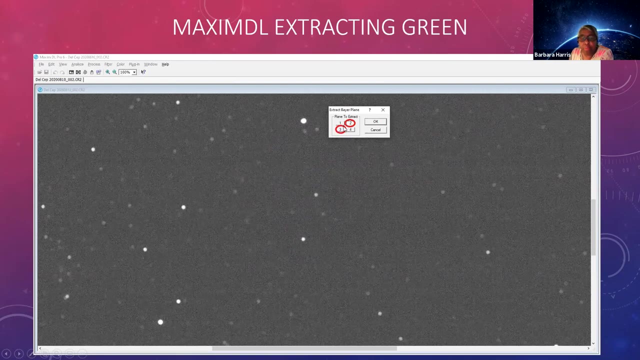 So if you're in Maxim dl, if you go to the, the color menu, you'll go down and you'll find an item that says extract Bayer plane And it is, instead of listing it is red, green, green, blue- it lists the option as one, two, three, four. And that's because every camera 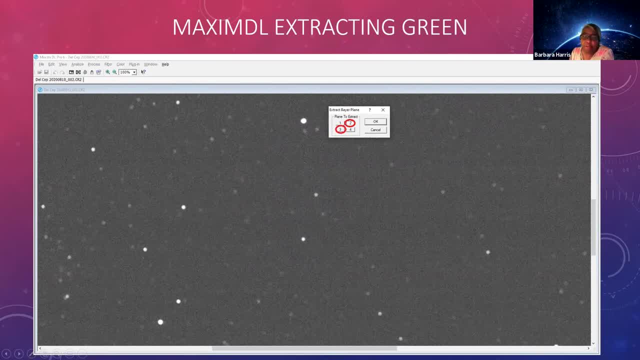 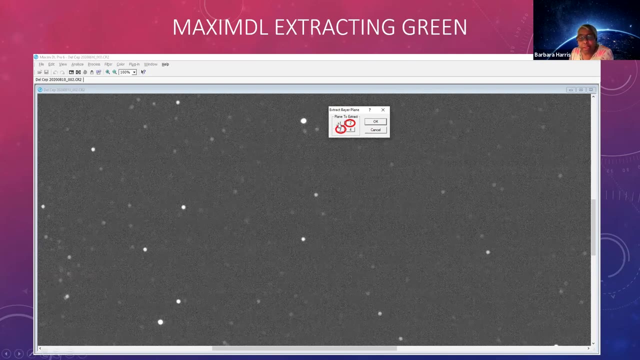 manufacturer has a different order of how their pixels are organized. So for my Canon 40D and Canon 70D the Bayer array is: number one is red, number two is green, number three is green and number four is blue. So you have to know what the Bayer array pattern is for your camera. 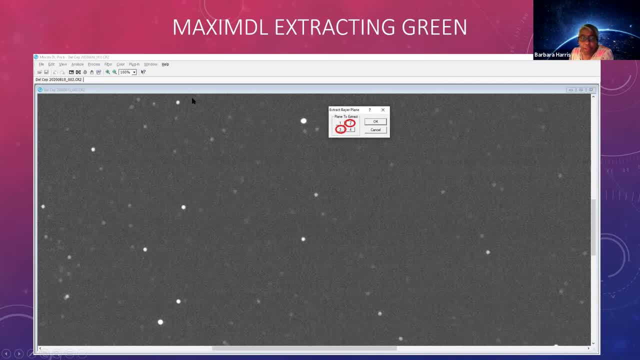 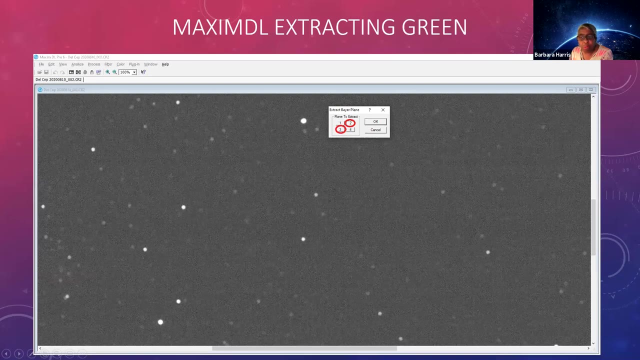 to know which ones to extract. So for me, I have a raw image here and I'm extracting number two and number three, which are the green, And what I do is I subtract those two channels from one image and I average them together to. 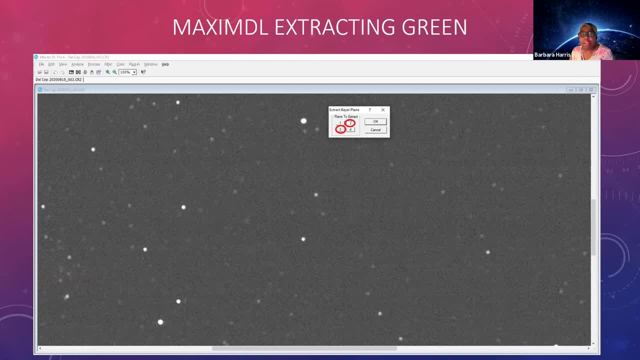 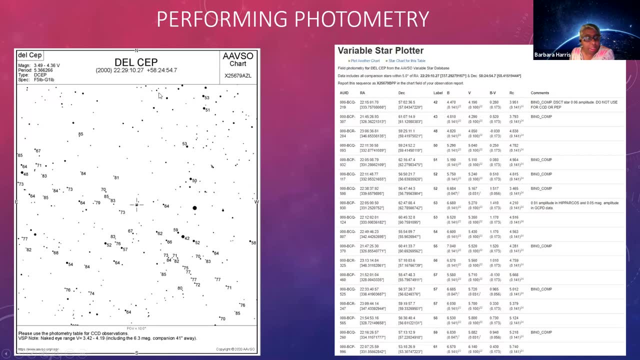 come up with one green image And that's the image I do photometry on. Once you know what your target is, you can download your chart and photometry for that particular chart from the AAVSO website. For my 85 millimeter camera lens, it gives me about a 10 by 15 degree field of view. 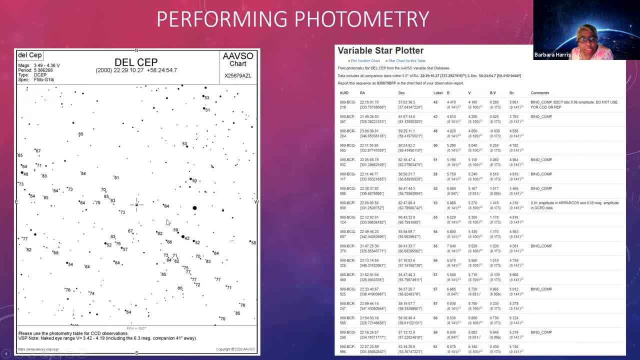 So I usually download a field of view of 10 degrees and I limit it to like in this particular chart it's limited to probably 8.5 magnitude. You don't want too many stars When you're trying to create a chart, because one the website, it'll crash before it gives you an. 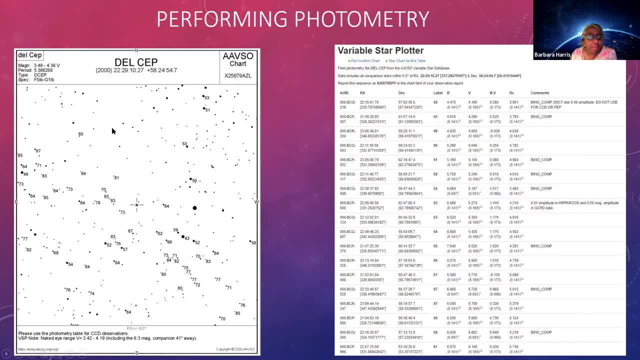 image And also your image isn't going to contain stars any brighter than that anyway. So this is a field of Delta CFI, that's a 10 degree field of view. Here's Delta CFI, in the middle here, And then it lists magnitudes all around it so that you can, you can see the image And then you can. 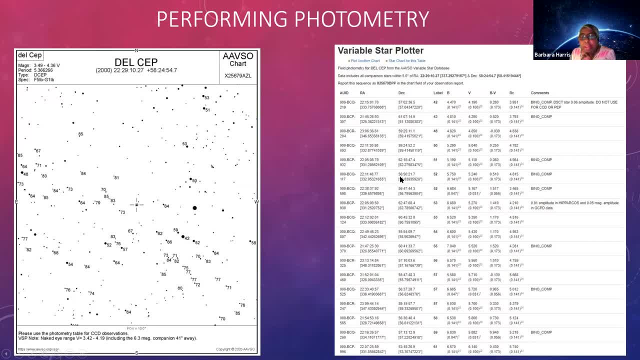 find the keeper. You can see the video too, Surprise, So that you can use for comparison stars. Then here's the photometry For those, uh, comparison stars. Uh, that that you're gonna get with this chart. It tells you exactly what the magnitudes are like. There's 53 star right here. 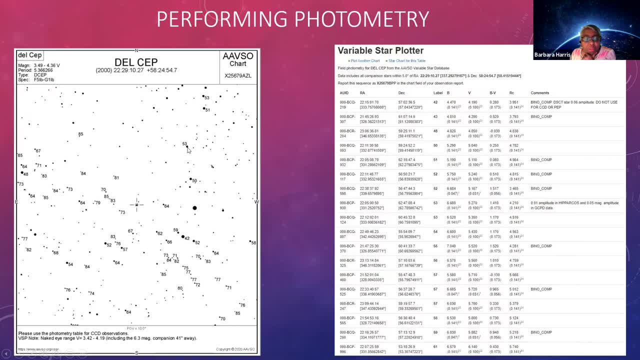 That means that it's 5.3 magnitude star right here And if you want to use that as a comparison star, you go over here and find 50.3 points, which may be an much smaller ending in portion. 高 company. right here And when you're looking at honest person does veryoger results, but sometimes it's between 50 and 53. tickets. So now this interlock or a double-g leaning feature and the camera doesn't take advantage of your camera. 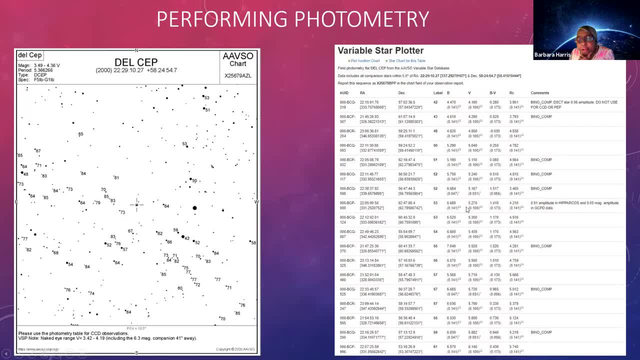 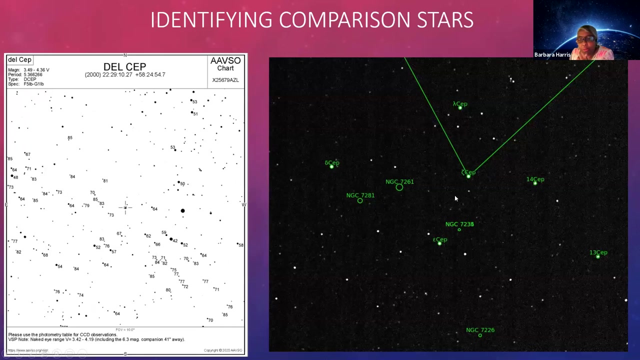 563 label here and for V filter the true magnitude is 5.270.. So these you can download from the AAVSO website, depending on, and you can tell what field of view you're interested in. Sometimes I have an image and sometimes I can't figure out why the variable that I'm 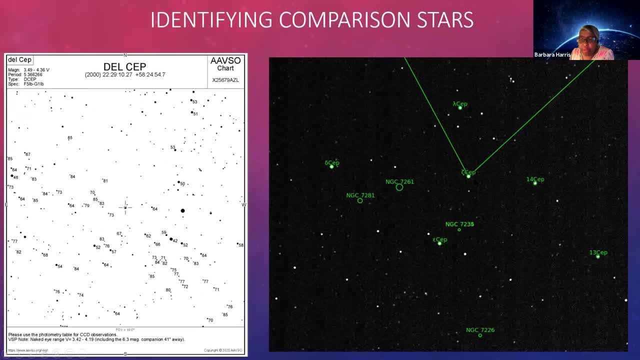 interested in is in there in the image. and if I can't figure out what I'm looking at, I upload my image to astrometrynet and it gives me a label of what stars are in the image And it tells me that delta CCI, right here, is in the image. 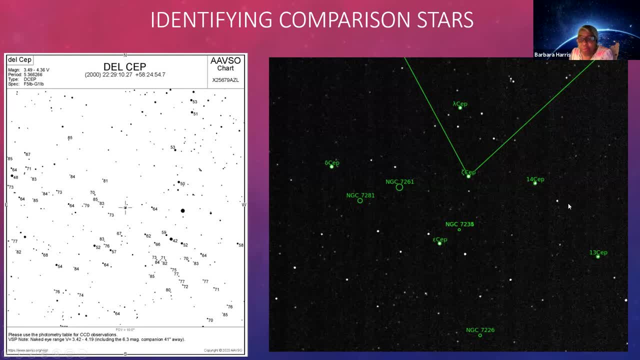 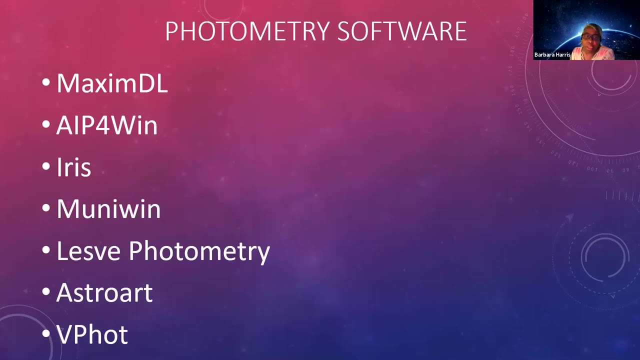 And so it kind of tells me that, yes, my variable is there and other stars that I'm interested in is in the field of view. So some of the software that you can use can be a problem for DSLR photometry, because some software like 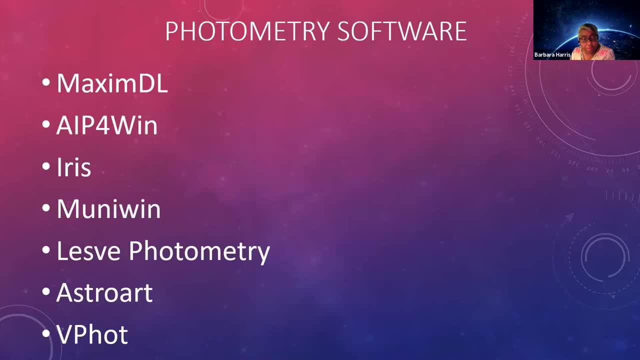 my template, my our own software on the AAVSO website. You can't subtract the color channels from the raw image, So you have to have software that you can extract the color channels first. Once you do that, you can use V Notes software. 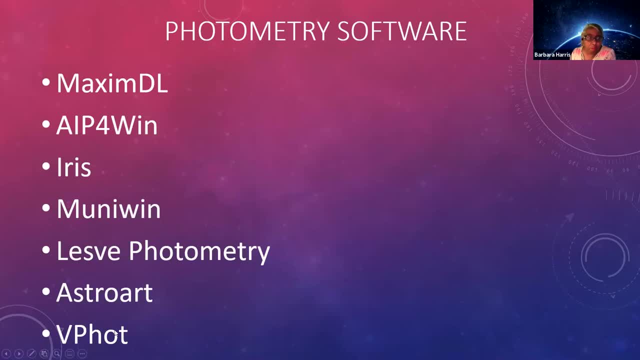 Other software from the WRSSR collective is: text ergases: I use some. Jacksonук has data and chalkboard. I use maxim DLL. Jackson trucs are very distractive on campus that people aren't able to get right now. 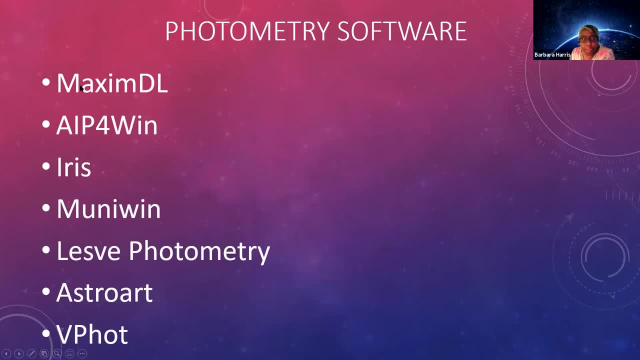 DL, fortunately, can do everything. I calibrate my images from Maxim, I extract the color channels, I perform photometry in Maxim, And when you perform photometry it creates a file of your photometry that you can then submit to AAVSO. AIP4Win also is software that you can pretty 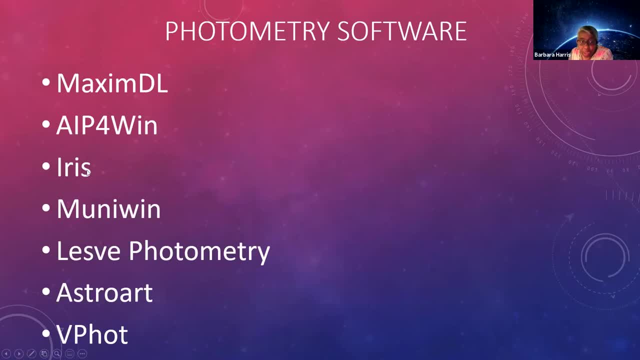 much do. everything in IRIS is good. IRIS is free, So that's a big plus. IRIS has kind of a steep learning curve, but it's very good and you can do everything. MuniWin is another photometry software. Let's see, photometry is also good And it's free. but the problem: 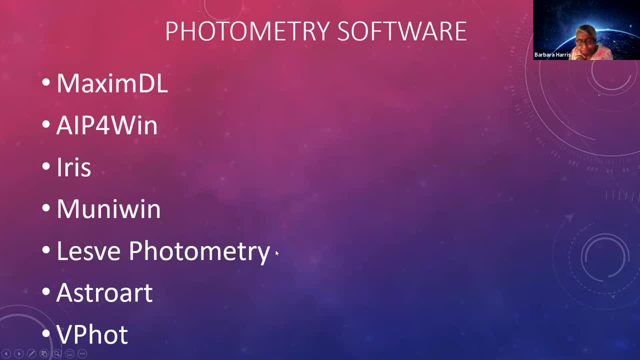 is that you also have to have Pinpoint Astrometry, which I think is about $150.. So if you have that software then you can use Let's V Photometry to do your photometry AstroArt also. you can do everything in And 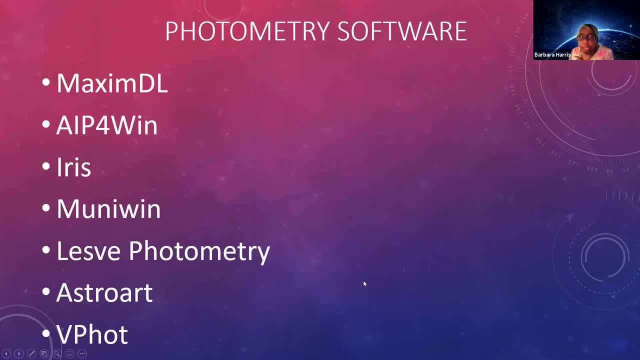 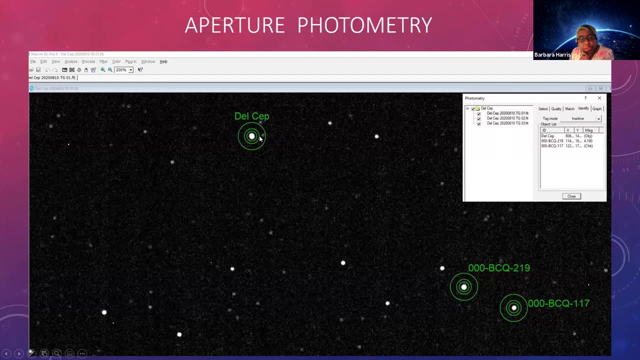 like I said, our own VFoat. you can do your photometry there. as long as you extract your color channels before you get to VFoat, Okay, And you can also use VFoat to do your photometry. So, like I said, I use Maxim for my photometry. 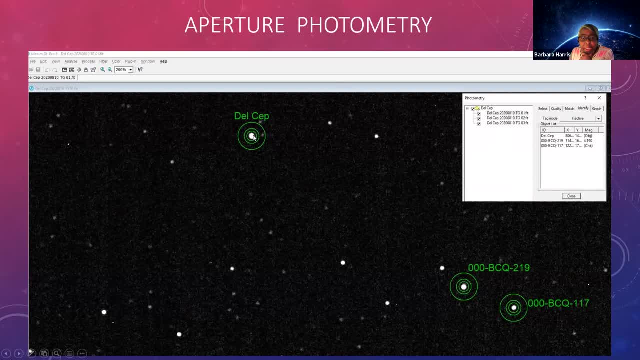 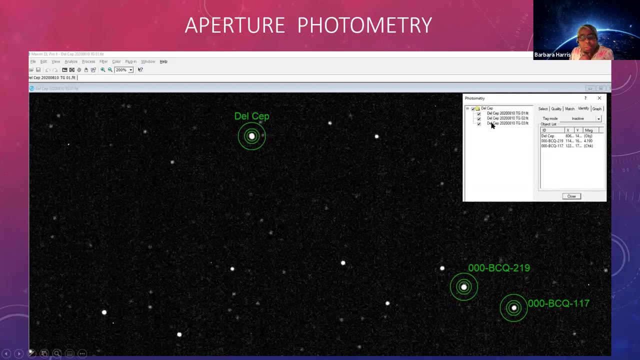 You're basically telling Maxim that this is my target- Delta CPI- and these are two comparison stars- One is a comparison star and one is a check star- that I'm going to use. I have three images that I'm working on, So Maxim is going to identify the image that you're. 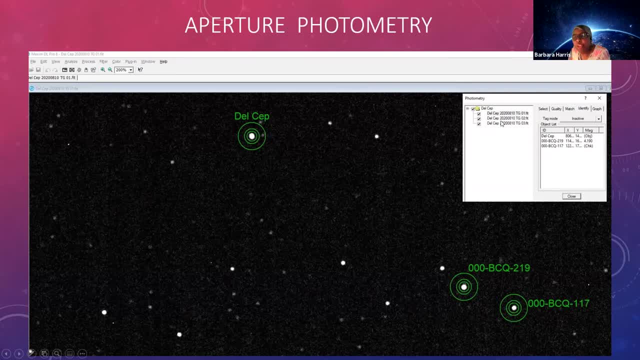 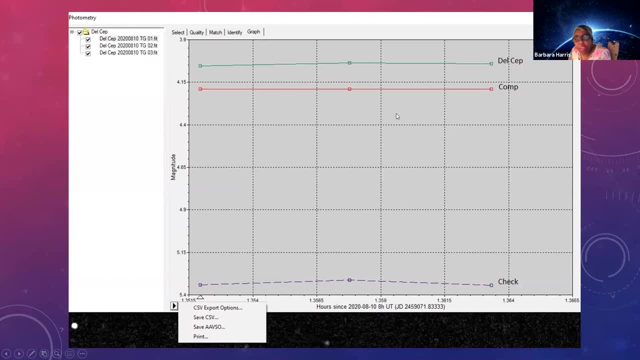 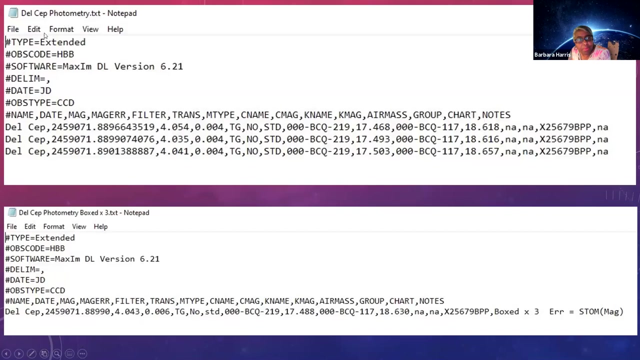 going to see. I'm going to use the comparison and the variable in each of those three images And then it basically gives me the magnitude of Delta, CPI and my comp and my check star, And then I save the photometry as an AAVSO file And it looks like this: So this is an 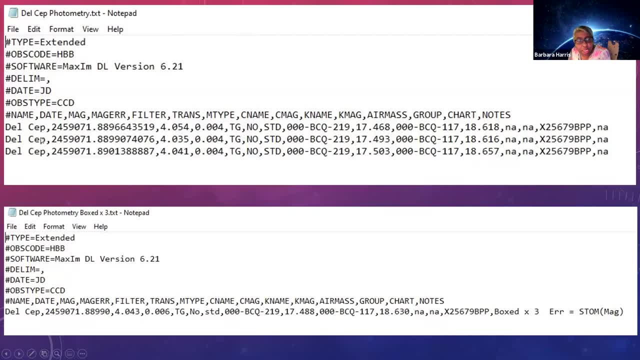 extended format file for photometry. Okay, It gives me three different magnitude readings for the three different images I had for Delta CFI, and so these are the three magnitudes: 4.054,, 4.035, and 4.041, and the reason I do. 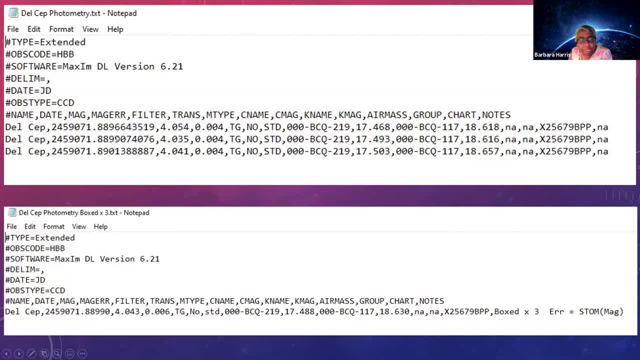 multiple images. is that for a star like Delta CFI, where it's not going to very much on like a 10 or 15 minute time that I collect my images? I basically average these three magnitudes together to get this one final magnitude of 4.043, and I use the standard deviation of these. 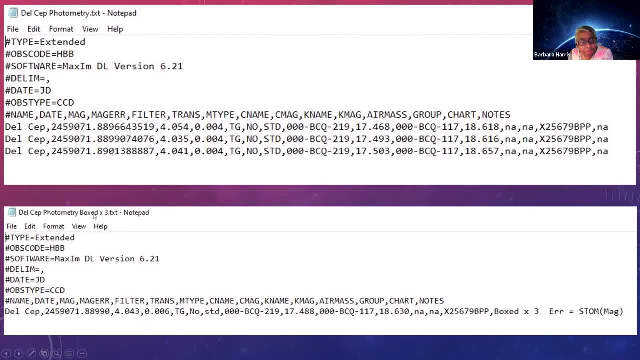 magnitudes as my error, and so this is what I submit to AAVSO. this that's measuring just one image, or an average of three images of Delta CFI. It also averages the time of the three times, and so this is the file that I submit to AAVSO, and if you go on AAVSO website, 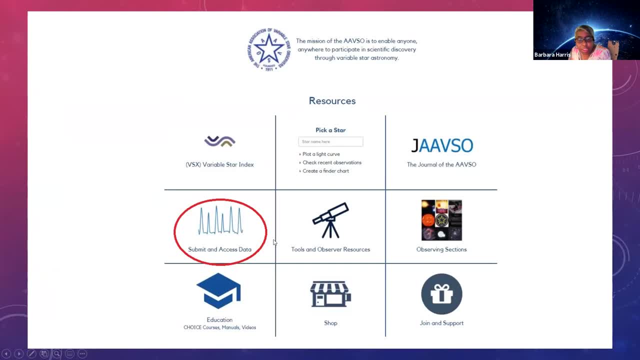 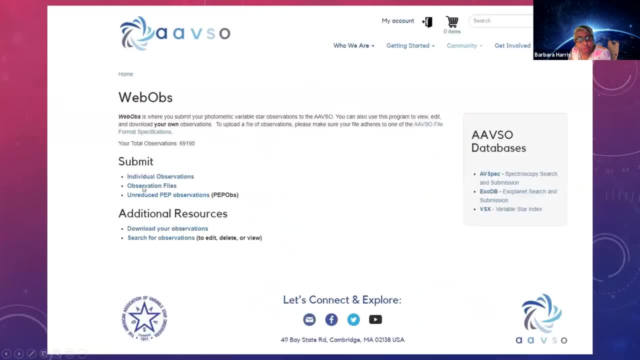 the new website. on the front page you just click on submit and access data, upload photometry, and you're going to select observation files and you select observation files and then you find that file on your computer and submit it. One thing that I want to mention is that 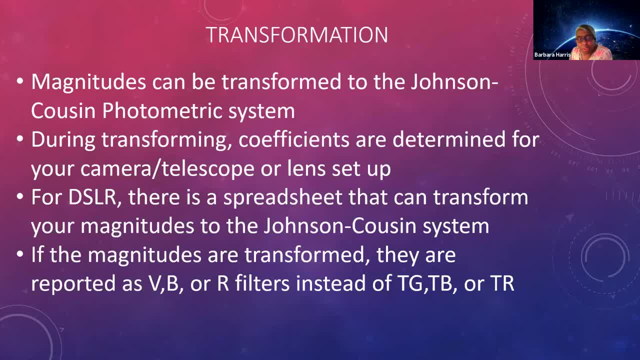 when you submit your results, you're going to submit them not as a V filter, but as TG, which means tricolor green. There is something called transformation, where you transform your tricolor magnitudes, your tricolor green, your tricolor blue. 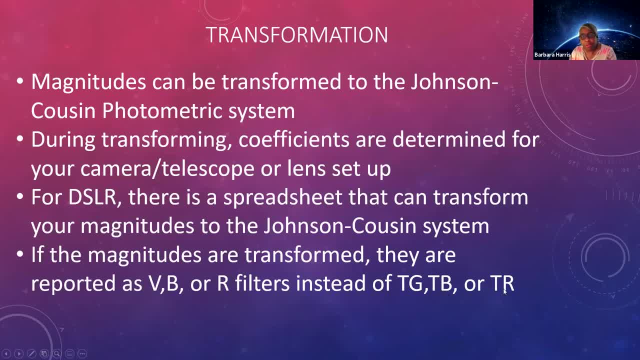 or your tricolor red magnitudes into. you're transforming it to the Johnson-Cousins photometric system. This takes a lot more work. It can be done by imaging a field like M67 that has standard stars or there's a list of standard. 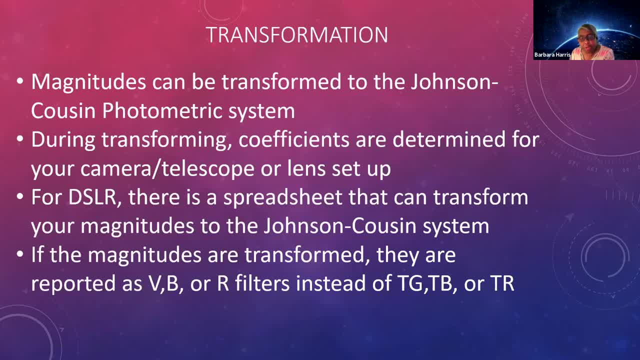 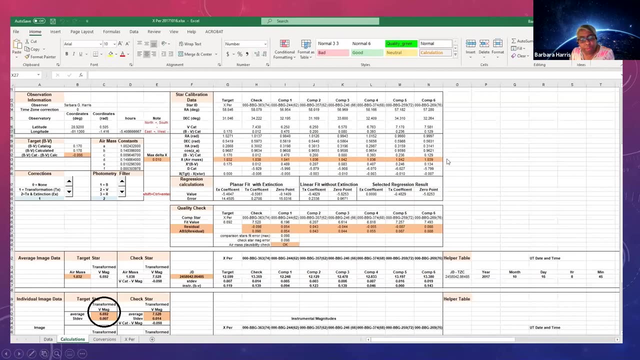 uh stars in the sky that you can image and calculate the transformation coefficients for your system For DSLR. also, there's a spreadsheet that you can do, that you can use to transform your images to the Johnson-Cousins photometric system and if you're going to do that, you're going to need at. 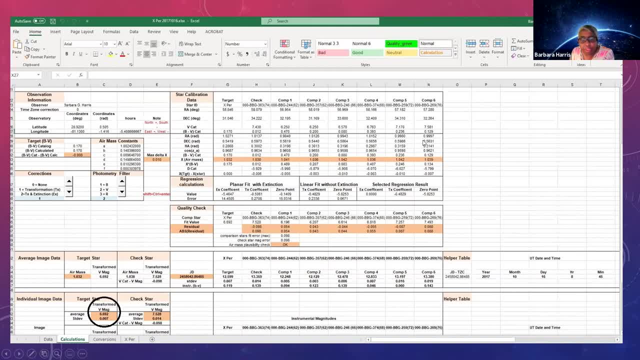 least about seven pump stars. um, uh, uh, uh uh, to be able to transform your, um, your tricolor- green or blue or red images- into a photometric red, green or blue image. So it can be done, but it takes a lot more work. 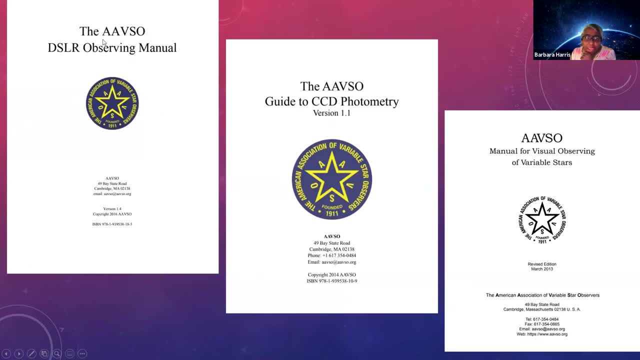 Uh. so, like I said, AAVSO DSLR observing manual is on the website. Everything I've talked about can be found in this, this manual, And what I would also say is I would also recommend is uh, uh. 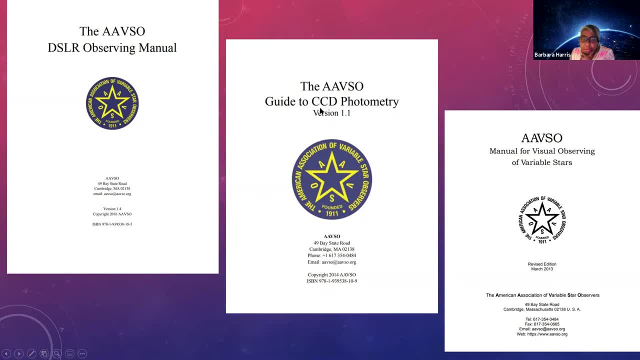 uh, if, if, if you're, especially if you're new, to also download and and read through the CCD photometry uh manual, because there are um some things here that also translate easily to DSLR um. 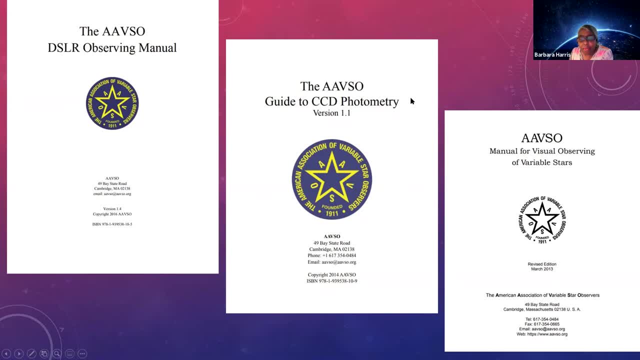 especially uh calibration files, uh, but a lot of other things. So I would also recommend getting uh this manual And if you're new to variable star observing, also uh read through the manual for visual observing of variable stars. 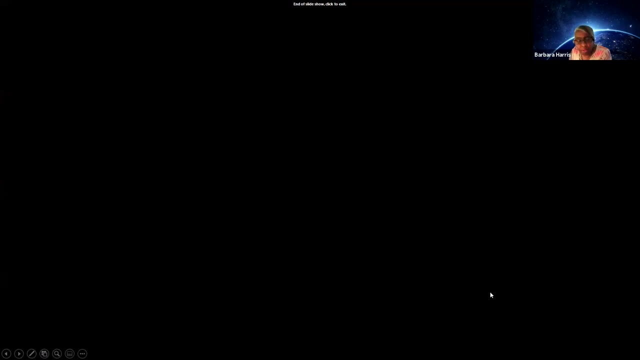 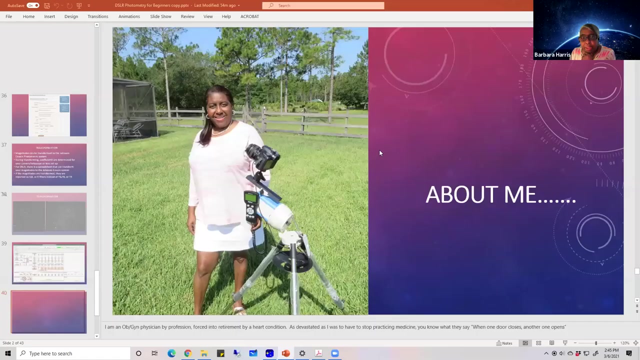 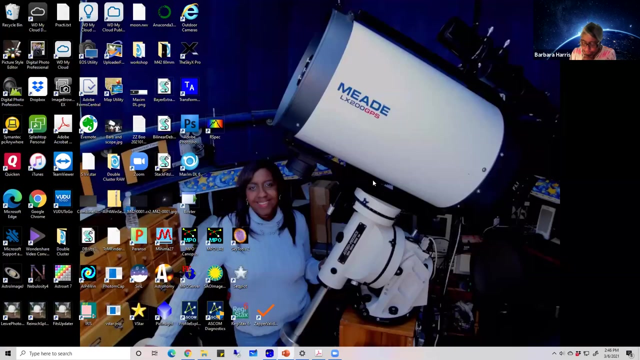 uh, that could be helpful also. So I know this was a lot, uh, but, like I said, everything can be done through. uh, everything I've mentioned can be found in that DSLR manual And, um, if you still are having problems, 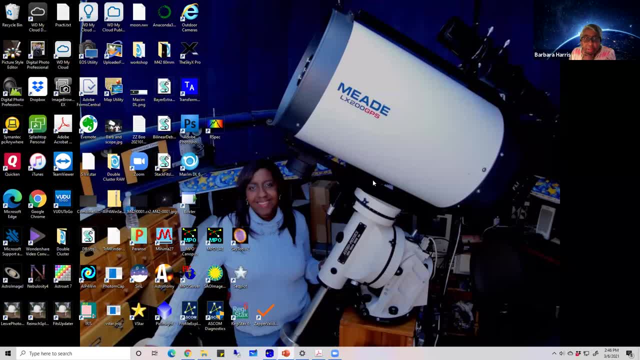 there are mentors uh on uh in the AAVSO, including myself. uh that uh will help you, So let's have questions. Thank you, Dr Harris. All right, Uh, yes, let's get to the questions. 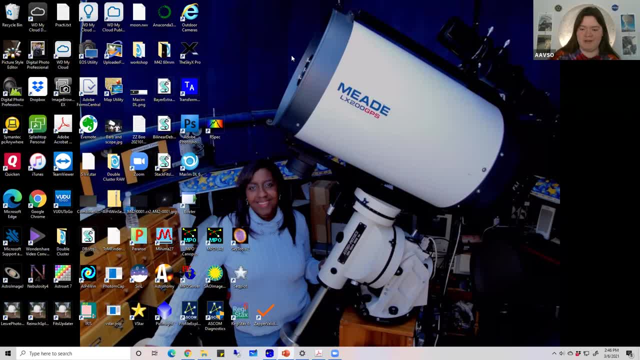 Now I saw that there was a common thread between quite a few of these questions coming in, So let's address that one first. We had a lot of people asking about how does it affect photometry if you're using, uh, a modified DSLR? 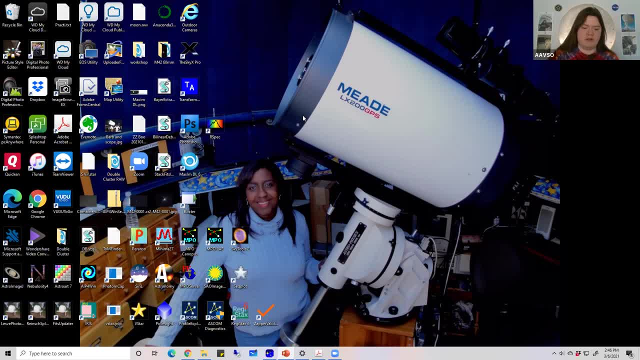 whether uh completely clear of filters or uh with a modified infrared filter that passes a little bit more hydrogen. Well, you can still do photometry uh, but, like I said, I usually will only do uh the green channel. 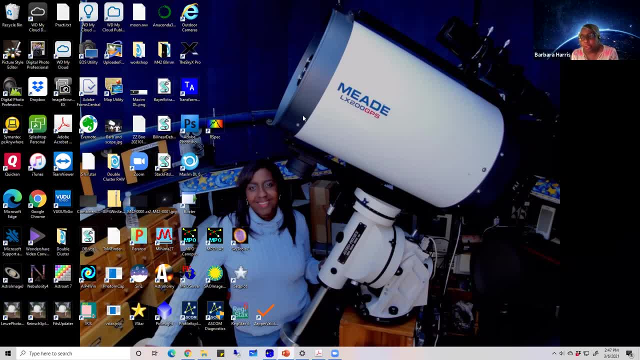 uh for my photometry. So, uh, modern, you can still uh extract your green images out of your modified camera If you're. if you want to do photometry of the the uh red and blue. 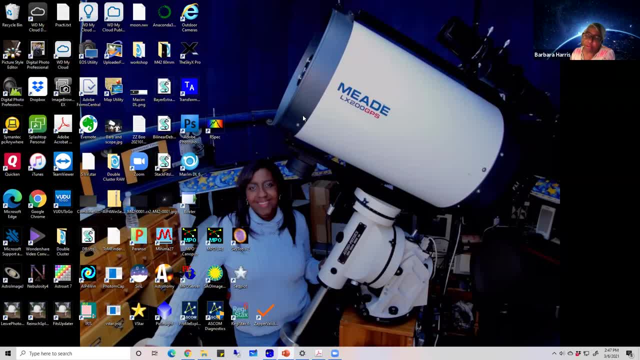 uh, I usually recommend transforming those if if you're going to to uh submit red and blue data, but there's no reason why you can't uh extract the green channel from that camera, from those images, and do photometry on that. 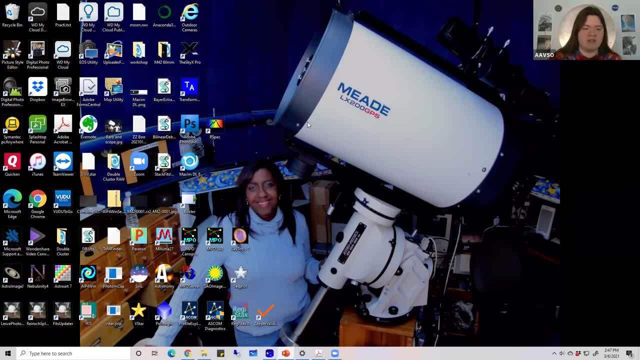 Thank you. Uh, we have a question here from Brad Vici who asks: can the Bayer mask pattern be deduced from an image? I'm not sure I understand. uh, presumably, if you don't know, the Bayer mask pattern of 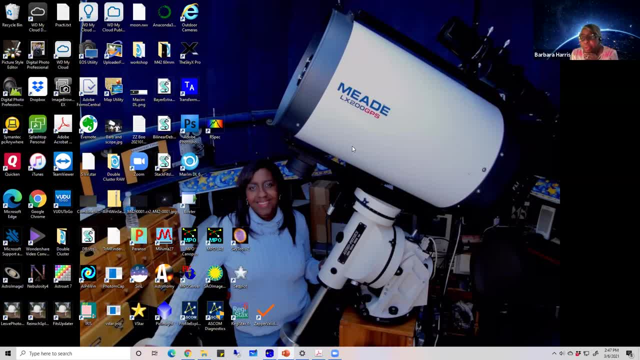 oh sure, Uh, yeah, it's, it's easy. Just just take it uh a regular uh image, Um and um, depending on your software, uh like, like I have pics inside. 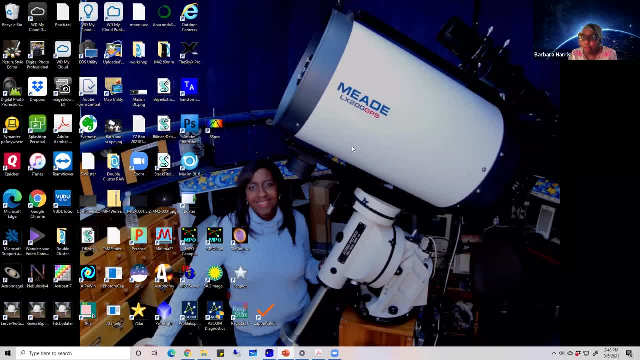 um, um and, and especially for if I'm doing a long light curve, I like to do some of my preliminary work- and picks this side where I extract the color channel And um. one thing I didn't mention is that 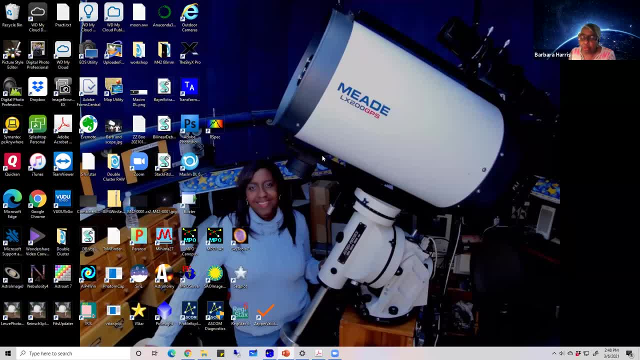 um, what's recommended in the manual is to extract the color channels before you did Bayer, So you're you're not really debayering- You extract the- uh, the colors from the raw image and then you're doing photometry on that in AIP for windows. 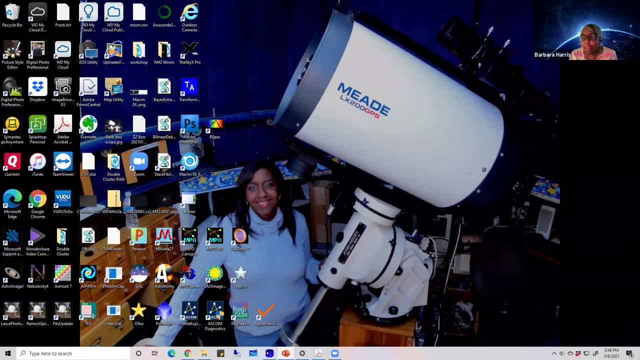 Um, that program it actually does, uh, a bilinear interpolation, meaning that it it debayers the um the image, and then it takes out the color channel, It it takes out the, the green or red or blue. 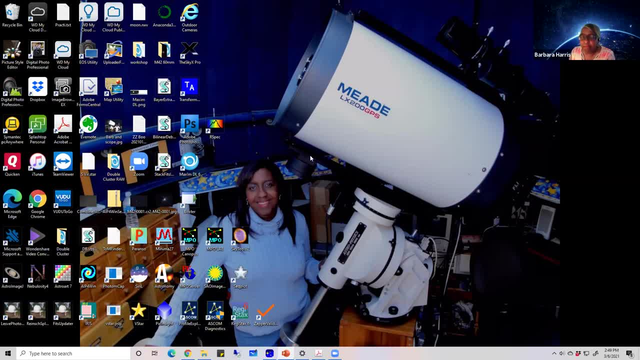 Channel. And actually I like that best. And I've started doing that because if you do an interpolation or D mosaic, the image first and then, um, you separate out the color channels, the image is going to be the same resolution as your original raw image. 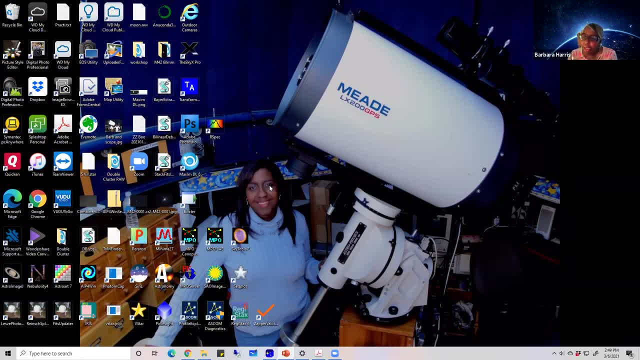 And that can be significant because if you're using a lens um, the star images can be very, very tiny And if you extract the color channel and the, you're taking out an image that's half the resolution of that original. 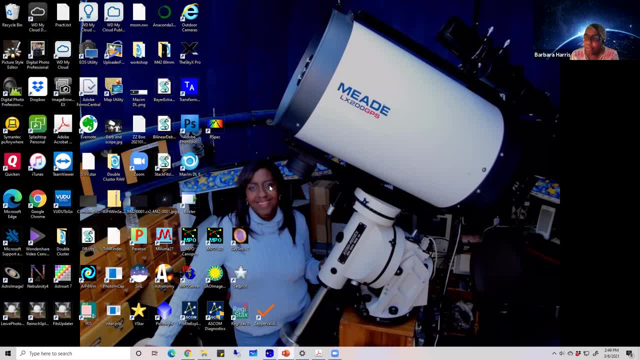 then the stars are even tinier. So I like using a bilinear interpolation And, according to the manual, if you're going to debayer your your raw image, um, the, the. there are several algorithms for D mosaic in their deep bearing. 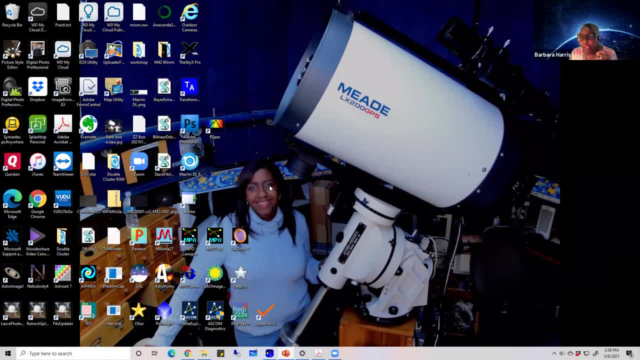 Uh, they recommend only the bilinear for photometry. Uh, so you could figure out what Bayer pattern by just taking the regular color image of something outside or some person And then, um, like opening it and pick in pixel in a picture site and selecting the different. 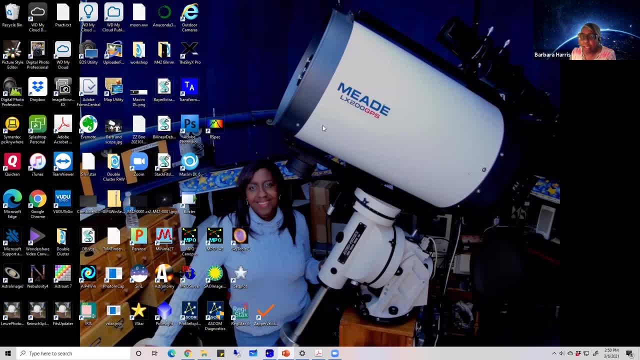 uh, um, uh Bayer patterns, and see which one gives you the correct color rendition. So it, and there's not a whole lot of combinations of what the pattern can be. Um, so it's easy to do: just take a regular image of something and 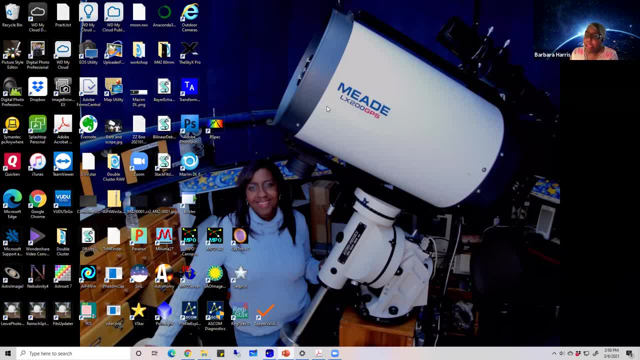 and put it in your software and debayer it and see what gives you the uh, the, the best rendition, And that's going to be your, your Bayer pattern. All right, Thank you. Um, so we had in here several different questions about software. while we're on the topic, 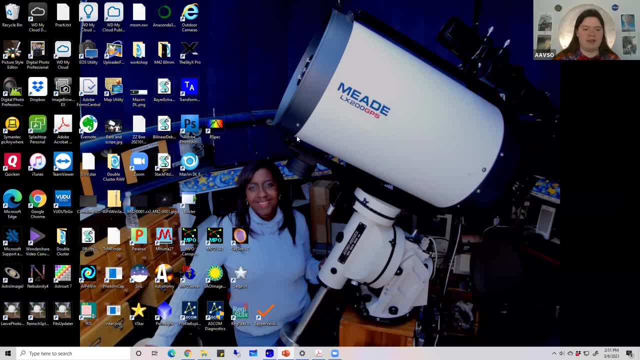 Uh, one was from Blake Nancarrow who asked: can uh Canon digital photo professional do color channel extraction? No, Uh, cause I, yeah, I have, I have that. Um, I don't think so Uh. 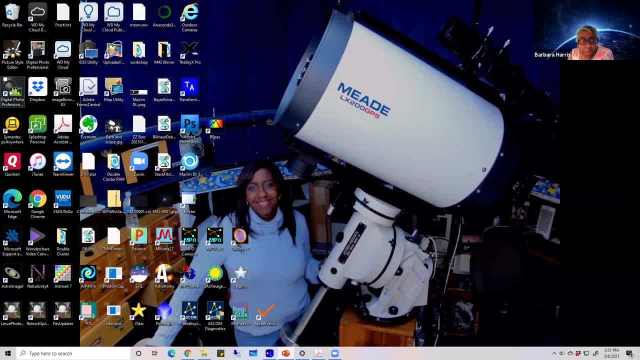 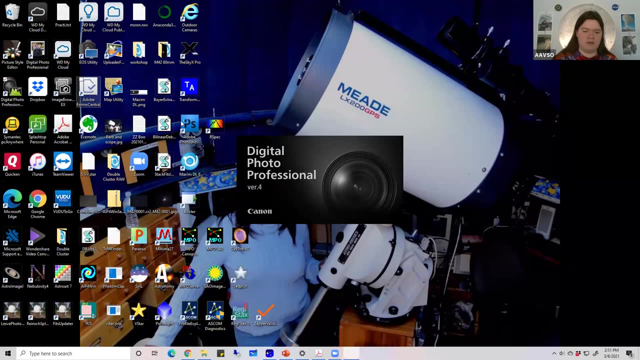 it. it will do, it'll convert it to color, but, um, it can extract the separate color channels. Uh, it can't separate out the three uh color channels. All right, Thank you. Um, we have a question here from Jose Bosch, who asks: 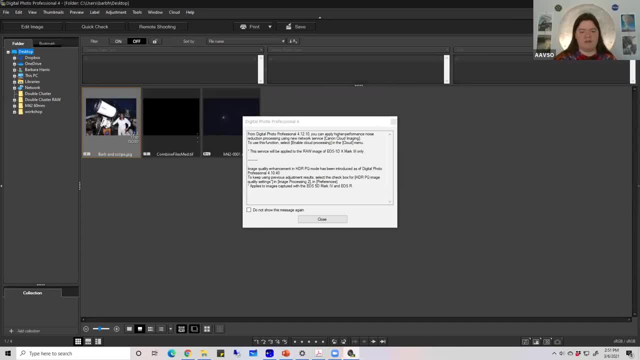 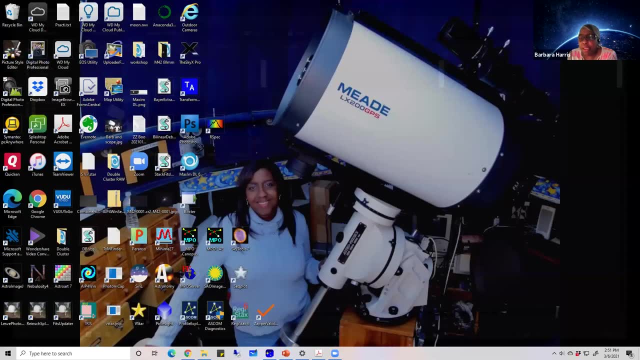 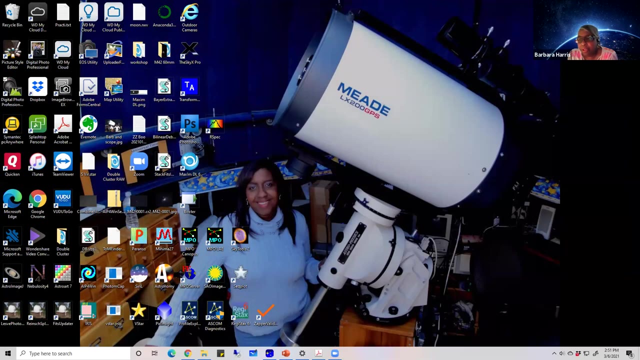 what is the maximum air mass that you recommend for doing good photometry? Oh, I can't convert it to air mass, but I try to stay about an altitude of 30 degrees above the horizon. going, going below that, You, you. 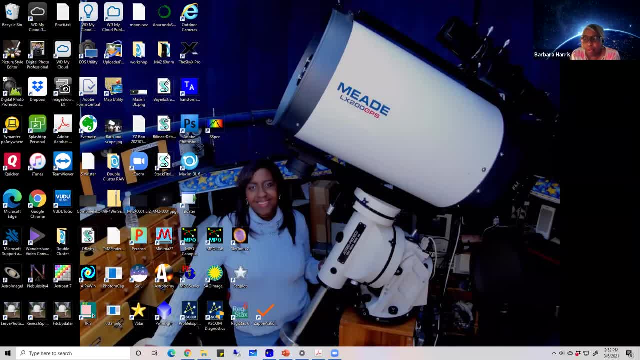 you really start to, uh, to introduce error in your, in your photometry. So, um, I stay above 30 degrees I I I'll have to calculate what that is than air mass, but basically an altitude of 30 degrees. 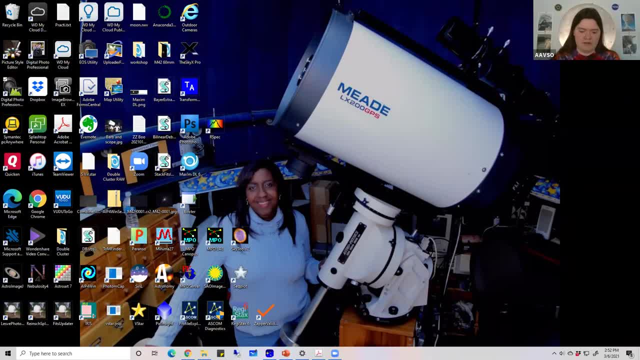 Okay, Thank you, Good answer. Um, we had several different questions here that were all relating to exposure, So I'm going to go ahead and read those out. uh, in order, We have a question here from Gary Shaw, who would like to know what percentage of full well depth would you recommend? 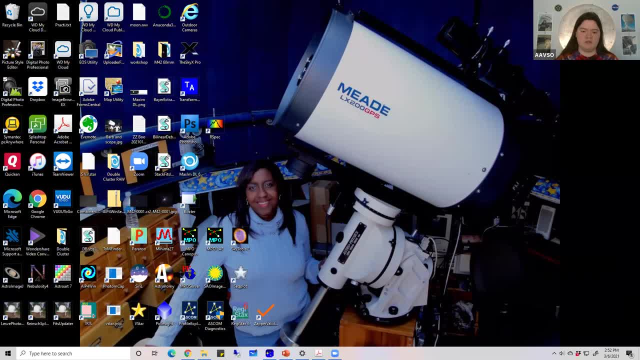 Trying to achieve. when you're setting your exposure, Um your one, your software should be able to measure signal to noise ratio, Um. so what I do is I? I take an image of my star field and I put it on the computer and I want. 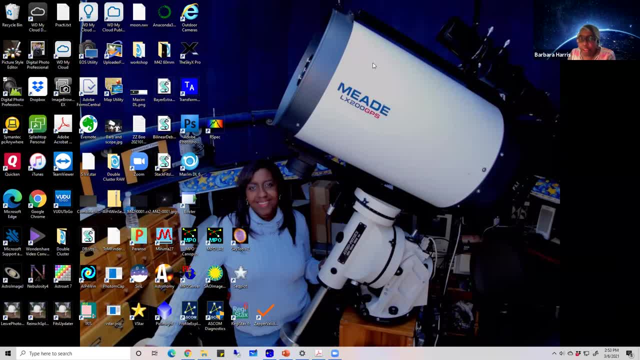 I make sure that my target and pump stars are there, but your software should be able to measure the signal to noise ratio of of the stars in your image. So if you put your cursor over a particular star, um, you should be able to measure the signal to noise ratio. 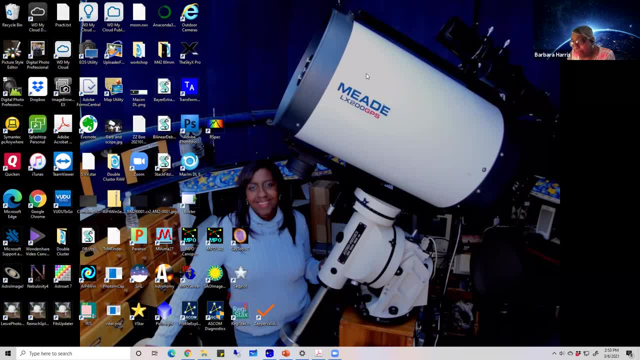 You want. ideally, you want a signal to noise ratio of about a hundred is what I usually shoot for. anything over That is even better, as long as it doesn't reach saturation. Um, I usually try to stay, uh uh, about a thousand or so below saturation, just to be safe. 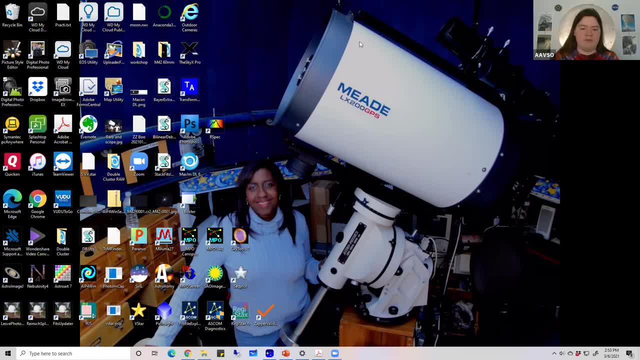 Thank you. Speaking of saturation, uh, the next question is from Gregory Wandless, who has asked: how do you determine if your star is saturated? Uh, like I said, for all those software packages I I mentioned, they should be able to measure the amount of. 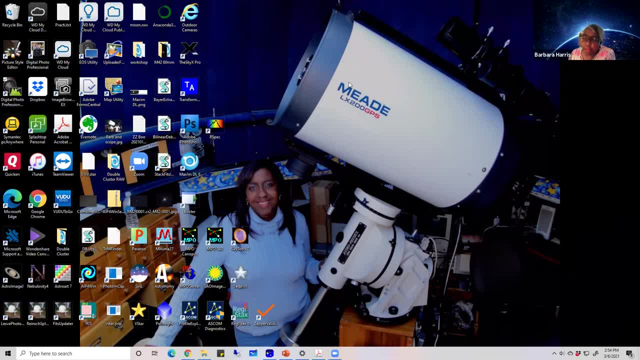 uh, the ADU value of your star. So, um you like in in Maxim, you just put the cursor over the star and um you pull up the information window and it will, uh, it will say signal to noise ratio. 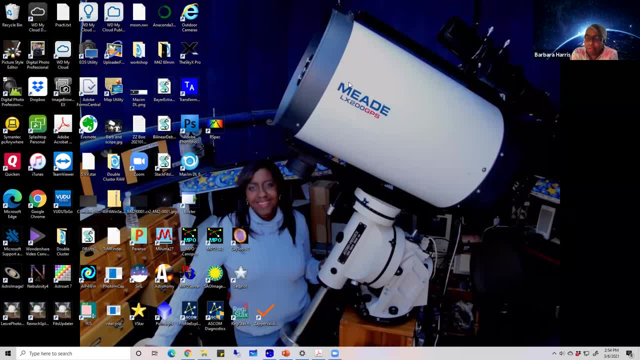 So, uh, in the information window in Maxim it gives you the signal to noise ratio or whatever you have your cursor over. It also gives you the full width, half max um of that particular star. So all of that you can see in. 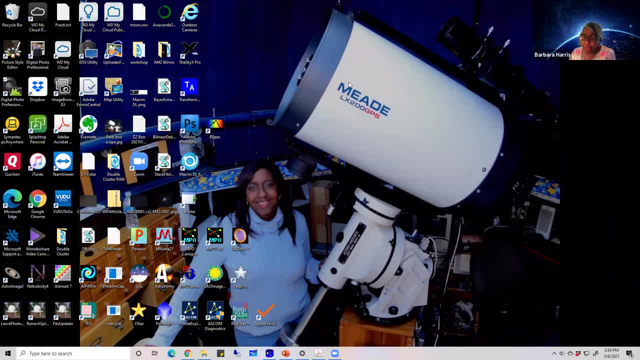 in the software, in in Maxim, Like I said, it's, it's. it's in the information window. Thank you, Uh. Antonio Celia has asked: uh, when you are setting out to shoot a target, do you take at the start some test pictures to analyze the safe exposure time and make sure that you're not out of the linear region? 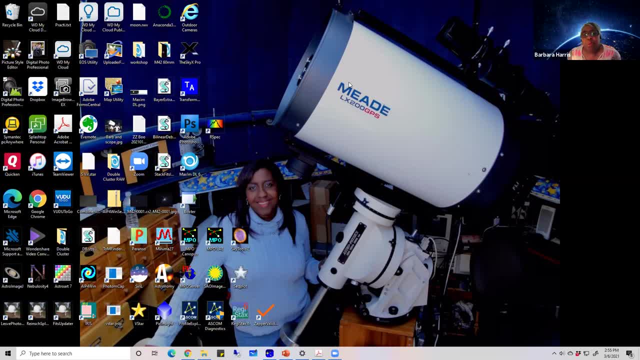 Yes, I do Um. like I said once, once you've had enough practice, usually, uh, you're going to kind of have an idea um, um like Delta CFI or like X per X per CI is one of my favorite DSLR targets. 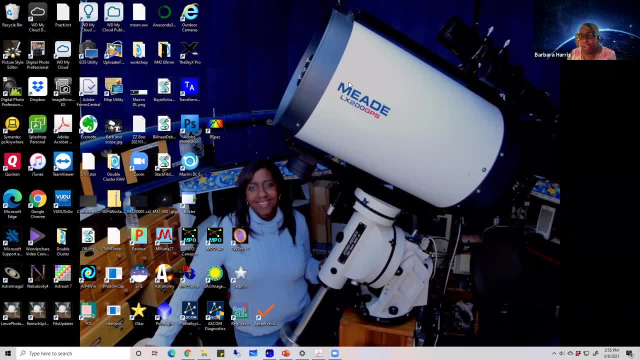 Our Corona Borealis is one of my favorite targets, Um so one I'll. I'll take a test shot, uh and, and I also have learned um what the comp stars in the field are, So I know that. 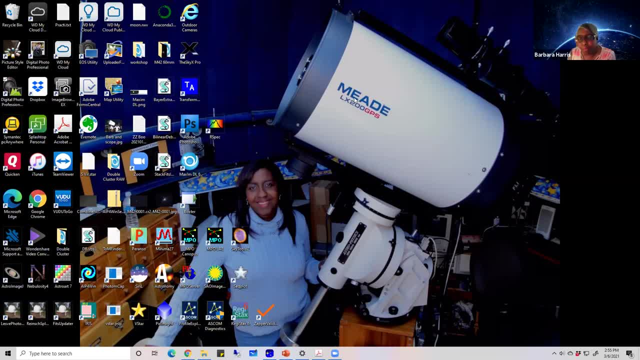 okay, that's my 6.2. So I'll, I'll look at that one and make sure that's not saturated, And I'll I'll put the cursor over, like our Corona Borealis, and make sure that that's not saturated. 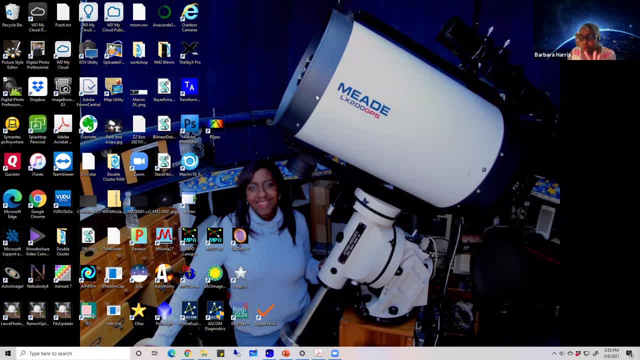 And if, if I take a quick image and I I can see, get an idea of what the um, the magnitude is by looking at the comp stars around it, uh, then I I know that I'm not saturated if I. 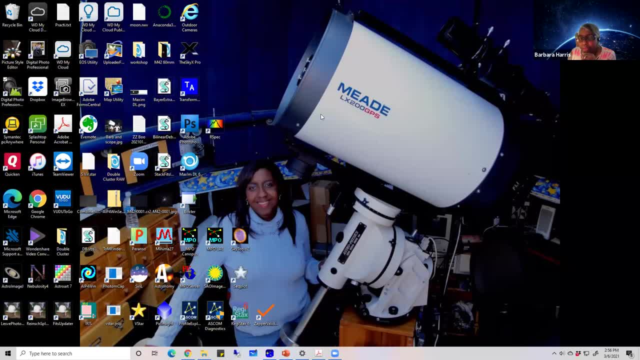 I know that my comp stars aren't saturated, Um, but, like I said, once you've done this enough, you get an idea of what exposure you're going to need for what magnitude your variable looks like. But uh, early on. 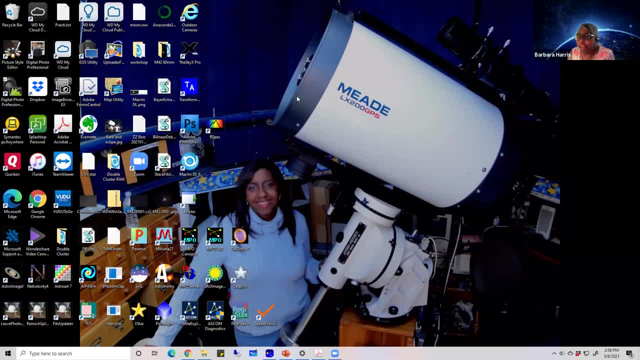 that's basically what I I would do is like I would take a a 20 second shot of my um, of my target, And I would take, I would take the card out and put it, go in the house and put it in the computer and look at the image. 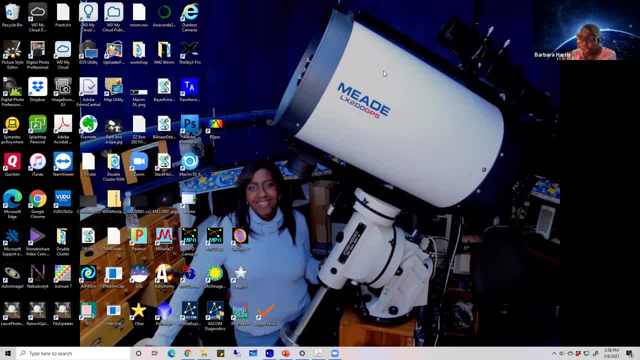 One. I would make sure that I'm pointing correctly and that my target and my comp stars are in the image. And then I I measure the full width, half max of um my target to make sure that it's it's the. 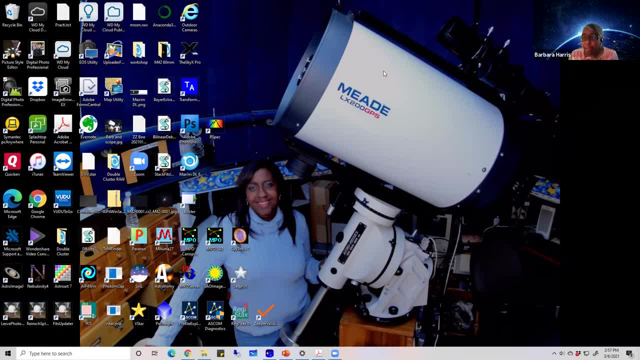 uh, star is spread out over enough pixels And then and then I make sure it's not saturated and that it's a good, decent signal to noise ratio. And if it's not a good signal to noise ratio, I'll extend it. 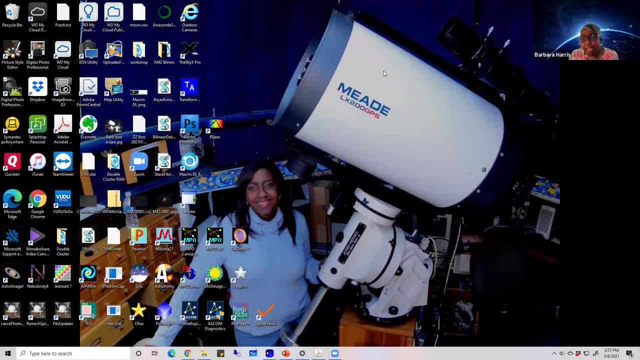 Um, sometimes I'll, I'll leave the exposure the same and just take several images, and then I'll, I'll stack. And if you're going to stack for DSLR photometry, what? what you do is you, uh, you, debayer first. 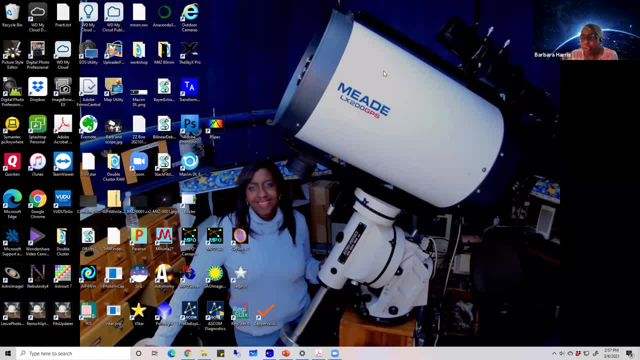 you extract your color channel and then you stack those color images together. So you debayer before you you stack, or you extract the green or red or blue before and stack those. Thank you, Speaking of stacking, the next question comes from Manmeet Vriti. 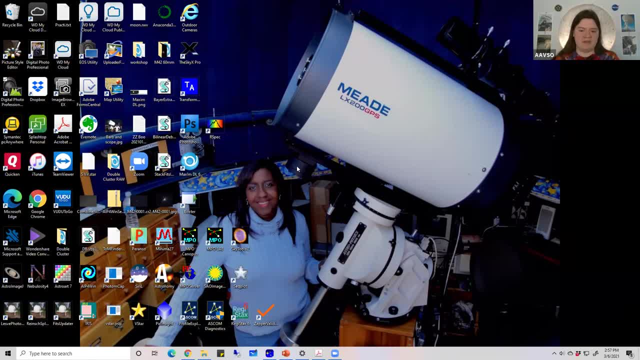 who has asked if there is a rule of thumb to calculate the number of images which should be taken, for example, with a DSLR on a 50 millimeter telescope. I'm sorry, repeat the question again. He would like to know whether there is a rule of thumb to calculate the number of subframes that should be taken for a stack. 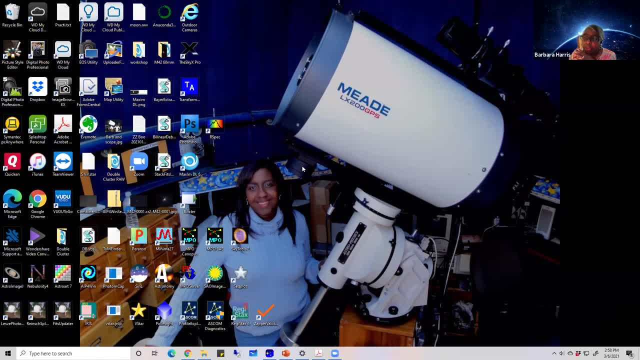 Well, it it basically depends on what your target is. Like I said you, you, you want to have a signal to noise ratio of at least a hundred for your target star. So, as you want to stack enough to get to that signal to noise ratio, 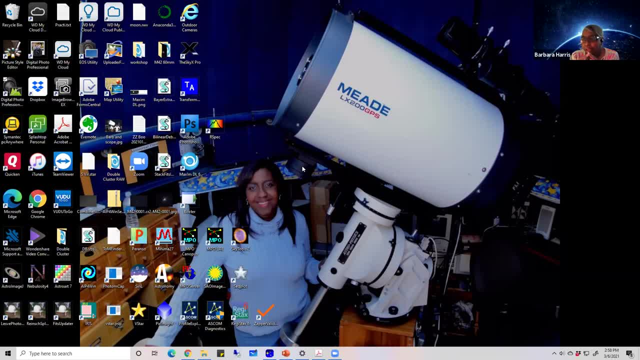 and it depends on how bright the target is and how many, and that determines how many images you'll need to stack. And sometimes it's just trial and error. It's like, okay, well, let's try five and see what kind of signal to noise we get for that. 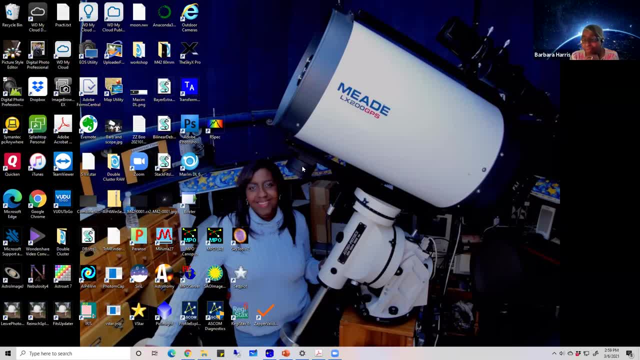 So it, it, it depends. Okay, Okay, Thanks. So our next questions are on the topic of software and I'm going to go ahead and combine these two questions that are very related, from Antonio Celia and Kevin Halsock. 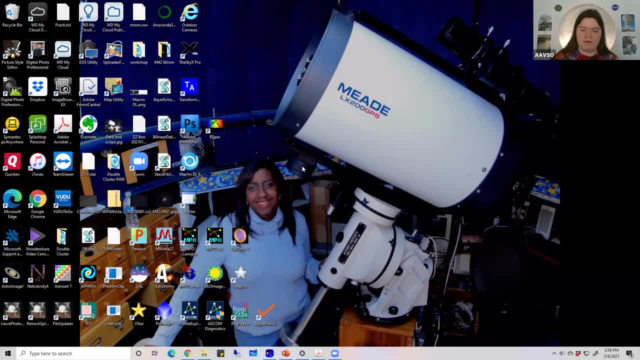 who have asked: what software would you recommend to use if you don't have Maxim DL? And what about Astro Image J? Is that? is that a viable option? You can use Astro Image J for photometry, but I'm not sure that you can extract your color channels from that. 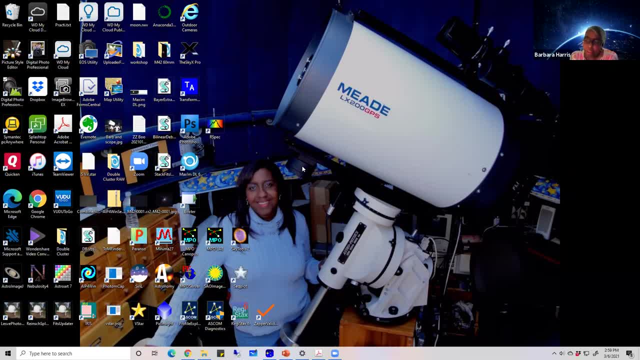 So you may have to do that in another piece of software And then you can. you can. once you extract your color image, then you can do photometry of that image in Astro Image J. One of the things that that can be difficult. 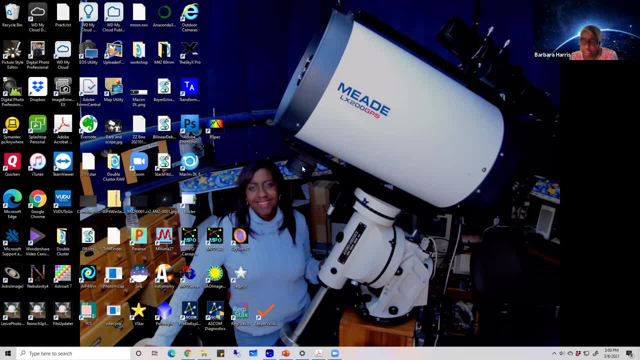 like I, I started playing with Let's Be Photometry. It's a great program for photometry, but that and and the same goes with VFoat also The way they're identifying their, the comparison stars- is that it 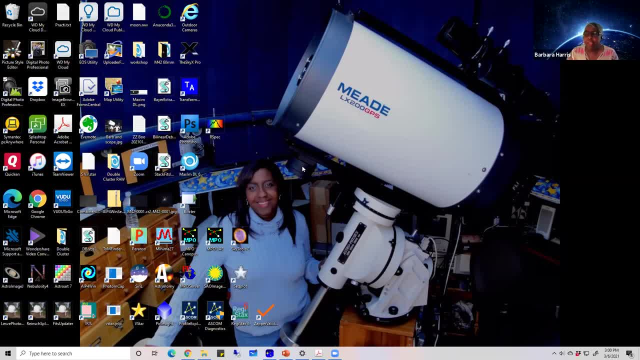 it does astrometry on your image so that it knows the coordinates of your variable and your comp stars in the image, And one of the problems with that is that when you defocus an image for DSLR photometry it makes it a lot harder to do astrometry on. 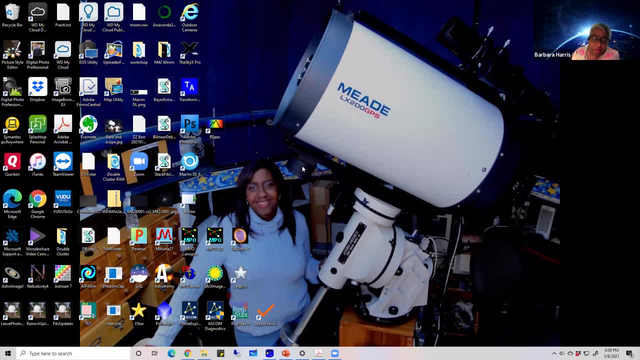 So I've had, I've I've tried VFoat and Let's Be Photometry, doing photometry with DSLR, but sometimes it fails because because of the defocusing routine that you have to use in DSLR photometry. 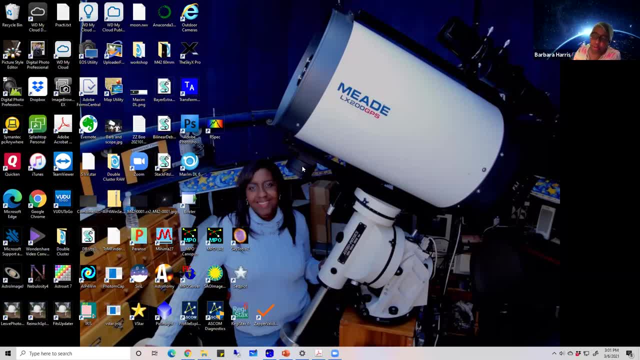 It's. it's a lot harder to to do astrometry on those I. I have used VFoat and Let's Be Photometry, but that's one of the issues of having to do astrometry to to identify your target and your variable stars. 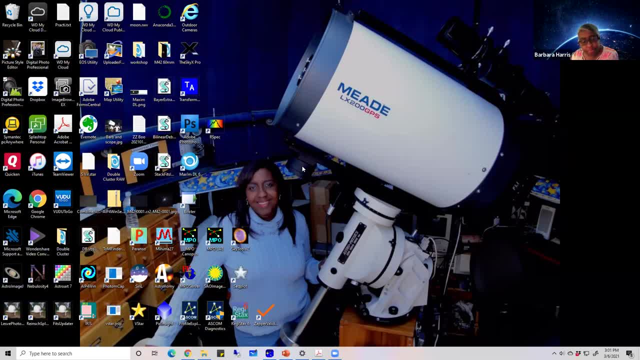 In AIP, for Windows and and for Maxon. you don't have to rely on astrometry. You basically you have to know where your stars are in the image like: which one is your variable, which one's your comp. 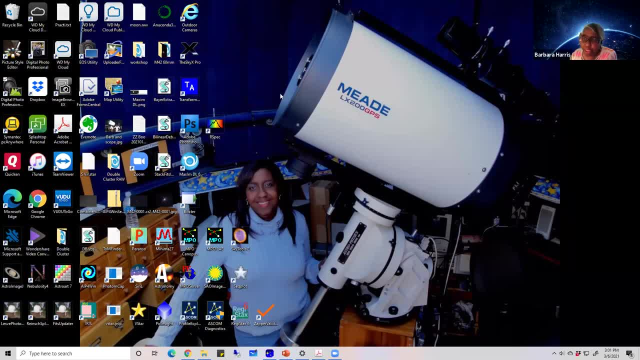 And you basically click on those, like in AIP, for when you you click on your variable and then next you you click on your. your comparison stars in the image. So those I like that for DSLR photometry because sometimes because of the amount of defocusing, 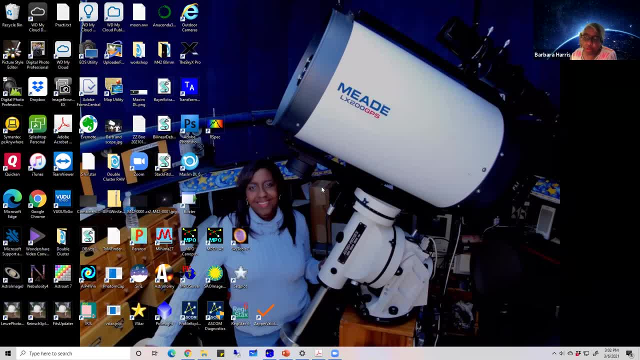 it can be difficult to to do astrometry on those images And, like, like I said, VFoat and Let's Be Photometry relies on astrometry to identify the variable and the and the compare comparison stars Also Iris. 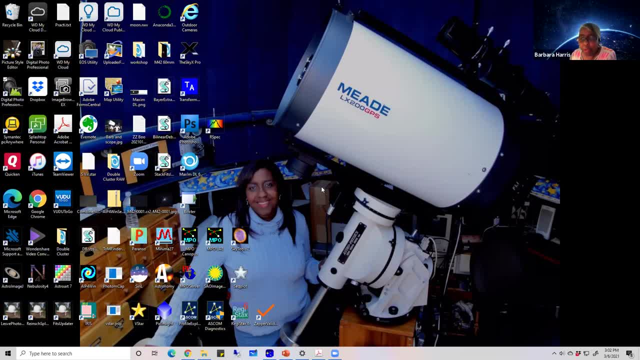 you don't need to rely on photometry. Iris is a great program that does everything, but it. it does have a steep learning curve. It can be it takes some effort to learn how to use, but it's a great program because one 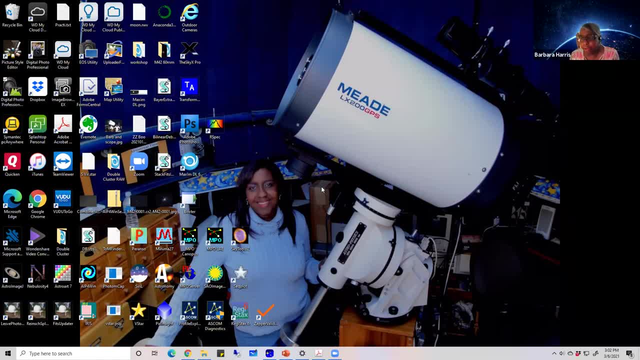 it's free and you can do everything in Iris. You can extract your color channels and and do photometry, do do your image calibration, do photometry- all in that one package. So it's a nice program, but it it takes some effort. 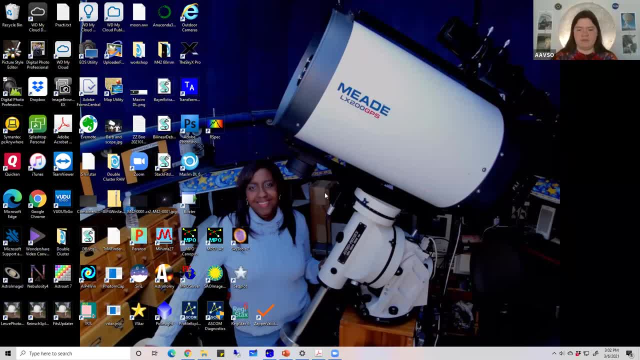 Thank you. We have two last questions here about software Should be pretty quick ones. Ken Mayfruit has asked: what about PixInsight? Is that valuable for photometry? Yes, Like I said, I I just purchased PixInsight and you actually can't do photometry in PixInsight. 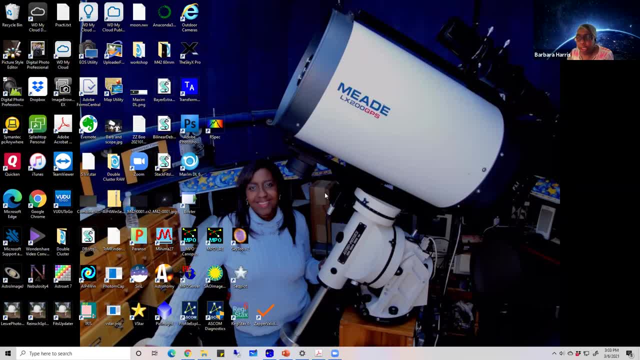 but everything up to the photometry. PixInsight is great for doing And, like a few nights ago I did, I collected images for for ALGOL. Beta Persei is an eclipsing binary And I have 197 DSLR images for ALGOL. 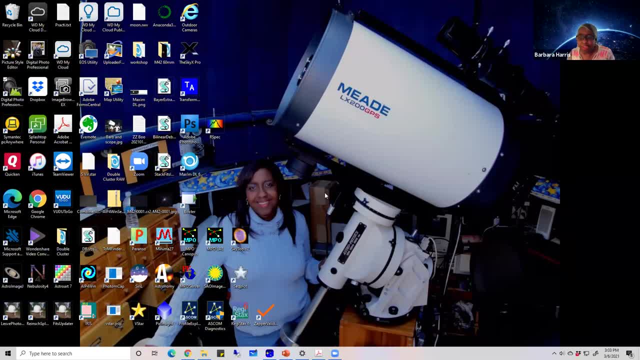 And some of the programs for for batch processing a large amount of files like that for for Maxim. it is good batch processing that for my image calibration. But when it comes to extracting the color channel, the green channel, to, there's no good batch processing routine for that and Maxim. 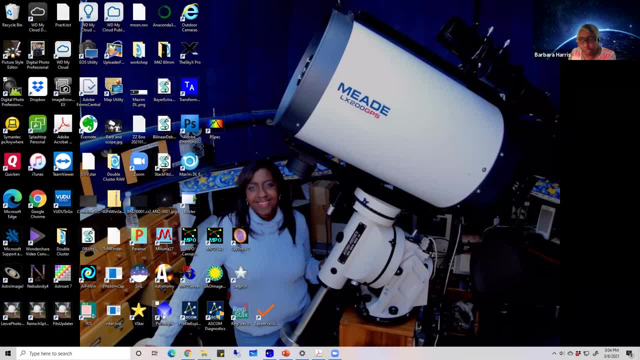 So PixInsight is has a great script for batch processing that where what I did for for that particular group of images, those almost 200 images, is that I did a a bilinear demosaicing routine in PixInsight on all of the 197 images. 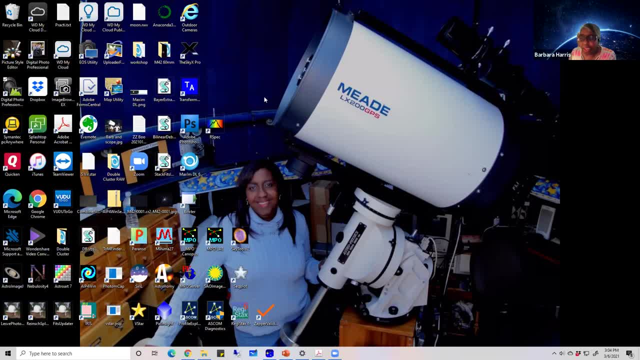 And then there's a script in PixInsight where you can extract a color channel. You basically tell it to extract the green channel and it saves those images. And then you you can't do photometry in PixInsight, but then you go to another program to do your photometry. 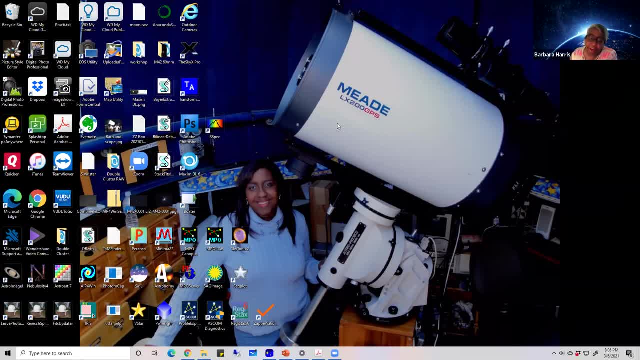 So that's one great thing, Like if you have PixInsight that you you've been using to do pretty pictures, you can do some of the work in PixInsight, but you can't actually do photometry in PixInsight. 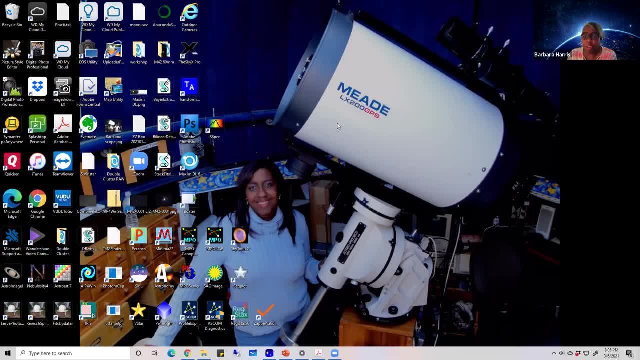 but it has a lot of great features for doing the preliminary work up up to doing the photometry. Thank you, Let's see, while you have been answering, that we've had a couple extra questions about software come in. We have. Timothy Weaver has asked about using Serial. 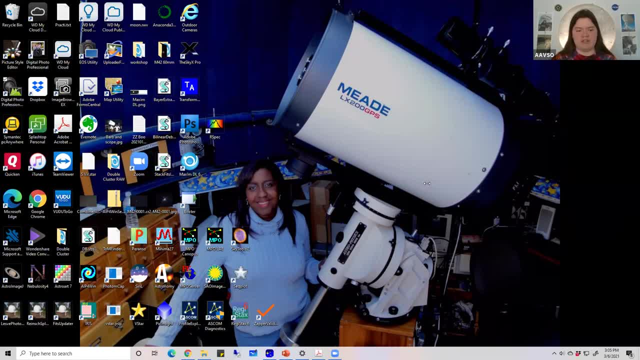 which he says extracts the color channel and converts the DSLR images into fits files. He wants to know if that would work suitably. Yes, actually I just found out about Serial about a week or two ago and started playing with it, So it will do almost everything I just explained in about PixInsight. 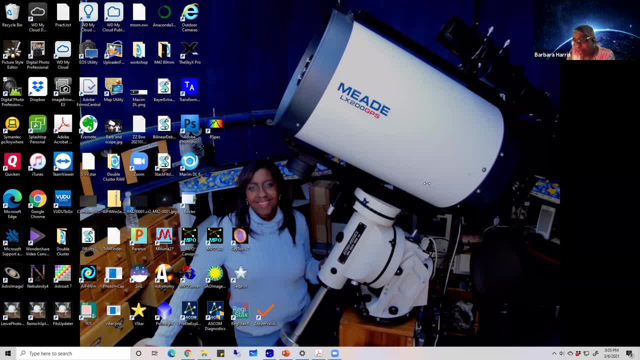 You can do that in Serial. Now, you can't do the photometry in it, but you can do everything else like calibrate and extract the color channel in Serial, And it's a free program. It's actually a great program And it basically does the same thing that I talked about in PixInsight. 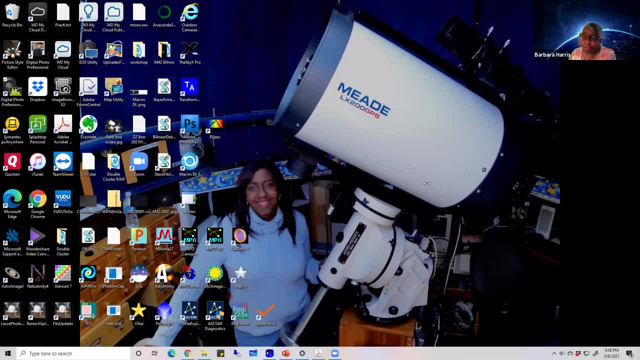 You, especially if you have a ton of images, like 40 clips in binary, like I had from a few nights ago, and it takes a long time. like DSLR, images are very, very large. So almost 200 images of DSLR images. 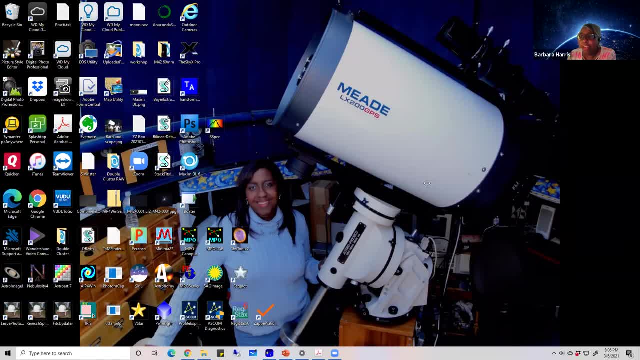 It actually took me a few hours in PixInsight to calibrate, to do a bilinear debayering and then to extract my green channel. So it took a few hours for those two almost 200 images. But that and Serial are pretty good for that. 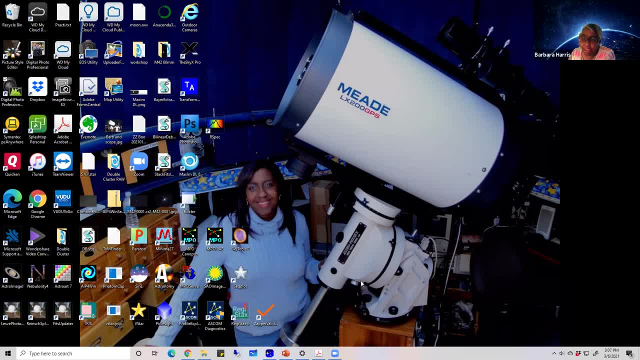 especially when you have a very large amount of files like that. And, like I said, I like to do eclipsing binaries, So usually I have a minimum of about a hundred files for an eclipsing binary that I'm doing photometry for. Thank you. 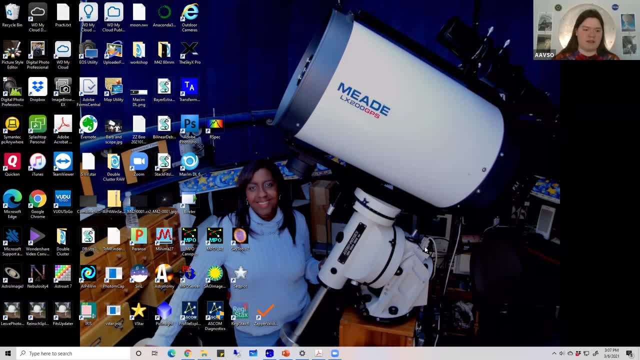 Now we're going to move away from from the software questions and start asking. Actually, I just noticed one quick question that says: can I use the filter? You don't want to use additional filters for your DSLR, just what's in the camera. 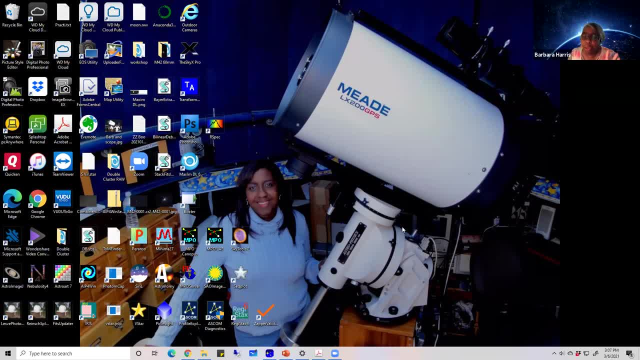 Like you don't want to use light pollution filters or anything like that. All you're going to do is just use what's in the camera and then extract those, those color channels from the Bayer filter Array, So you don't use any additional filters for DSLR. Thank you. Also, while I'm looking at it, someone asked: can I stack images of a star taken over different nights And that's not recommended that these are variable stars, So they may be different magnitudes for different nights. So you don't want to stack from different nights. 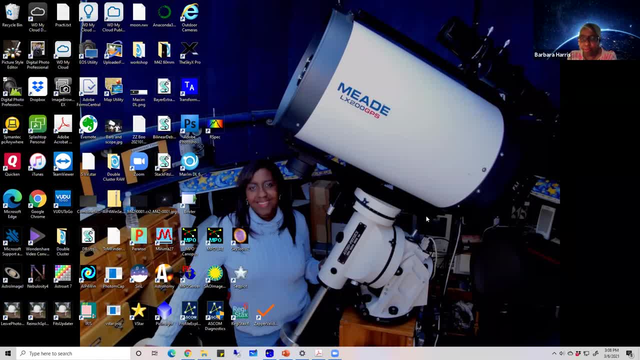 If you're going to stack, it needs to be from a very small window of of of shooting And it depends on on your, on your star Also, like if you have some cataclysmic variables that have some variability every two minutes or so. 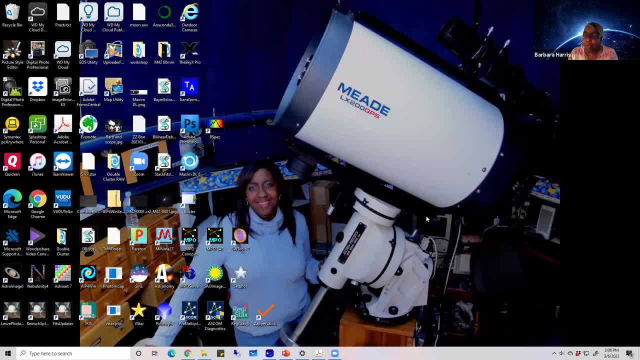 you know you don't want to stack those because you're going to lose that variability by stacking them. So something like a long period of variable, like a Myra or Delta. CCI is a pulsating variable with a period of about five days. 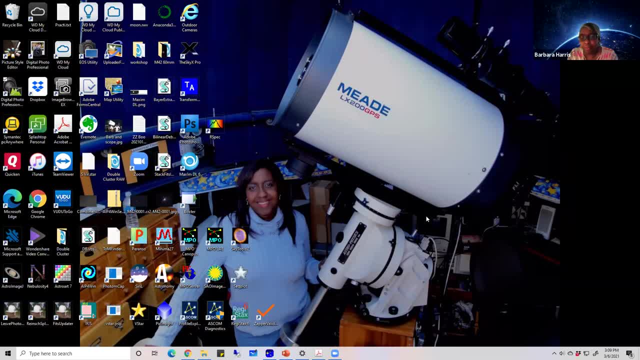 I believe So. so taking you know, 10 minute window of images and stacking those isn't going to affect the variability. But if you have Delta CCI from one night and then Delta CCI from another night, you need to do those separately. 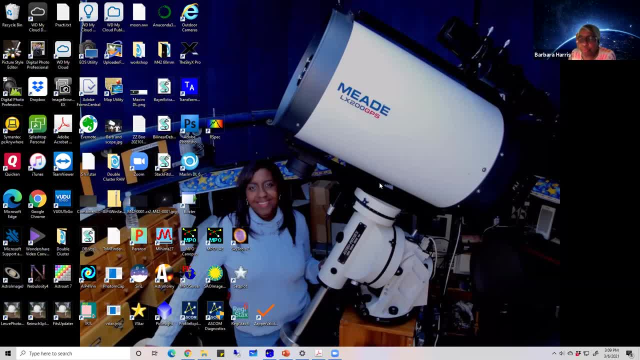 You can't stack those, Okay, Thank you. So, oh, I've already done that one. We have a question here from Stephanie Cyphers, who has asked: how much does using a tracking mount affect the photo or make it blurry due to movement? 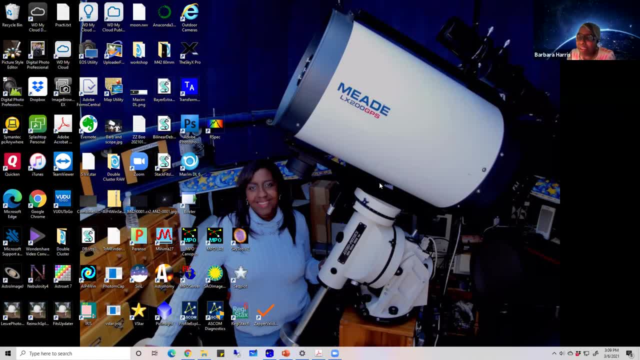 I'm sorry, I was reading a question and wasn't paying attention. The question was: how much does using a tracking mount affect the photo or make it blurry due to movement? Well, because it's tracking, it shouldn't be. it should not be blurry. 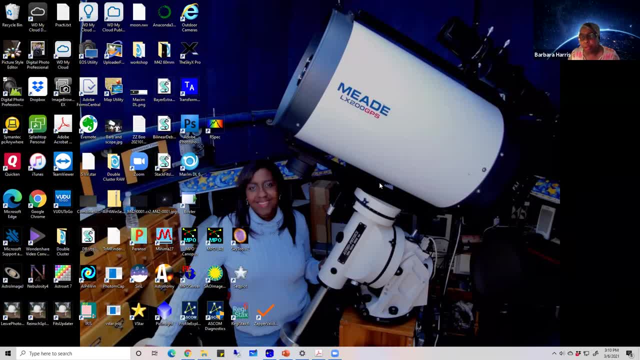 So if you have a tracking mount that's accurately polar aligned, if you're tracking your target, there shouldn't be any blurring. Your, your, your star should remain round. You shouldn't get any trailing. So you shouldn't have any blurring if you're tracking. 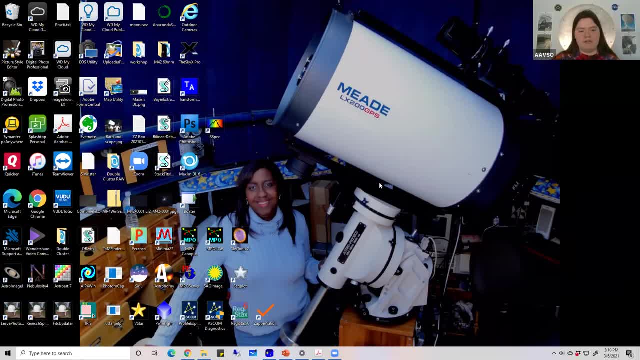 Thank you. Kevin Halseig has asked: how do you define bright stars With respect to a tripod mounted DSLR Beetlejuice? for one Ones that I typically use, the tripod is Beetlejuice Delta, Delta, CPI could probably. 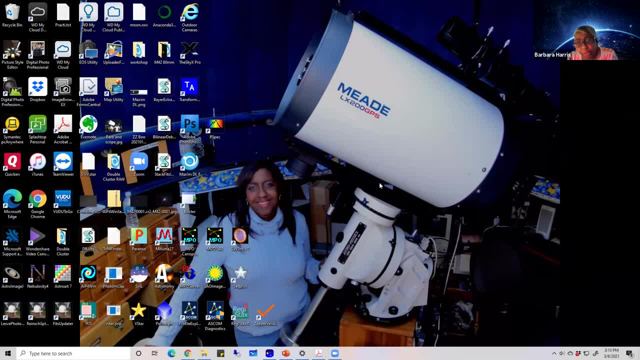 I could use a tripod, Epsilon or Rigi. I can use the tripod because those are going to be very short exposures And when I say short exposures, I never go below 10 seconds because if you, if your exposure is too short. 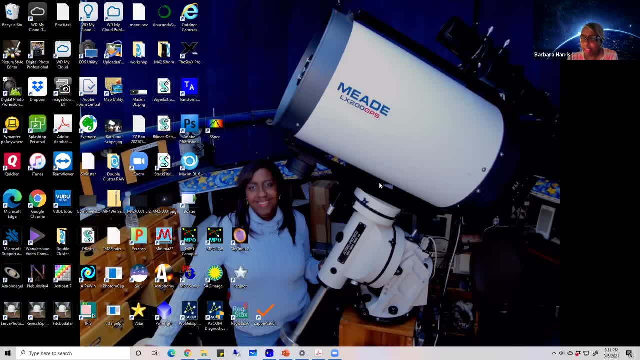 you could get inaccurate photometry because of scintillation of the atmosphere where the you know, there's always some turbulence in the atmosphere And if you're using too short of an exposure you run into getting inaccurate photometry because of that. 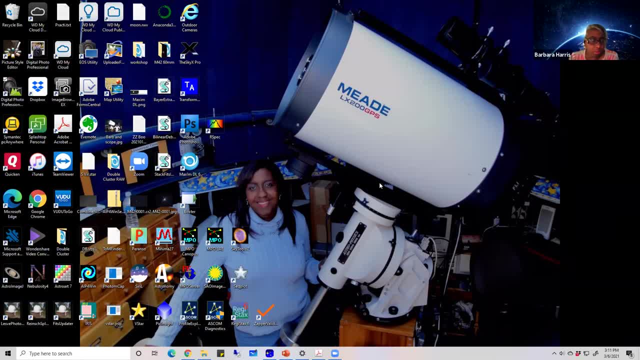 And if you have to go to a very short exposure, shorter than like 10 seconds, then what I would recommend is that you stack like a minute's worth and hopefully not get saturation, but at least it's enough to even out the scintillation. 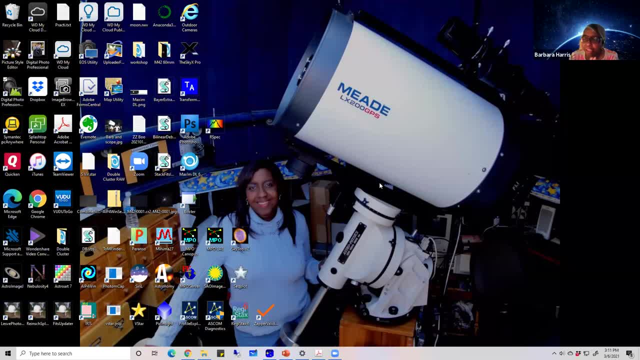 and not be affected by that. So I never go below 10 seconds, And with a target like Betelgeuse, 10 seconds is still too bright. So if you don't want to go below 10 seconds, then your target is still very bright. 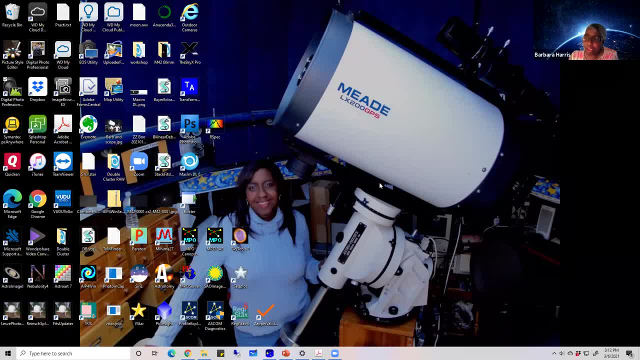 There are two things you can do. One, you can increase the f-stop. So I usually take Betelgeuse at an f-stop of like 5.6 or a little bit higher. And the other thing you could do is you can use the lowest ISO setting. 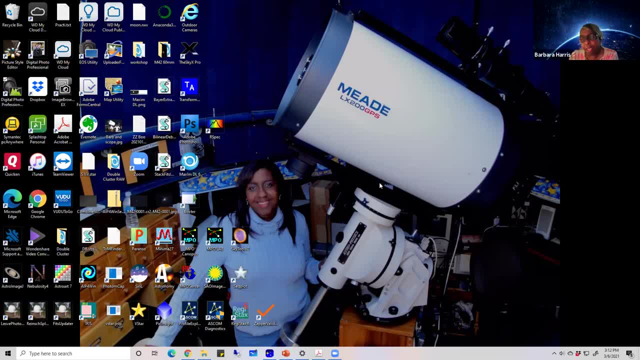 So, even though for my Canon 70D, the ideal ISO setting that gave me a gain of one electron per ADU, I use 100 for Betelgeuse because going to a lower ISO setting, I won't saturate as quickly. 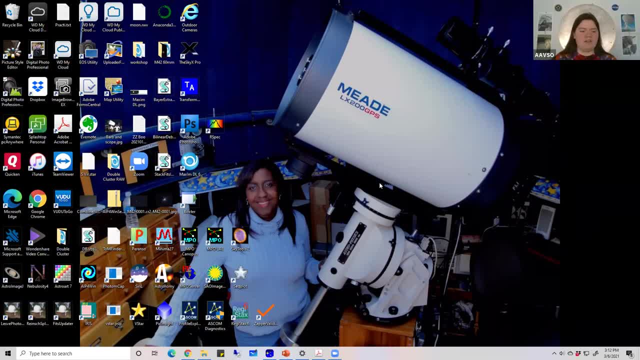 Thank you. Let's see, We have a question here from Blake Nancrow, who is asked: high f-stop numbers will create big diffraction spikes. Is that something that you want to avoid for photometry? Yes, OK, Thank you. 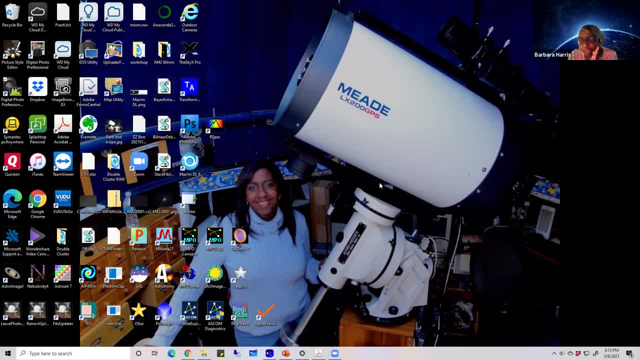 Like usually, I try to keep my f-stop for my lens like between f2.8 and f7.. I try to stay in that range. And while I'm staring at the question, someone- Andre- asked if there's an up. 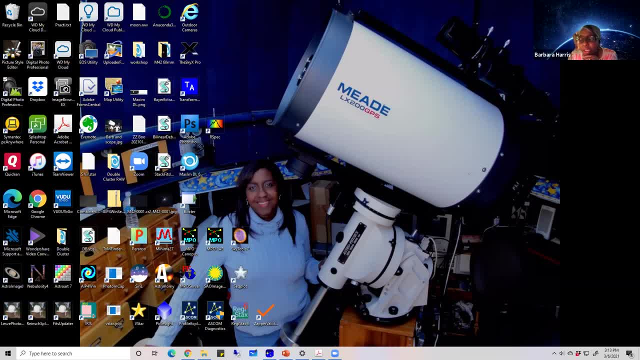 is there going to be an updated version of the DSLR observing guide specifically including prime focus photometry with the telescope? I'm not sure the guide or there's any updates plan, But everything I've basically mentioned can apply to prime the focus of a telescope also. 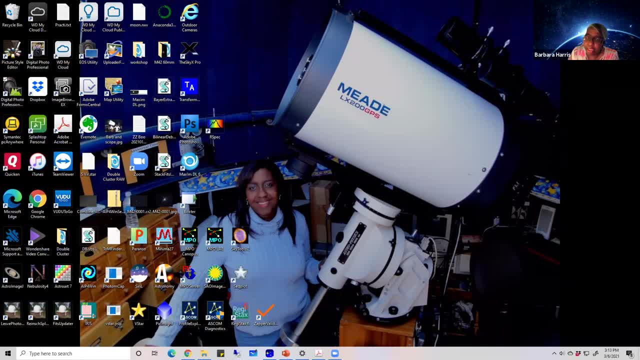 Like part of my photometry, I use an 80 millimeter refractor with a Canon 40D attached, So everything I mentioned applies to that. The difference between that and my 85 millimeter lens and my DSLR is that the telescope is going to have a smaller field of view. 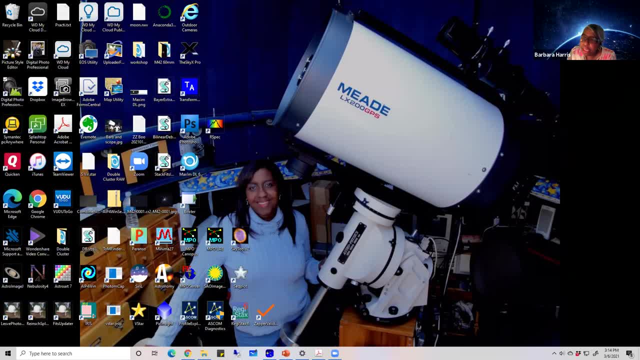 So you might be limited, Like you're probably not going to be able to do Betelgeuse through a telescope because the field of view is going to be too small that you're not going to be able to find comparison stars that are bright enough to use as comparisons. 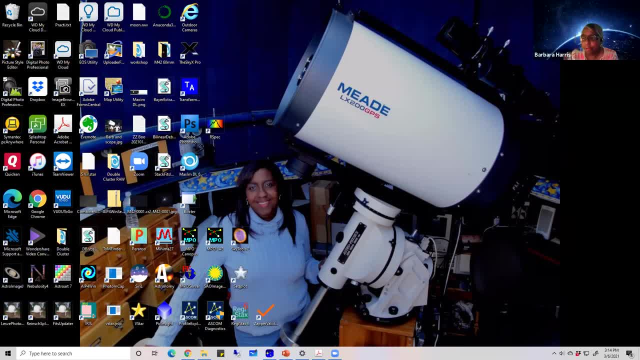 That makes sense. Yeah, So everything I've said applies to a telescope also. It's just that you're going to probably have different targets to choose from compared to your lens, Thank you. While we're on the topic of education, let's go ahead and take some of the other questions related. 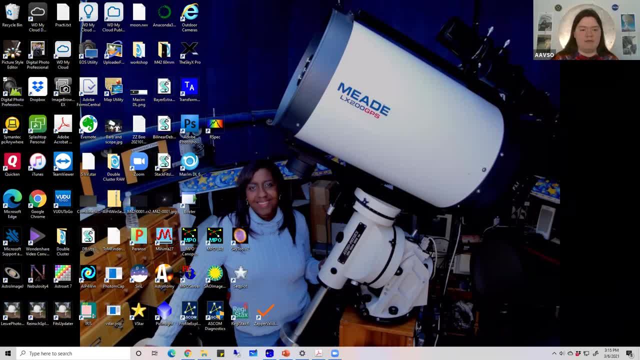 to that, like this one from an anonymous attendee who would like to know when will you be giving the next DSLR choice course? I'm not sure. I taught a few of the DSLR choice courses and I noticed. I'm not sure if he's still on here. 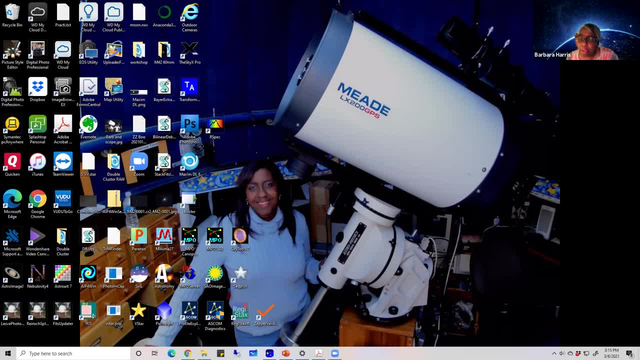 but I noticed at the beginning that Mark Blackford from Australia was on here and I took my DSLR course from him, So there are only a few of us that are willing to give the course And because of health reasons, I had to stop. 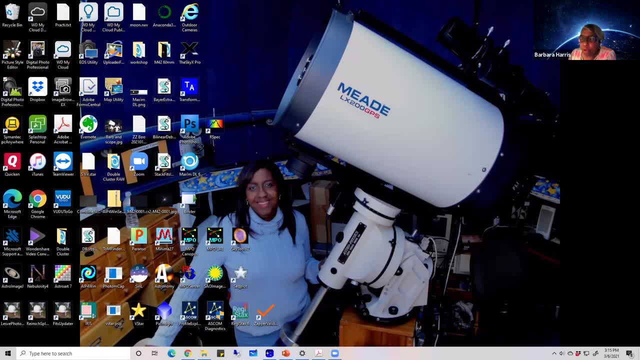 I enjoyed it, but it became overwhelming Because we had recommended assignments due and everybody wouldn't turn in their assignments on time and you can't go to the next step until all the assignments were in And it was tough for me to do as a course. 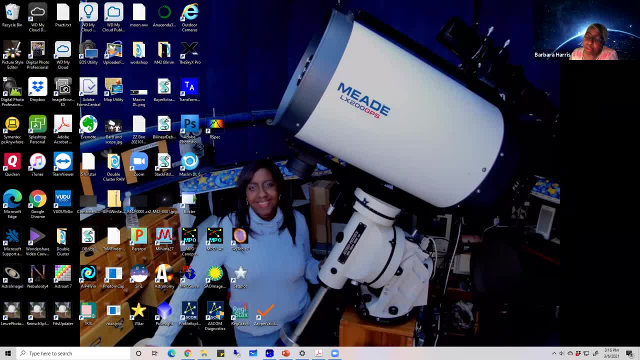 Now I do a lot of mentoring but I'm not sure if I'm going to be able to give another DSLR choice course Or who's able to give one. That's been one of the problems. why they haven't had one in a while is 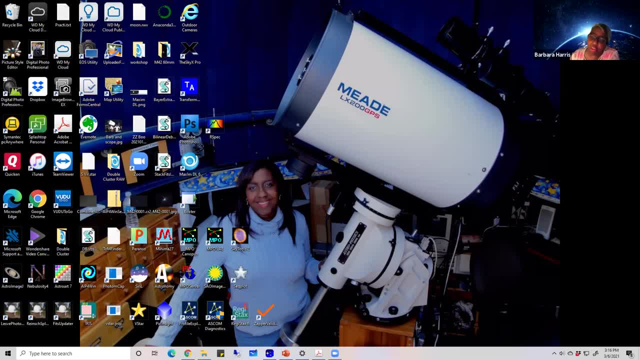 they haven't been able to find anyone that's willing to teach a four-week choice course, But I do. DSLR mentoring, Thank you. Speaking of mentoring, we had a question in here which I don't see. There we go. Cameron McEwing asked it. 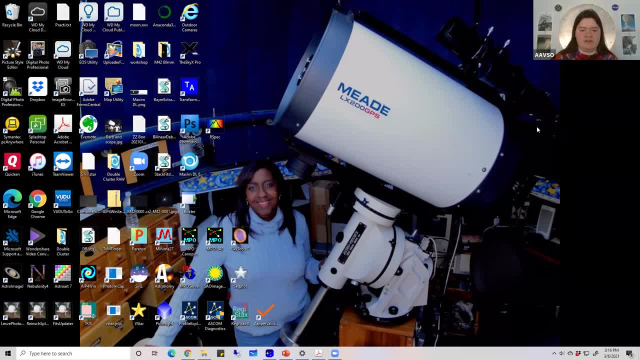 How do you connect with A mentor for DSLR photometry? Well, the mentoring program is open to any AAVSO member, So you have to be an AAVSO mentor to start with, And if you're interested, I'll see what page it's on. 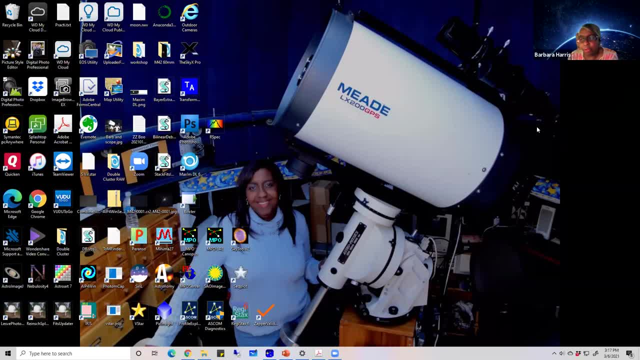 But if you search the AAVSO website, if you put into the search block, mentor Sebastian Otero is the head of our mentoring program, So he basically gets an idea of what you're interested in learning. Like is it DSLR? 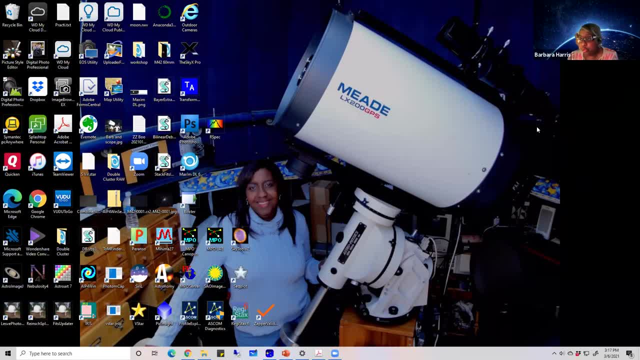 Is it CCD visual? So he gets an idea of what you're interested in And then he assigns a mentor to you. Or some people say I heard Barbara Harris gave a lecture on DSL, Can I have her as a mentor? So some people will request. 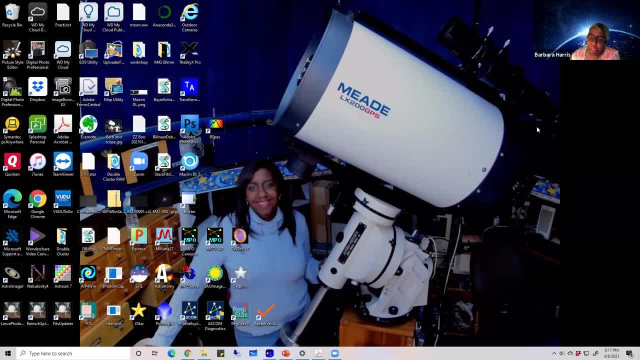 But the easiest thing is to go through Sebastian and let him know that you want a mentor and what you're interested in, what your goals are. All right, Thank you. I see we had a couple of questions here from people who would like to know. 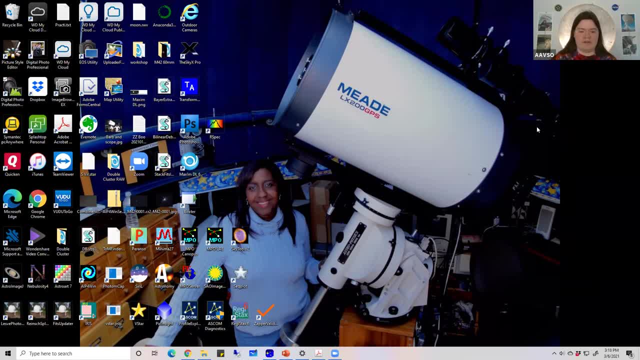 if they can obtain a copy of the slides for your presentation for reference. Sure, I can make them available. I'm trying to figure out how, But maybe you can tell me how I can. I think we will be able to figure that out if you're willing. 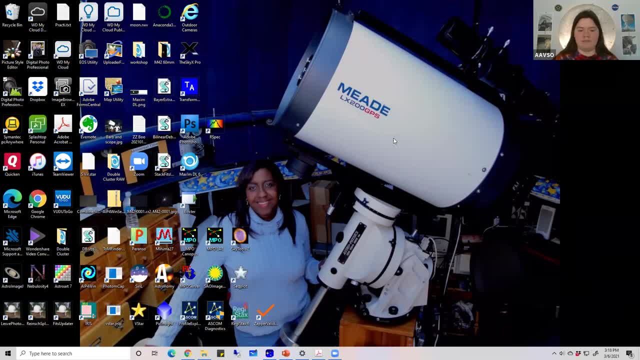 I think we can probably send an email to all of the attendees of the webinar, considering that they did register with their email addresses, So we can as a resource. OK, All right, Great, Thank you. OK, So we're going to go back to some of the more. 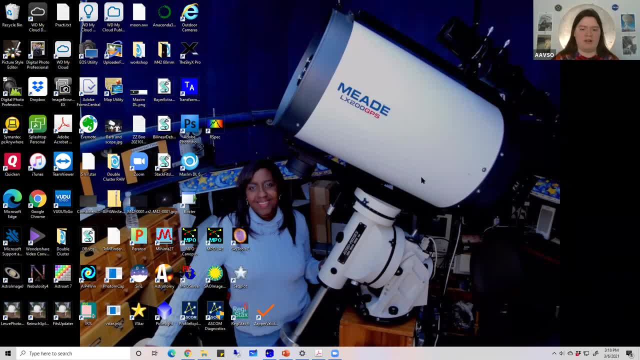 technical questions now. We had quite a few questions about the cameras themselves. One recurrent theme was: does it matter what the white balance of the camera is set to? No, it really doesn't matter what the white balance is, So you don't need anything special for white balance. 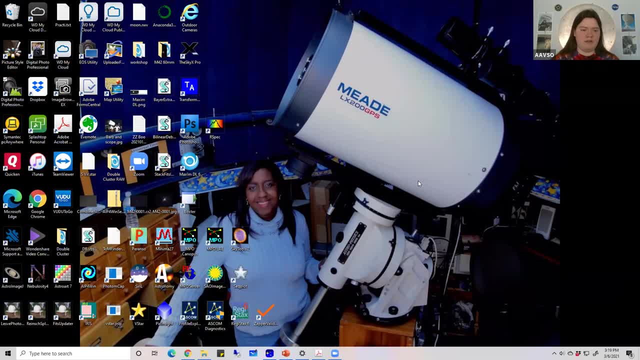 OK, All right, Thank you. We also had a question here from Mike Ashby, who asked: what does ADU stand for? It stands for Analog to Digital Unit. Like I said from the beginning, most DSLR cameras are 14-bit. 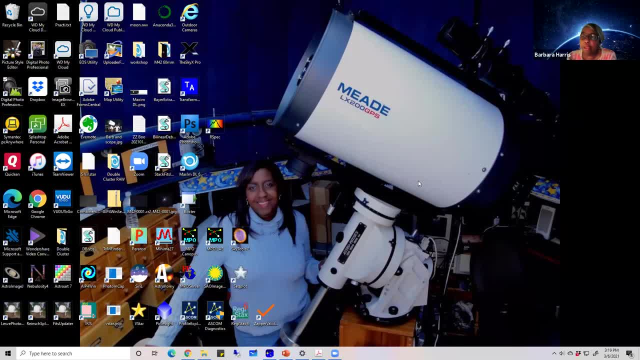 meaning that they have 16,384 levels of gradations, from 0 to 16,384.. And there's one ADU that's between 0 and 16,384.. So ADU stands for Analog to Digital Unit And, like I said, the gain of the camera. 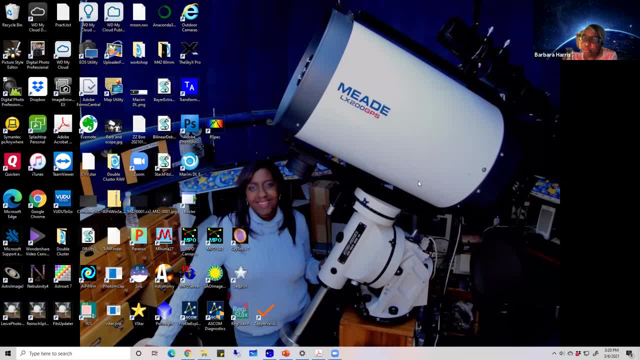 is how many electrons it takes to move from one ADU to the next level. OK, Thank you, Let's see. OK, A couple of questions here that came in earlier. There was one where we had people asking about if you know what the best photometry software for Mac OS would be. 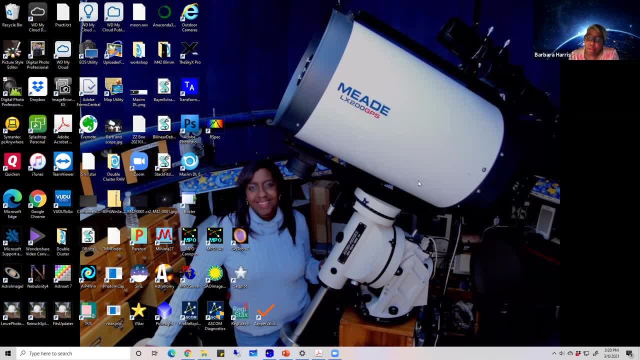 No, I don't. unfortunately, I'm not familiar with Mac at all, So I'm not sure what the best software would be. Thank you, So we had a question here from Antonio Celia who had asked so when you submit your photometry data to the AABSO? 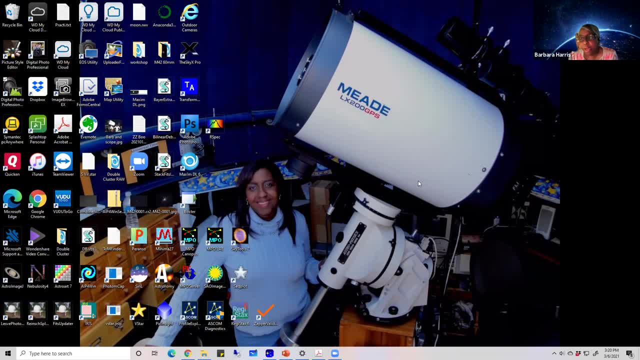 it is not transformed. correct, Correct. So when you submit your data you have to put what filter you're using And, like for my CCD images, I'm either using a B photometric filter, a V photometric filter, an R. 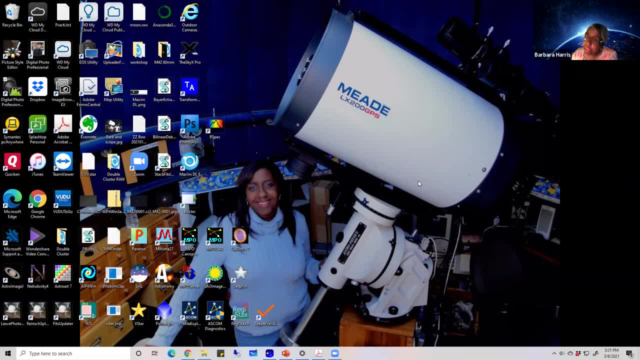 a Cousins photometric filter or an infrared Cousins photometric filter. So I'd list one of those as my filter. But for DSLR you're going to submit TG for tricolor green, TB for tricolor blue or TR for tricolor R. 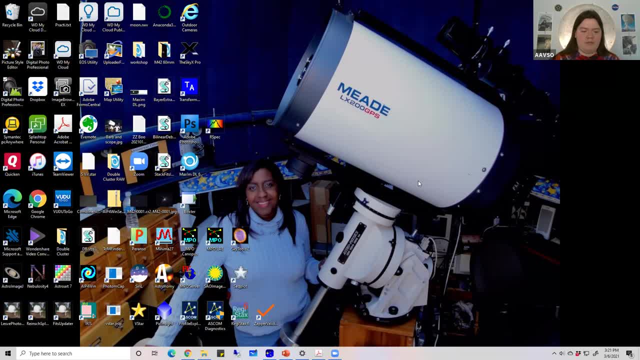 Thanks. Going back to you, We have some questions about cameras. We have a question here from Gary Shaw, who had asked if you can point out any key differences between the process that you've outlined and the process that would be followed if you were working. 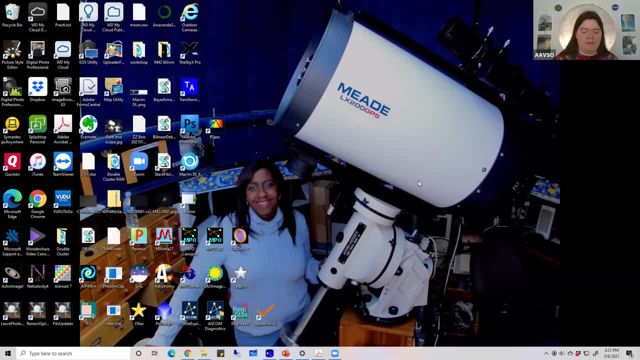 with a CMOS camera. I think some other people also mentioned. Yeah, actually I was going to mention that If you have a one shot, one color CMOS camera, it's probably identical to what I've been saying here, Where you're going to set the gain at a certain level. 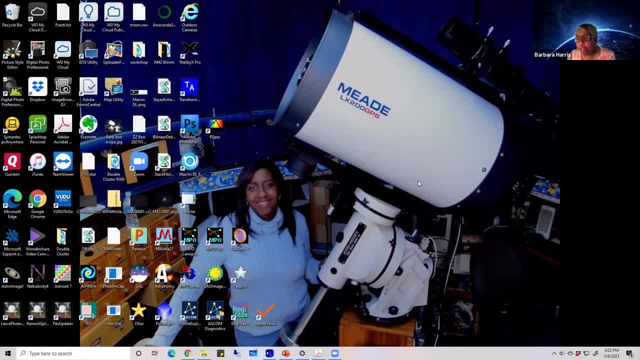 If you're working with a one shot color camera, you're going to extract the color channel, just like I said for DSLR. So there isn't any reason why you can't basically do what I've talked about here for a one shot color CMOS camera. 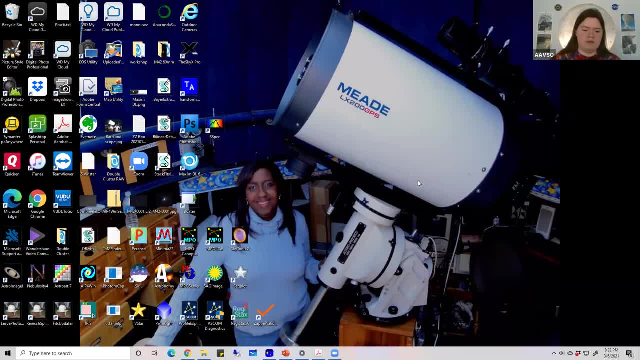 Thank you. All right, let's see. I think there were some other questions here about cameras. Yes, that's right. Gary Hawkins had asked: do temperature variations affect the accuracy of the photometry when using an uncooled DSLR? 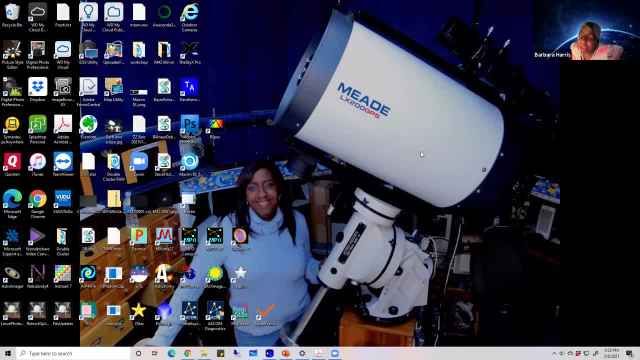 Well, cooling is nice. That's why CCD cameras are a lot better And unfortunately there's no cooling with the DSLR. but that's why you do dark frames And you try to do your dark frames very close to when you do your science images. 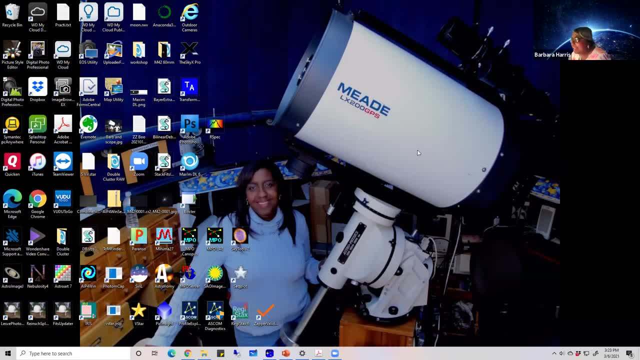 so that the temperature is pretty close. You're not going to get almost identical temperatures, but you're going to get pretty close to what your science image temperature was. And for a cool CCD camera you could take your dark frames at different times. 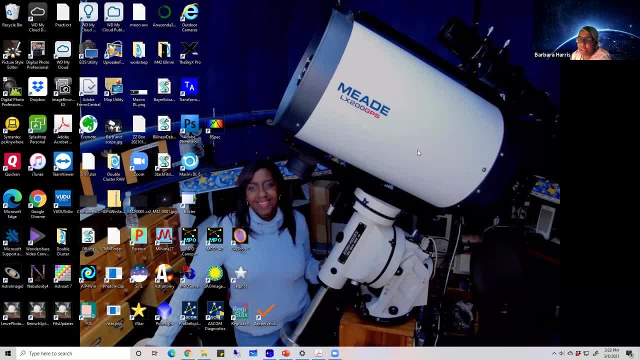 where, like, suppose you take a one minute image of your of a particular field for a CCD camera, You could actually use a different timed dark frame than your science image and you could scale the dark frame. For DSLR cameras, you can't scale them. 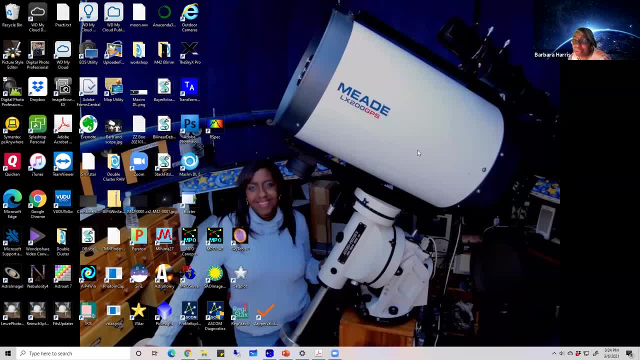 They need to be the same temperature and the same time as your science images, So like if you take a 30 second image for your science image, your dark frame needs to be 30 seconds also And it needs to be the same ISO setting, the same f-stop. 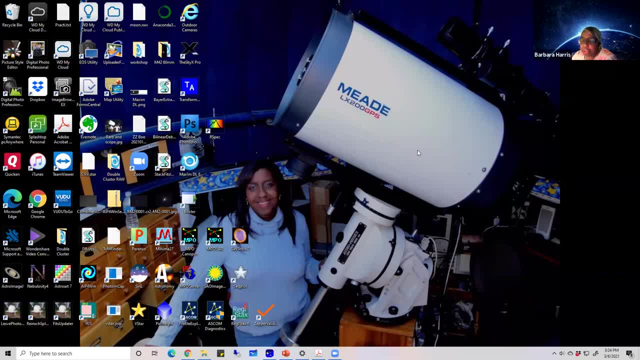 everything else the same as your science image. Thank you. We have a question in here about slides. Kevin Whitman has asked: can you use a computer monitor with a white screen activated, for example from YouTube, for an evenly illuminated field for the flats? 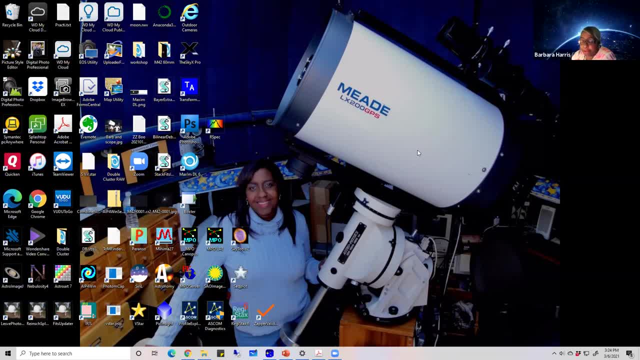 Yes, people have done that for flat fields, basically using a white computer screen. Also for my DSLR. before I purchased that EL panel, I would also use a that I purchased from Amazon- a little tracing panel- that a lighted tracing panel. that was pretty cheap. 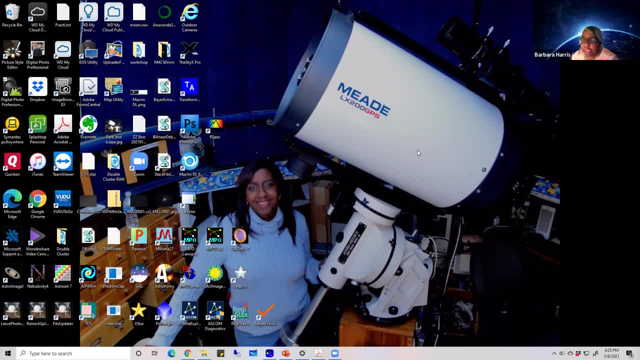 And that gave me great flats And they're pretty inexpensive. but you can use like an iPad or computer screen that has the white image up there and take your flats from there. Thank you, Now let's see, We have actually several more questions coming in here. 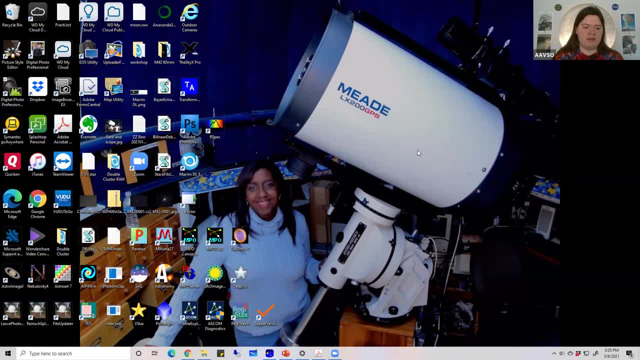 that are about cameras. So we have a question from Howard Moores, who has asked: can you use a grayscale setting on a DSLR along with BVR Johnson-Cousins filters? I'm not sure how to do that, Because when you're taking an image with the DSLR, 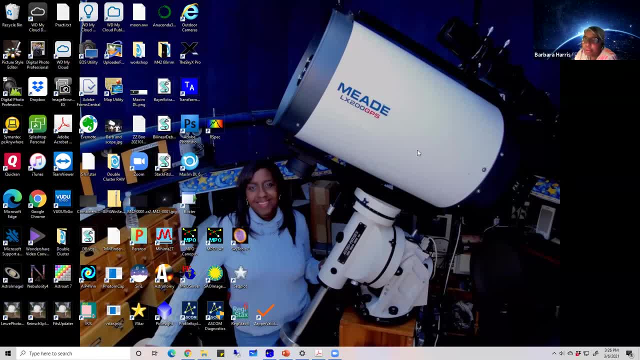 the filters are right in front of the sensor, So your image is gonna include that filter data. So I'm not sure how you can not take a color image from with the DSLR. Yeah, thanks. So Burt Watson, on a related note, has asked: 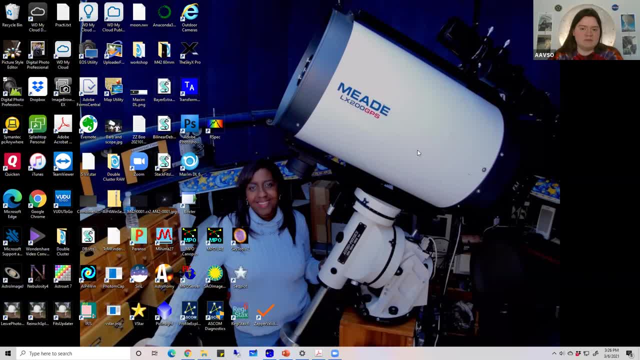 is it easier to use BVR Johnson-Cousins filters Or is it easier to use a monochrome camera? If you're gonna use a monochrome camera, you still need a filter in front of it. So, like my CCD ProLine camera is a monochrome camera. 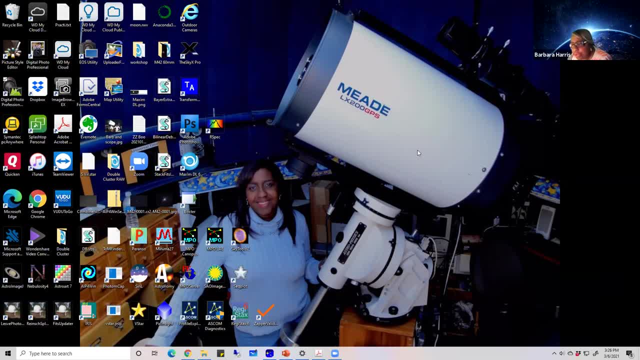 and I have a set of filters, So the majority of photometry is with color filters. Now there are some stars where they're more interested in just the timing, like an eclipsing binary. Sometimes you're not concerned with the absolute magnitude, You're interested in what time? the minimum. 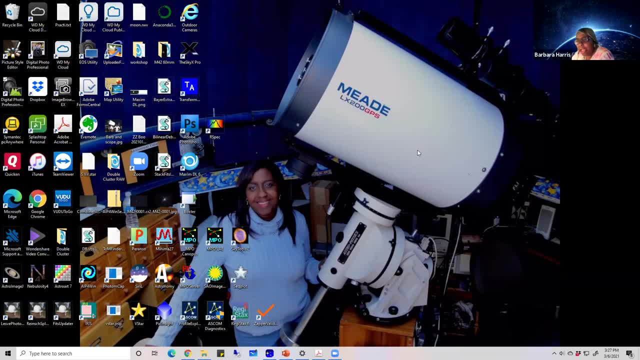 of that eclipsing binary happen. So sometimes, especially if it's a very dim star, they might use a monochrome camera with no filter At all, or clear filter so that you have a lot more light reaching the camera, but I would say 99% of data that you're. 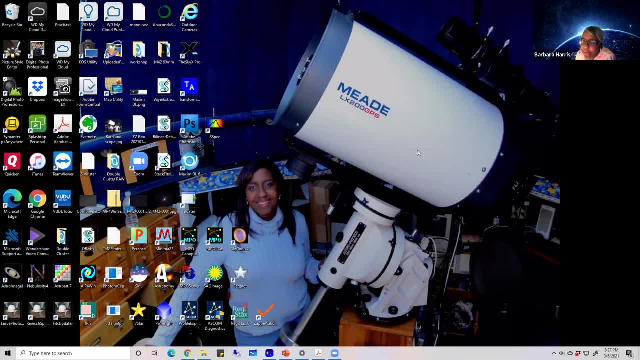 submitting to AAVSO is filtered data with photometric filters or tricolor color filters. Thank you, And usually monochrome cameras are a little bit more sensitive than color cameras, So so if you have a monochrome camera, that's great. 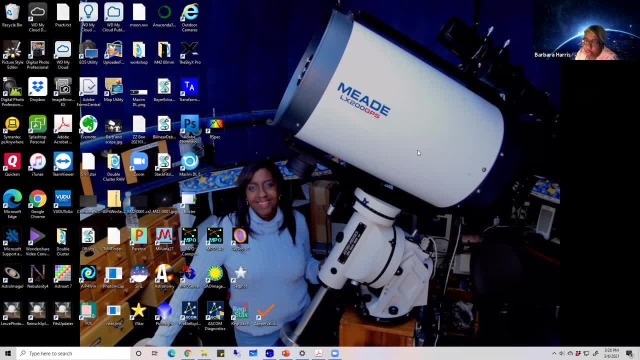 but you still need a photometric filter with it. usually, And if you're only going to get one photometric filter, a photometric V filter is what's usually recommended. So, relatedly, we have a question here from David Lee, who has asked. 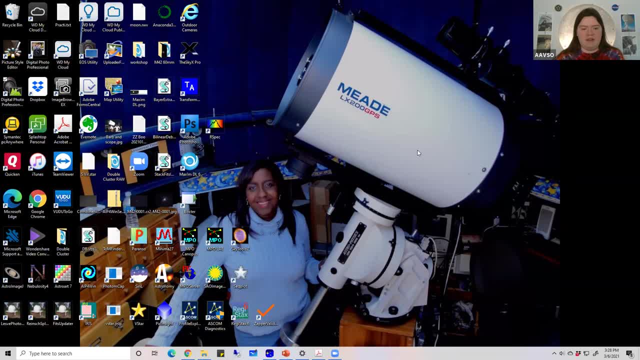 if you had a choice between using a monochrome CCD and a DSLR for photometry, which one would you pick, and why? Oh well, I would say 80% of my work is with my- my cooled CCD camera, And the big reason is one: it's cooled. 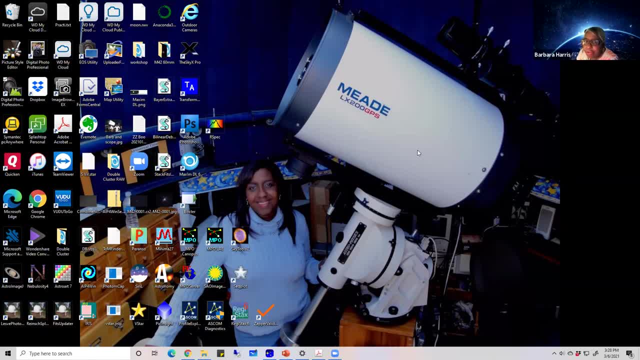 Two, it's a lot more sensitive, So I can- I can get a lot more fainter targets with the monochrome CCD camera than a DSLR, But for me the advantage of the DSLR was to go after those targets that were hard to do with a 16 inch telescope and a very sensitive 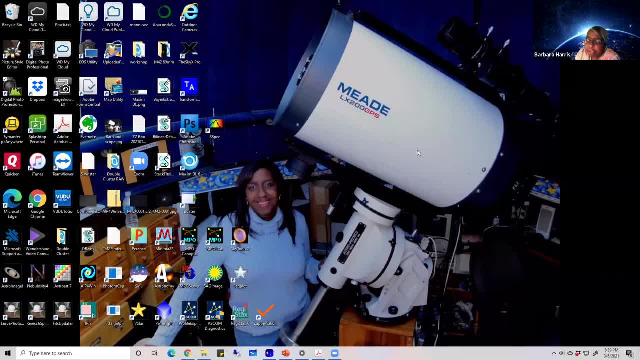 DSLR camera. Like like I said when I started, or the reason I wanted to do DSLR photometry is I wanted to track that Nova, which got to fourth magnitude, trying to do photometry on a fourth magnitude star in a 16 inch telescope with a sensitive DSLR. 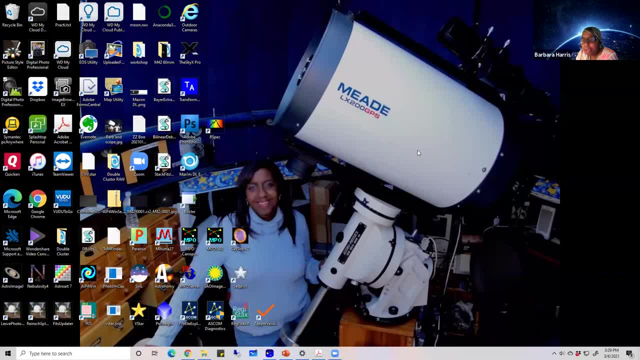 Like even one second with that would saturate the star And, like I said, if your exposures are too short then you run into inaccurate photometry because of scintillation. So you can't go too low as far as exposure. So so the reason I got into DSLR photometry for me is to be able 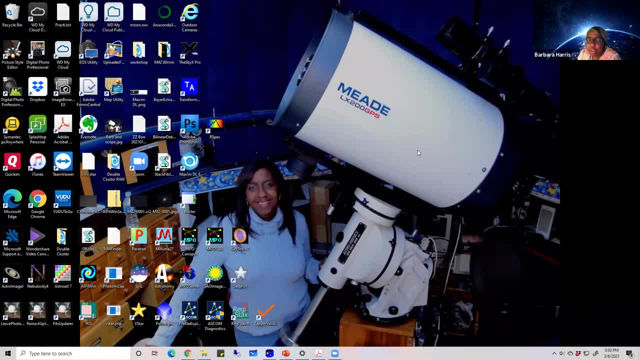 to capture those bright stars and do photometry on those bright stars that were basically overwhelming my big telescope. Thank you All right. one more question about cameras and filters comes from Leonard M Gray and he asked: can you use a photometric filter with a color? 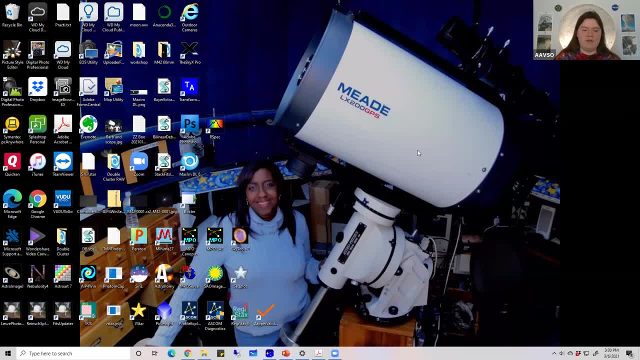 DSLR, for example, a visual filter? And if so, will you still need to debayer the image? I'm not sure that you should do that, Because it gets complicated, because you there's no way of taking out the green filter. you know of the of the bare filter array. 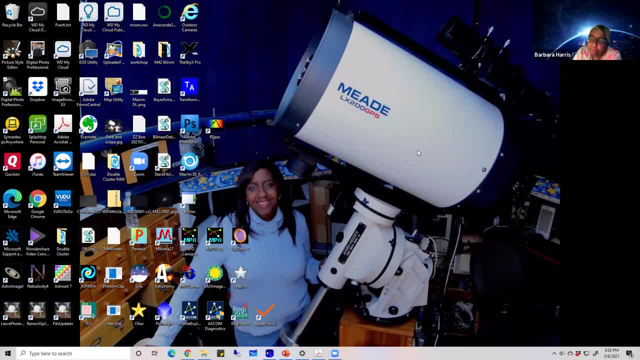 So having the combination of a green filter and a V photometric filter is difficult, Because the only way you could do that is to be able to take away all the color of the bare filter array And and just have the light from this photometric filter. 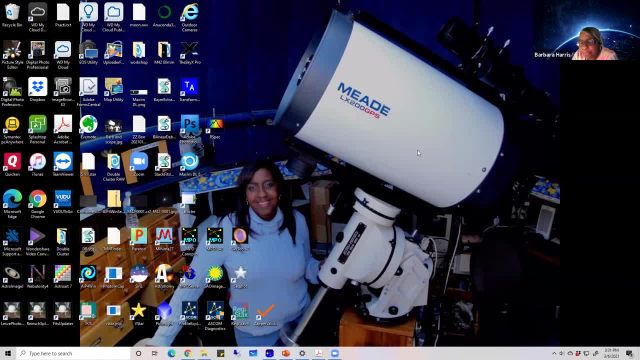 And I'm not sure how you can do that. Thank you All right. So now I think we had a couple questions about tracking, like this one from Alva couch, who has asked: is equatorial tracking required or will alt azimuth tracking do? Any tracking is fine as long as it tracks your star, and it it's. 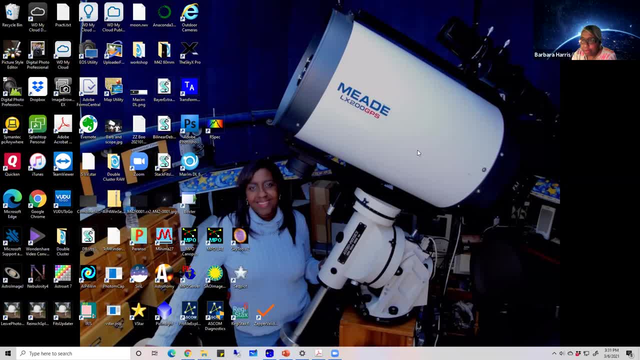 maintaining the star as a nice brown star. So any tracking, Okay, Thanks, I would like to add on that a little bit myself. So field rotation with alt azimuth tracking: Do you know about how long of an exposure you're looking at before? 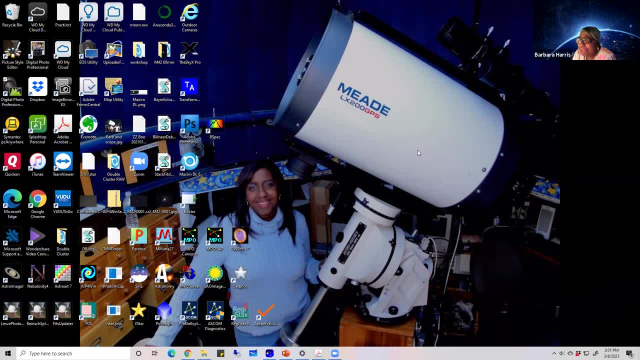 that becomes an issue with your science images. I'm not sure because I always use equatorial German, equatorial mount, So I can't say but but my guess, like for me, like a 30-second image, I'm getting down to about 8.5, 9 magnitude with my 85 millimeter camera. 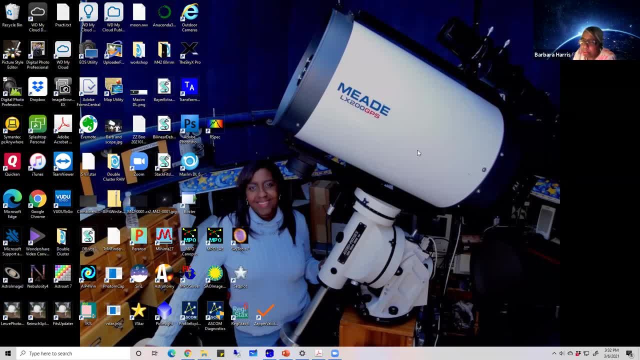 So I could imagine an exposure that short. You're not really concerned with field rotation. Thank you, Let's see. There was another question about Tracking down here. Well, I don't see it, But I remember what the question was. 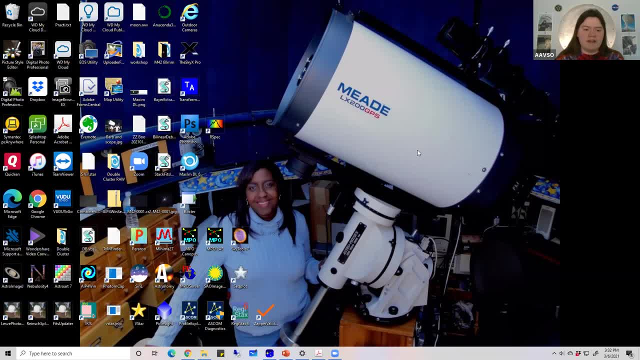 It was about a barn door tracker, And is that a good choice? And also about Dean. have any idea how many a VSO observers are using just the tripod, No tracking? Then I'm not sure and, like I said, it depends on the target. 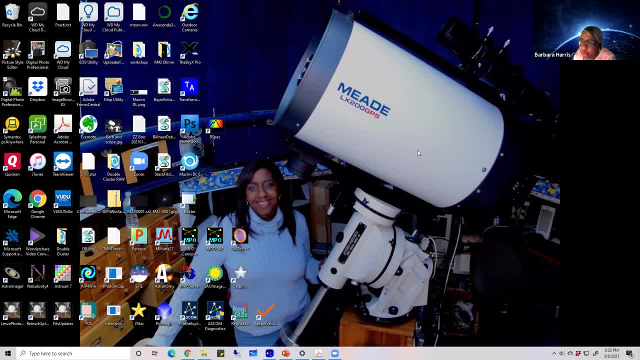 Like, if you're doing Epsilon or Reggie or Beetlejuice, That can easily be done with the tripod and like: even though I have like a and I opt on guide Guider Pro, It's a lot easier to just plop the tripod out there because I'm doing 10 second exposures. 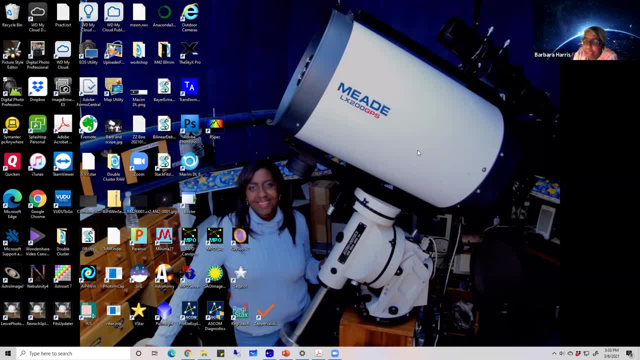 So it's real simple to set up and there are a lot of targets out there that are that are bright like that that you can do photometry on. Thank you, So we have some questions here that are somewhat related about doing photometry across the frame of the camera. 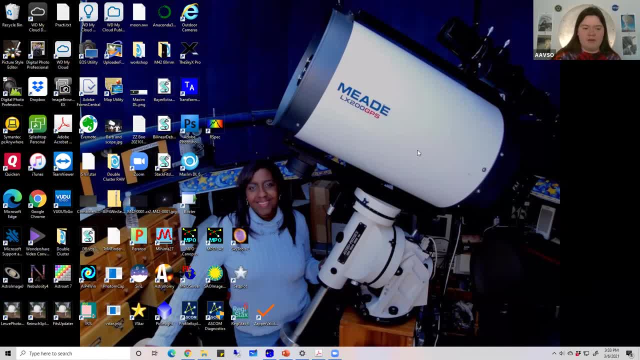 Like this one from Norman Gray, who would like to know if there's any software to automate the photometry extraction across a full image. Yes, actually, I'm like, if you're doing AIP For Windows, AIP for when once, like I today, I was working on images of alcohol. that I did from Wednesday night and there were 197 images. 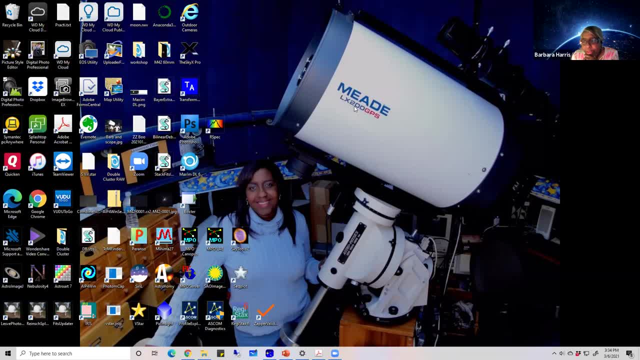 So you don't want to go through 197 images clicking on the variable identifying the comp stars in every image. So most of the software will automate that, Like once you select your first image, what the variable star is and what the comp stars to use. 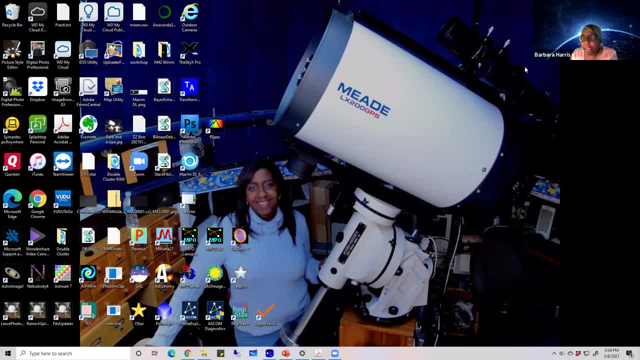 the software basically does that automatically. it goes through that whole list of 197 images and it identifies the variable in the image and the comp stars in the image. So most of the software will automate that. You just have to identify it in your first the. 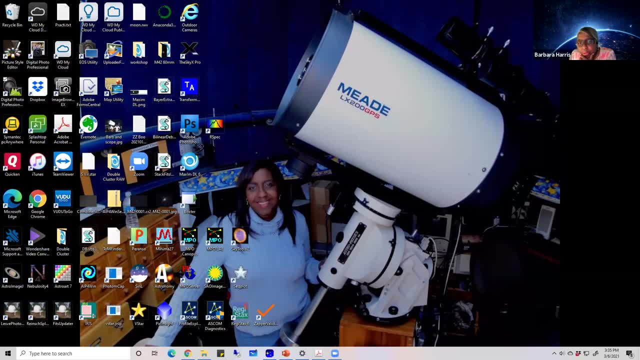 the variable and the comp star in your first image. So the photometry is automated, where you're not going through a whole list of all of your images identifying each, each of the variable and comp stars And for other things. as far as automation, like I said, Pixinsight and Serol will. 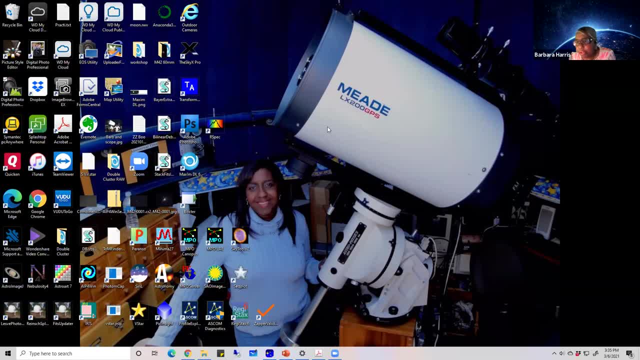 will debayer and extract the green channel From all of your image images. So that's automated with with a script in in both of those programs. So so, yes, almost all of the software. these things can be automated. Very nice, Okay. 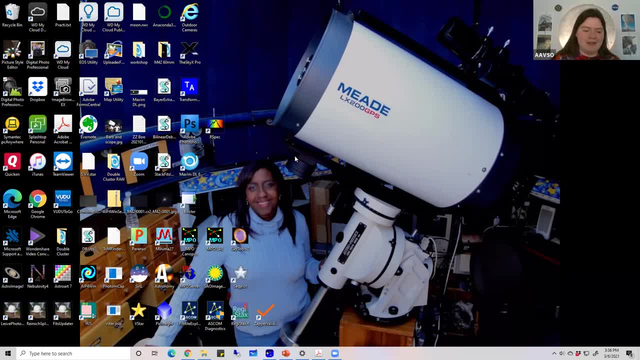 And we just had a thank you come in from Norman Gray, So that will save them a lot of time. So we have a question here That asked, yes, from Cameron McEwing. He asked: do you have to take care with the differences in atmospheric extinction across a wide field of view? 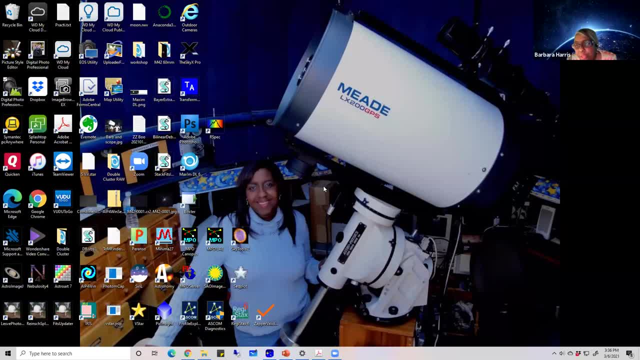 If so, how do you handle that? That that can be a problem with a lens, because with the lens you have a larger field of view and that's why, technically, with the lens, I tried to to select comp stars That as close as possible to my. 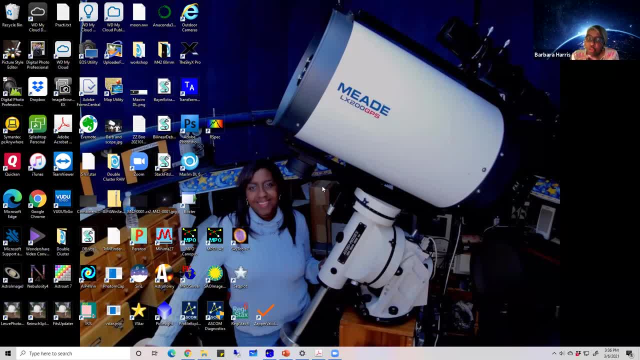 To my variable star, If you can transform Your image, your variable star photometry, from tricolor to photometric. If you're going to use that spreadsheet that I talked to you about, it also takes into account Atmospheric Extinction because of the large field of view. 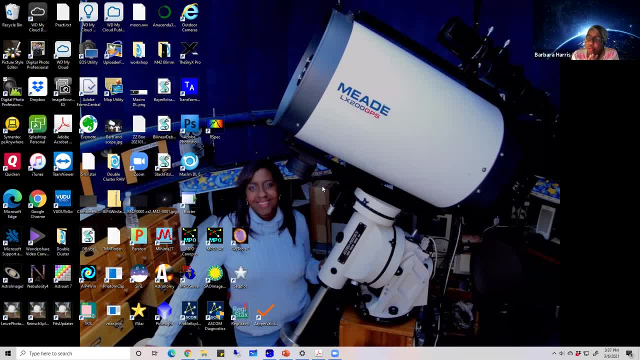 But if you're just using doing photometry on the, the tricolor image, then no, you're not really taking into account that extinction, that that is involved over a wide field of view. Thank you. So we have a question here from Gary Shaw. 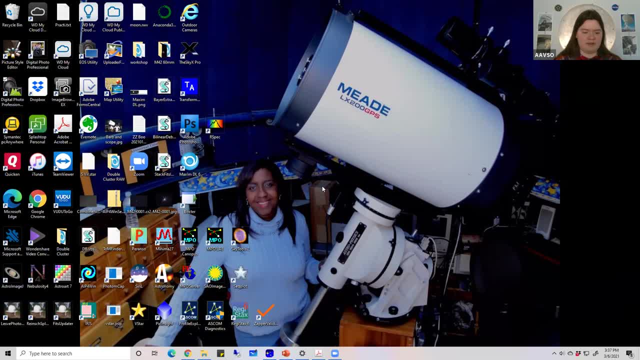 That is somewhat related and it's similar to a question That was asked earlier, but I think different enough to ask: Is there an altitude above the horizon at which scintillation becomes not much of an issue Theoretically? the higher you go, the less of a problem. 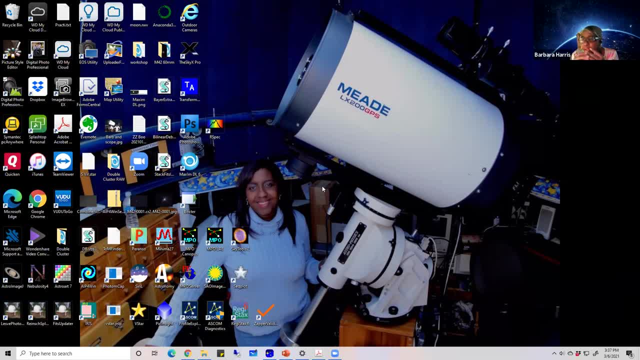 It should be but but theoretically, the shorter the exposure, It's always going to be an issue. So try to avoid it at all altitude. Try to Avoid those short exposures. Thank you, And let's see We've got a question here from Ralph wrong. 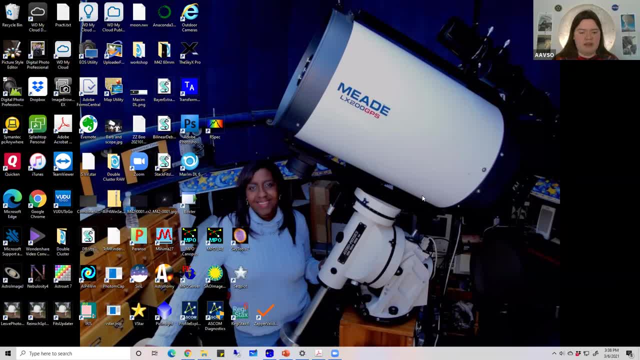 Who asks: is there a standard field of stars that is, that are bright enough for DSLR? is to calculate transformation coefficients That I haven't put a lot of effort in into exploring, Because one: if I transform, I use the, the Excel worksheet to transform, because 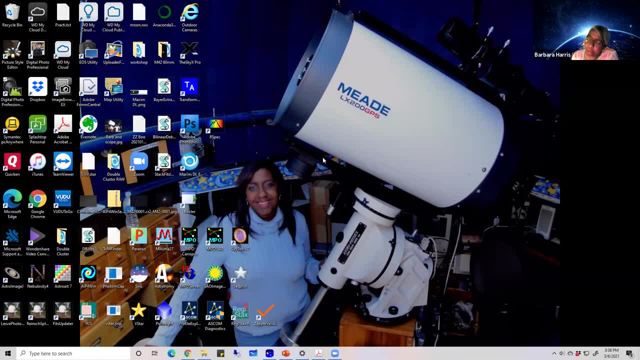 At least for the CCD field, for obtaining transformation coefficients. It's going to be really hard with a DSLR because The pixel scale that you're using with the with your DSLR, the stars are going to be very, very close together, Like for my DSLR. 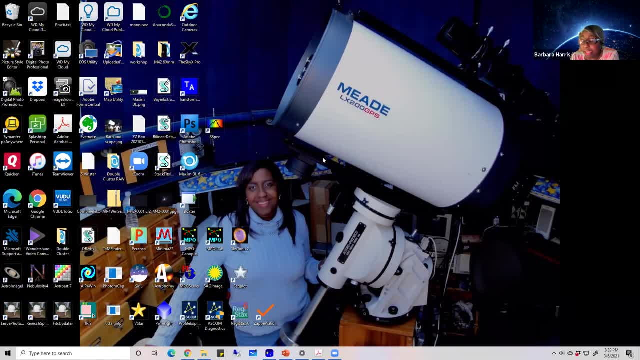 I usually use m67. I mean for my CCD. I use m67 to do my transformation coefficients. Trying to use that cluster for obtaining DSLR photometry is going to be difficult because the stars are just going to be too close together and It is going to be almost impossible to try to do. 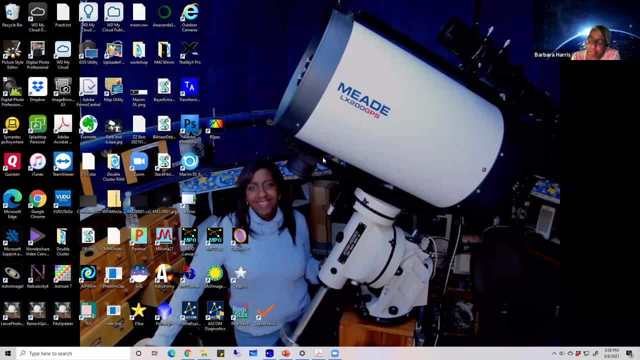 Photometry on the stars in that cluster. I haven't explored any other bright clusters with you know the stars are far enough apart to to do transformation. When I do transformation, I use usually use the the Excel spreadsheet method. Thank you. 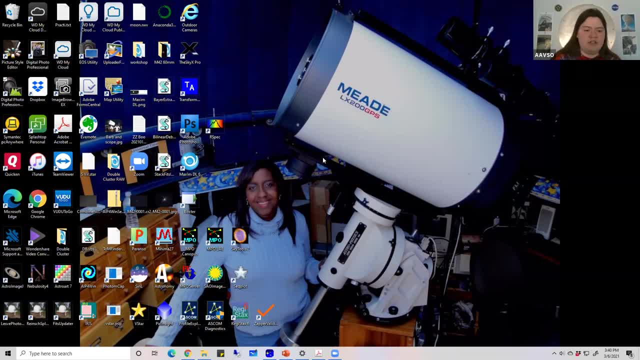 Relatedly to that about stars being too close together, We have a question here from Corey officials Who has asked: when you defocus the image, can another star near your target interfere with the measurements and, if so, how can you avoid that? Yes, that's, that's one of the problems with defocusing, and especially if your target is somewhere near the Milky Way where there is a crowded field. 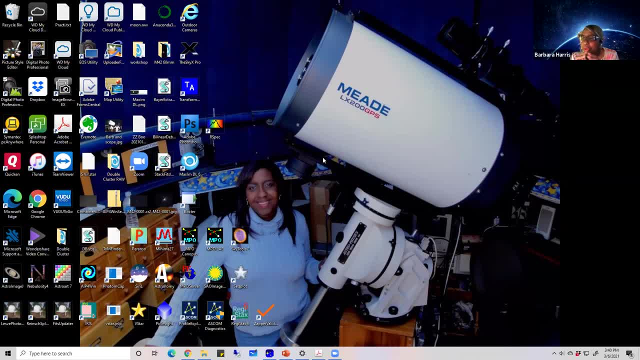 If you defocus too much, you're you're just going to run into other stars and it's going to be almost impossible to do photometry. So one is, try to avoid a very crowded field and two, if the field is a little crowded, just tried to defocus just enough, that where it's adequate, like eight pixels, and I've even gone a little bit less than that, where it's spread out over, like six pixels. 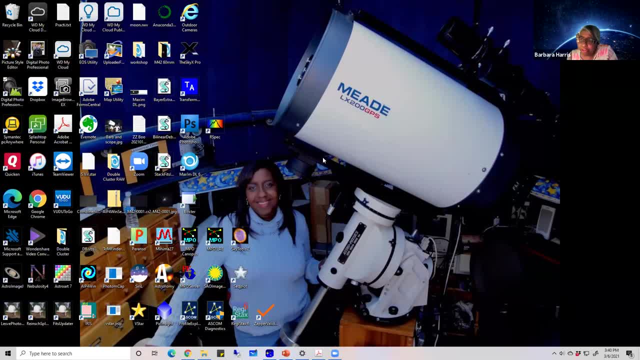 So you just minimize the amount of defocus and just try to stay away from fields that are very crowded, Because it, like You know, like he said, the problem is, if there's a lot of stars, the stars are going to start running into each other If you defocus too much. 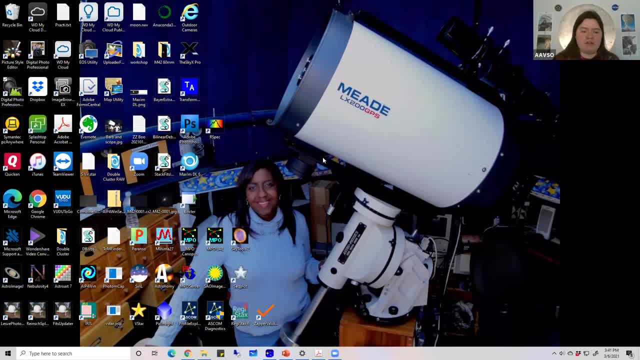 Right, Thank you. So we have another question here that's related to the focusing, from Jamie Jenkins, who has asked: is the point of covering so many pixels when defocusing to cover several green pixels, since they're separated by the bear pattern? Well, well, technically, 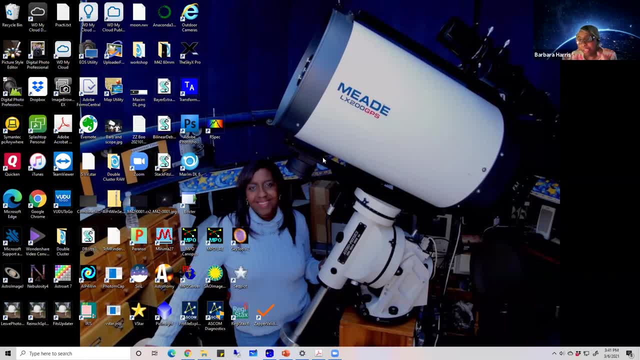 You use it over all of the color filters in case you start to, if you want to use data from those other colors also. but but for for adequate samples It needs to go over over several pixels. It's not like a CCD camera where Basically you you want your star to be spread out over about two pixels. 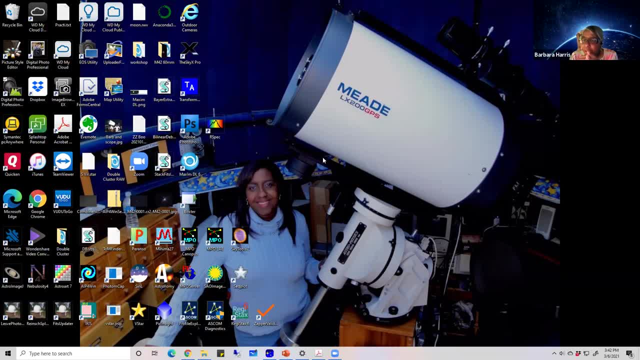 But for DSLR, since, Since you have several Pixels making up a particular color, It's got to be spread out enough to be adequately sample. Thank you, Good answer. Okay, Now, I think we had some questions here that were about Some more a VSO specific things, for instance this question from Patrick Cavanaugh: 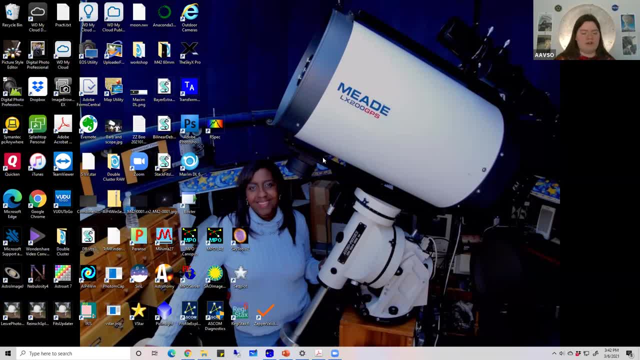 Who asked: Would you please go over again the process of going from the report that the photometry gives us to submitting the data to the a VSO? He says that the a VSO web page looks changed from the last time he used it and he's not sure what type of files to use. 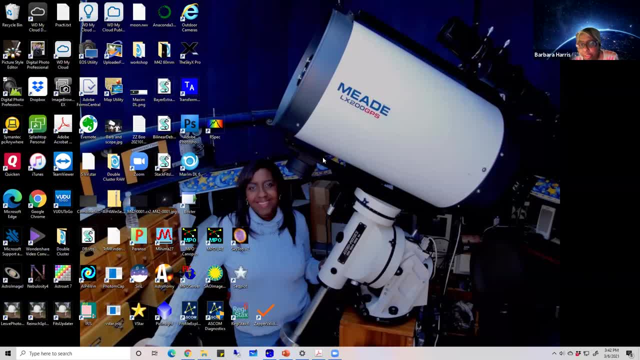 Well, most of the software that I talked about. Like, if you go to the a VSO website and and search extended Format file- Most of The photometry software- they will generate that file And basically there are, I think, about 15 different. 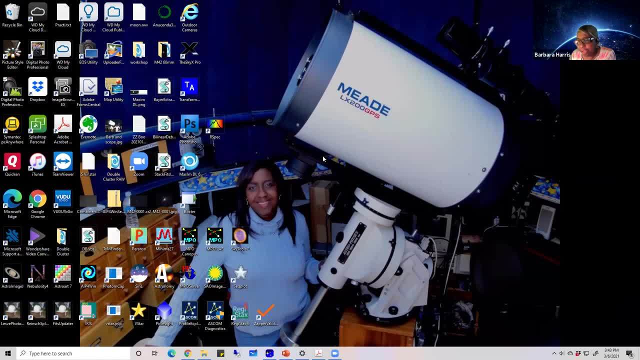 Items and it's the name of the star, The Julian date of the star, the magnitude of the star. The error That you get from The photometry, Whether it's transformed or not. The identification of the comp star and the comp star magnitude. identification of the check star and check star magnitude. the air mass. 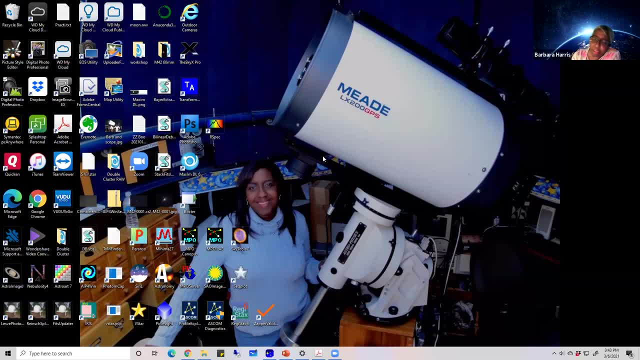 There's a comment section, So all of these are necessary. that has to be submitted and it can be submitted and a file which most a lot of these software programs will generate, Or there is When you click on the submit data on the front page of the a VSO website. 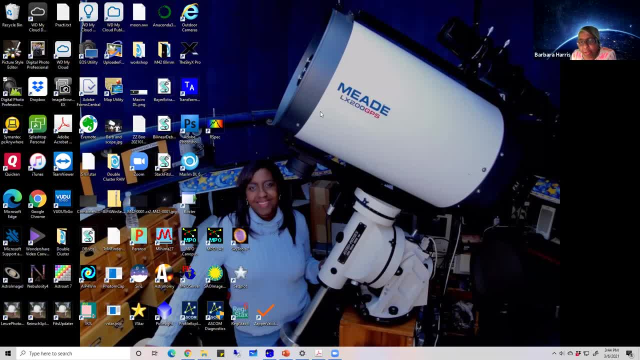 If you, when you go to submit data, there's an option to to submit data on an individual star, where it'll take you to a form where you fill in all of that information, Like you fill in the name of the star, you fill in what time your. 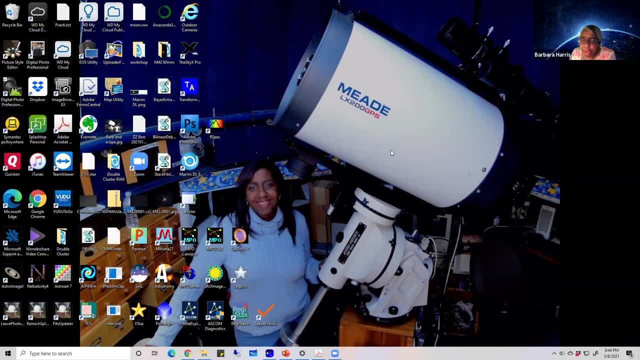 Image was taken And you put the magnitude, that that you've measured and the error, And so you can fill in all of that on a form, or there's an option: instead of Individual Submitting individual data is to submit a file and you just click on submit a file and you go to where that file is located on your what, on your computer to submit it. 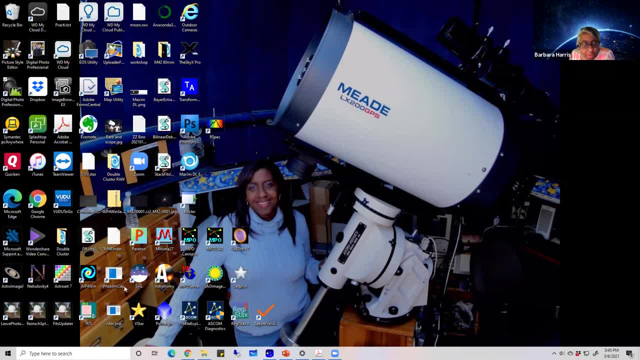 But, like Most of the photometry programs that I've talked about, will create it and a VSO formatted file of the photometry that been measured. Thank you, Let's see We also have a question here, or actually it's a comment from Andrew covex, who has said: please consider creating a DSL, our section, or some campaigns like epsilon or a key. 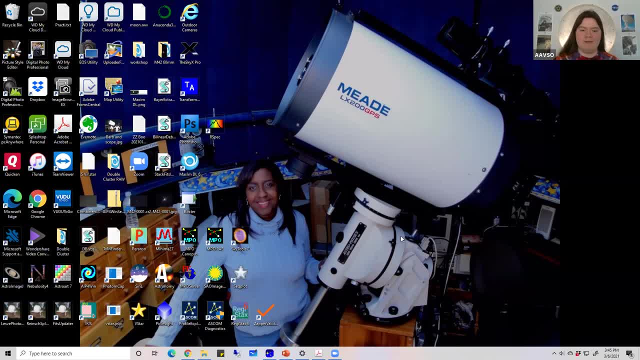 Campaign that used to be active many years ago, So we will take that into consideration. Here we have a question from Michael freeberg, and I think there may have been some other people asking to- who asked: what files do you archive in case you need to go back and look at your data? Do you only save the calibrated images that you work with? you save the Ross? 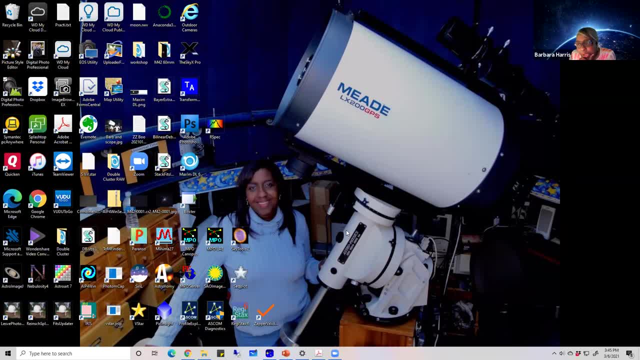 You know, I I fortunately save everything. I saved the raw image Images, I saved my calibrated images, I saved my extracted color images. So it it can run into a lot of A lot of Memory, but I saved everything, from the wrong to the calibration files. I save it all. 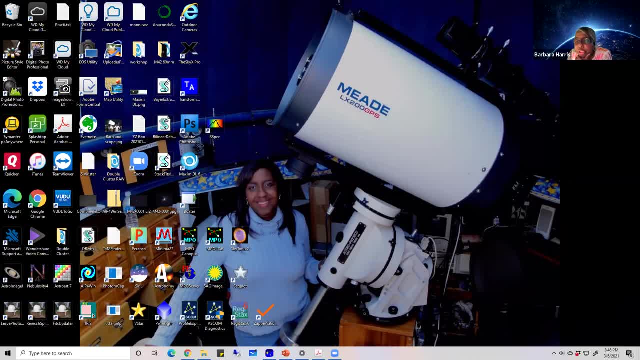 And someone above that, as are you doing photometry on the raw or the fixed images? Know, your, Your photometry Is done on a fixed image And one thing I should mention is that when I say that Your, Your star image, should Be spread out over so many pixels, When you measure that, you measure it on a raw image before you extract any color information from it, So, right out of the camera, raw image is where you measure. 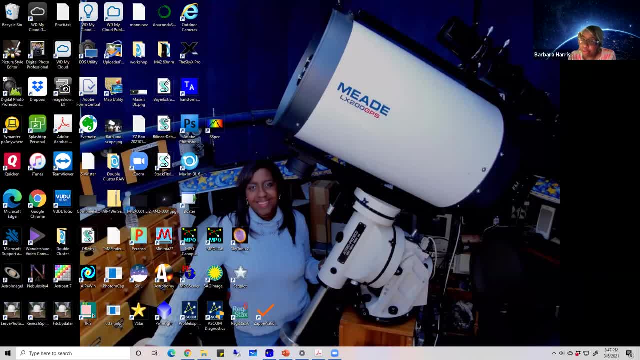 Your signal to noise ratio to make sure it's not saturated, and and you measure your full width, half max of the star, to make sure it's right over several pixels. You do all of that, you. you measure that in the raw image. But when you're doing photometry your photometry is on a fixed image that's been extracted from a calibrated raw image. 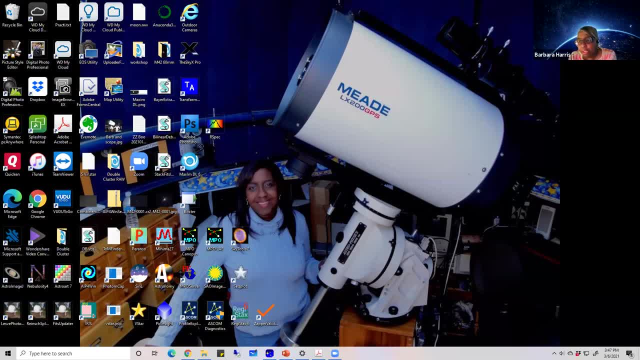 And and either debayered or Or just extracting the green channel from the calibrated raw image. So yeah, you're doing it on a fixed image, your photometry, not on the wrong Image. Thank you, I think we had a couple questions here about the mentorship program. 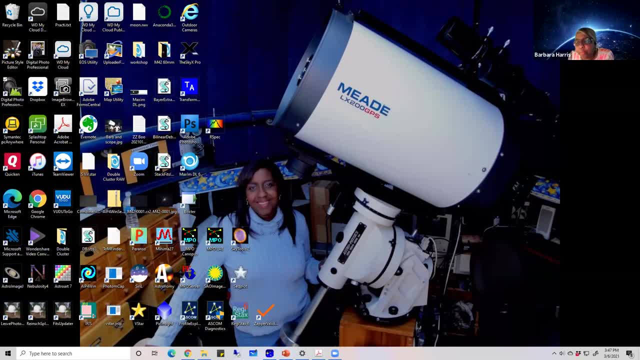 So I see one here. Do you think an external power supply for DSLR will provide a better linear response? And as long as your battery is is adequate And fine and not dying, It shouldn't have anything to do with the linear response. It's just that if you're imaging for quite a while, you may want to have an external power supply, like two nights ago when I was doing. 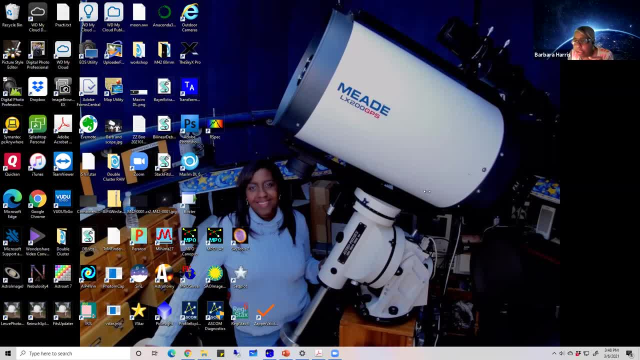 Epsilon, not epsilon Algol beta percii. It was about three and a half hours of data So that I wasn't relying just on my battery. I had an AC adapter for the DSLR photometry and doing that, But usually I just use a battery, because if I'm only just doing a few images, I just use the battery of the camera and it. 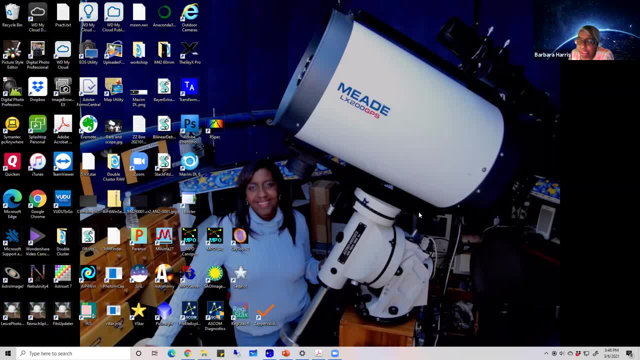 It's not going to change the linear response whether I use external power supplier or the battery of the camera. Thank you. Our next question From Edward real, who has said that he's interested in occultations and would like to know if the mentor program is only for variable stars or if he can turn to that to learn about how to record eclipses and occultations. 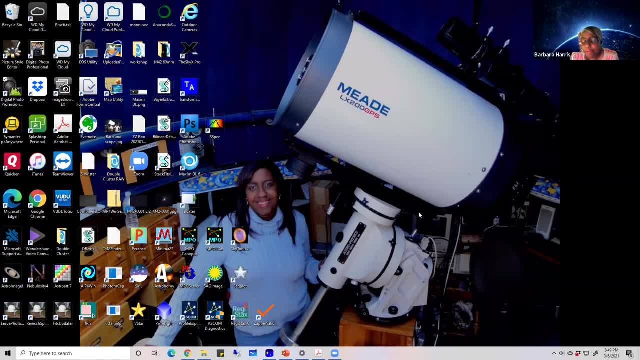 Oh, I think it's mainly for For variable stars. I have done occultations. I haven't done one in a few years. One organization I would recommend Turning to for that would be iota International Occultation Occultation Organization. they. 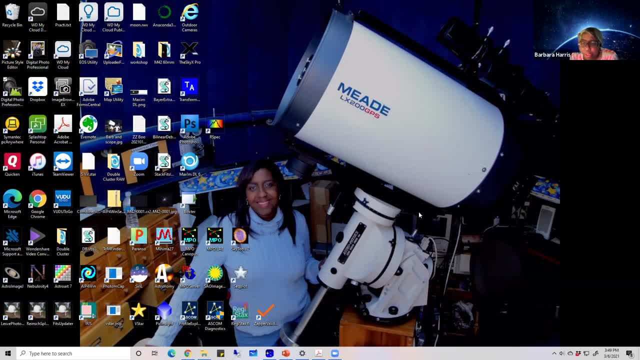 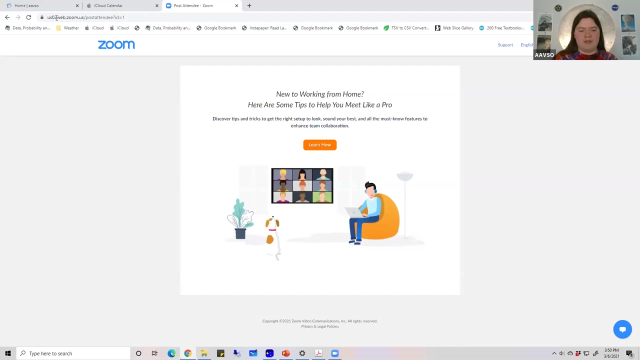 You can get mentoring through there, But I don't think a VSO has any mentoring for that. Yeah, we had one other Question about The mentorship program, which was someone asking about If they can come to the a VSO mentorship program to find a mentor for their PhD. 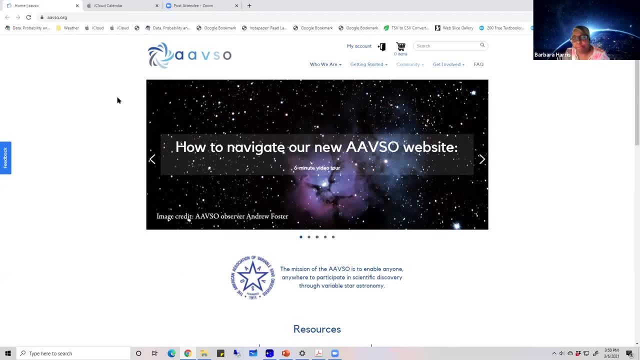 That you will have to consult the head of the, The mentoring program, for that. that I'm not sure. Thank you, All right, so back to some technical questions. William Daniel has asked, after collecting the images, What's your workflow for the post processing and analysis? And I think that was sort of the presentation. So if you would like to just summarize real quick, 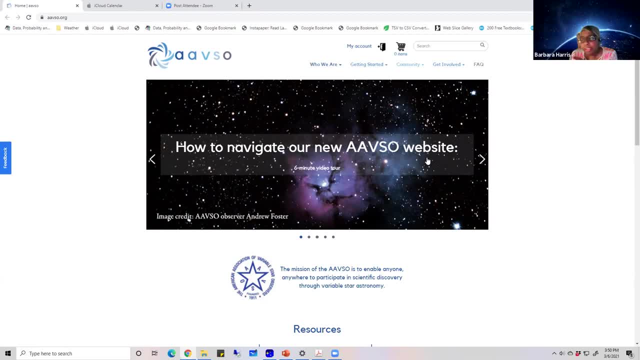 The recording will be available later for review. Okay, so, after I collect my images- and I reviewed them to make sure that they're not saturated and that there's a good signal to noise- I calibrate my image with With dark, flat and biased frames. after I calibrate them, 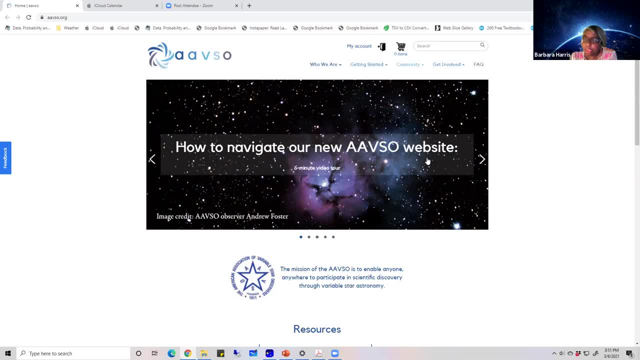 Then what I'm doing now is I'm doing a by linear, the mosaicing Of the of the calibrated images, and, after they're debarred, I'm taking that color image and I'm Splitting the Channels into red, green and blue, and I'm taking the green images and I'm doing photometry on those. 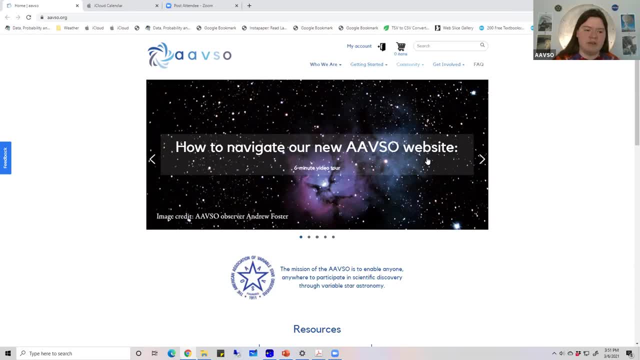 Thank you. We have a question here from Dino, your sink. I'm sorry I'm not, if I mispronounce that- Who would like to know how Big of an aperture radius Would you recommend that you use when you're measuring the instrumental magnitude? 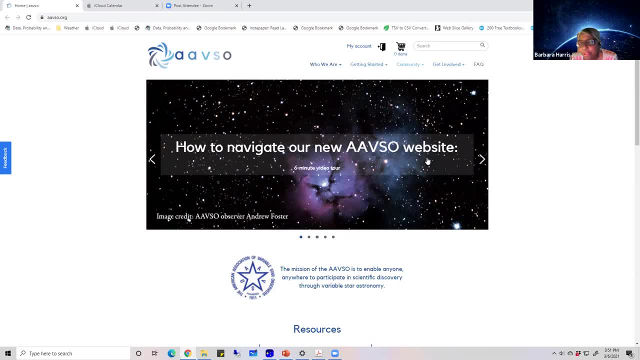 It depends on The size of your star. Usually The recommendation is- and it will if you go over the a VSO CCD manual, It has it there- also- To use a measuring aperture of about one at least 1.5 times Your pixel, your pixel. 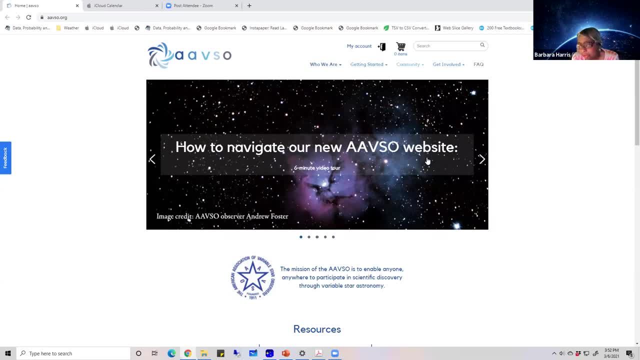 Diameter, radius actually of your variable star and your comp stars. So you want to choose an aperture That's about one and a half times The size of Of your variable star. Thank you, Let's see. Someone asked about what. what's one, two, three and four in maximum? 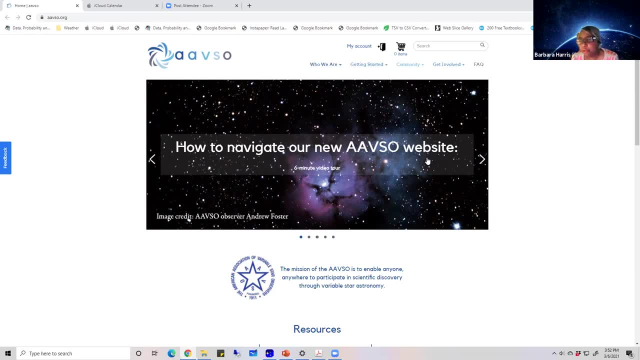 And I mentioned that you have to determine that for your camera, like from my camera, The green channel is two and three, red is one and blue is four. So you have to find out the bigger pattern of your camera to determine what's one, two, three and four and maximum. 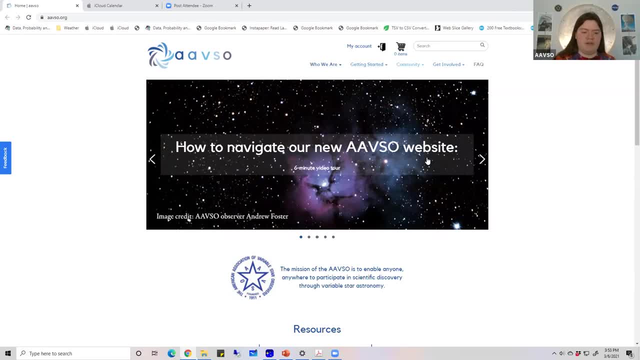 Thank you. Next question is from Gregory the wandless, who has asked: can you use one More than one comp star, and does doing so improve the results? Yes and yes. Sometimes you're you're limited to To just one or two comp stars, because that that's all there is in your field. 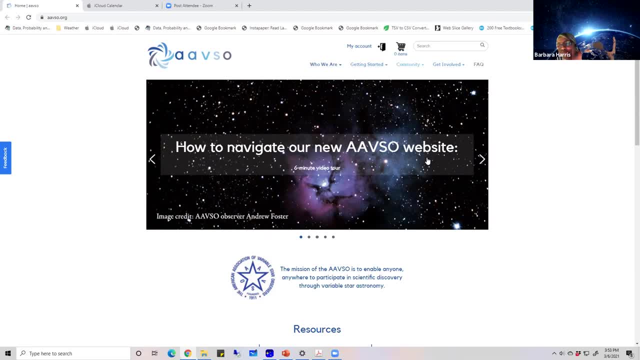 And you can't for comp stars. You can't just look at a Planetarium program and pick out all the stars around your variable field And say: I'll use These because my planetarium program says that this magnitude is, this is the magnitude of that star. 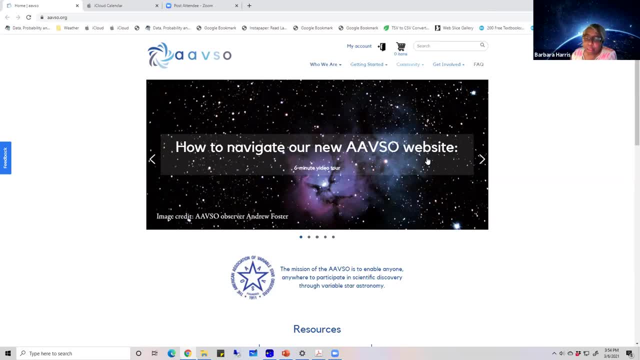 This is the magnitude of that star for every variable star field. AAVSO has selected stars that are adequate for comparison stars for that field of view. like in my slides I pulled up I had a chart for Delta cpi. So what you would do is on the front. 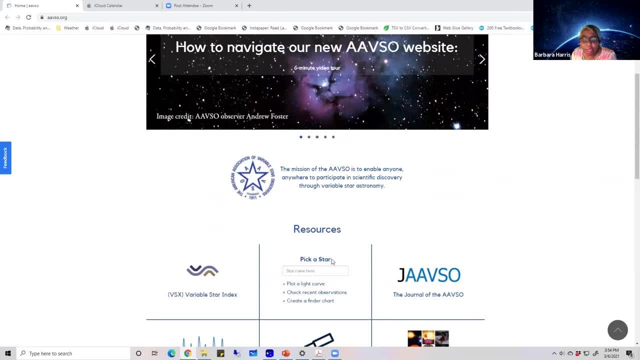 Page of AAVSO, under resources, under pick a star, You would type in the name of the star you're interested in and then you would click on create a finder chart and on the finder chart page It gives you, you put in the name of the star and you put in how big of a field of view that you want. 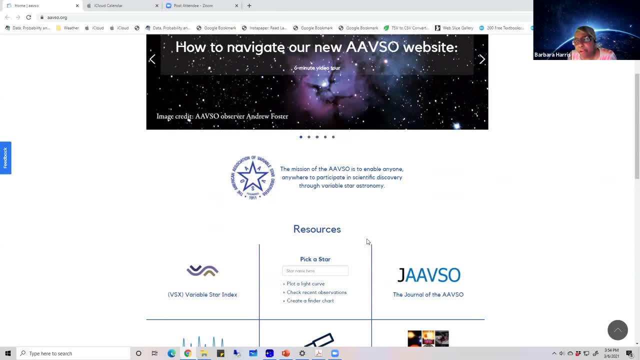 Like for my my 80 millimeter refractor and my Canon 40 D, I usually use a 2.5 Degree field of view Because it's it's somewhere around that. so I put in a hundred and fifty minute field of view for 2.5. 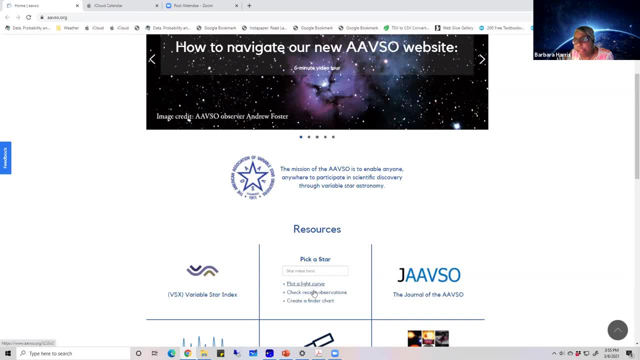 Degrees, and then it asks you for a magnitude limit And so, Like if I'm doing a beetlejuice, you want your comp stars to be, to try to be, within two or three Magnitudes Of your, of your variable stars, And that's why you need such a large field of view for bright variable stars, because you have to find bright comp stars. 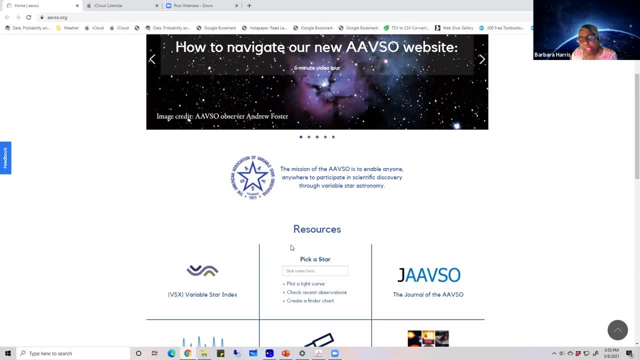 To measure, and so you put in the field of view that you want and you put in the magnitude limit. So, like for our core board, that right now about about 6.5 magnitude, I'll put in a magnitude limit of about nine, eight or nine. 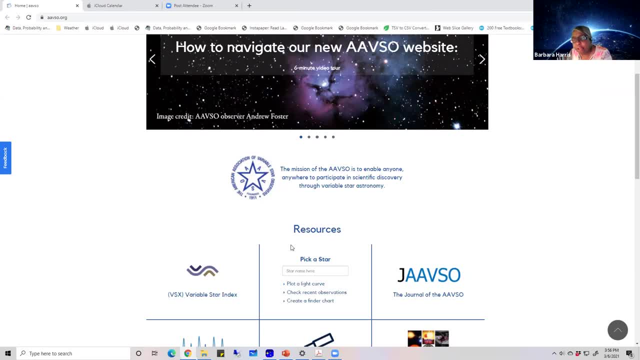 And then it'll it'll print up a chart of that field of view and all the comp stars that are up to that magnitude limit, that surrounding your variable stars, Thank you. So we have a question here from Robert Crumrine, who has said that you mentioned stacking three images for each observation. 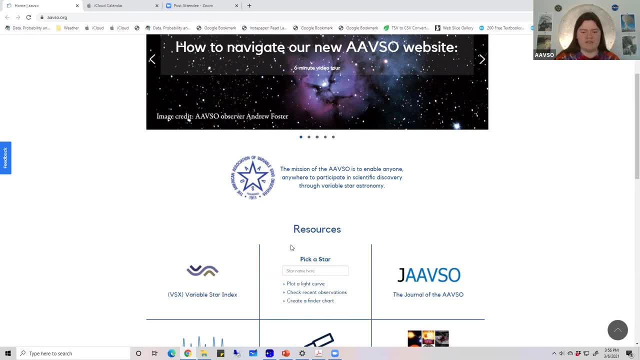 Of Delta Cephei and when you are following a rapidly changing variable such as an eclipsing binary, how many images should you stack for all three? Well, one, I did not stack the images for Delta Cephei. I took three images And I extracted the green channel from each of those three images and I measured the photometry from each image. 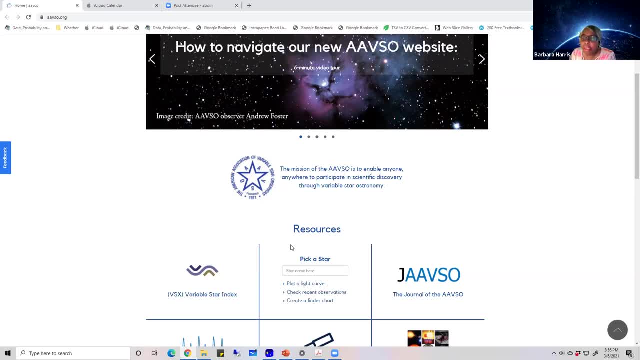 I did photometry on each image. So at the end when I measured the photometry I had photometry of. I had an estimated magnitude from image one and estimated magnitude from image two and an estimated magnitude from image three, And then I average those three magnitudes to come up with an average magnitude. 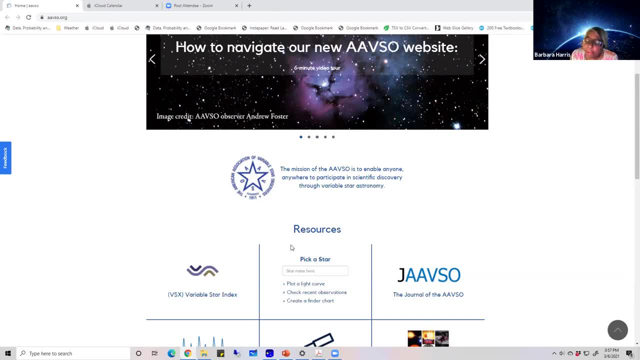 for Delta Cephei. So with with eclipsing binaries, you're doing several hours of a light curve in this rapidly changing. Those are times You don't want to to to stack images. You want to take an individual image and you measure each of those images. 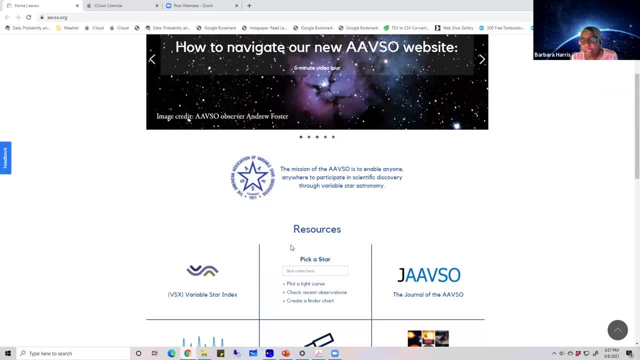 But for the Delta Cephei example that I talked about, I didn't stack the image. I've measured three different images and then average the result And then I I reported my error as the standard deviation of those Three magnitudes. Thank you. 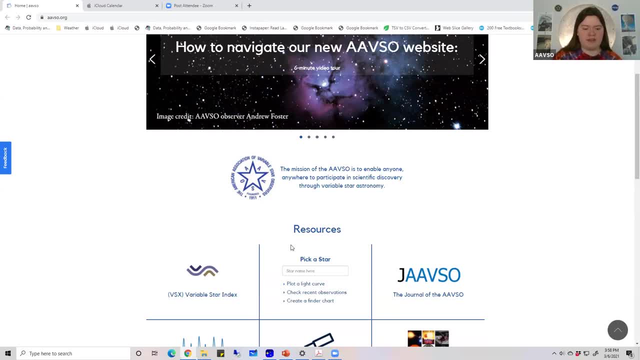 All right. question from Brad Vici, who has asked if you have any thoughts on remote triggering equipment or methods. Actually, like the other night when I did Delta Cephei and not Delta Beta, Persei, algol, Technically it, it kind of ran by itself. 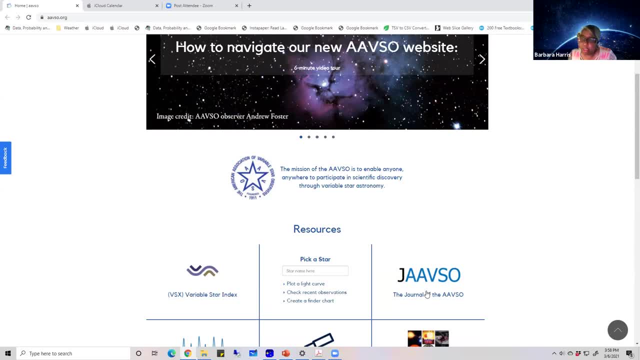 but I do have a remote intervalometer for my Canon camera that that I could be in the house and I could you know pro. I could either program it or I could take images using that for my Canon 40D and my 80 millimeter telescope in the observatory. 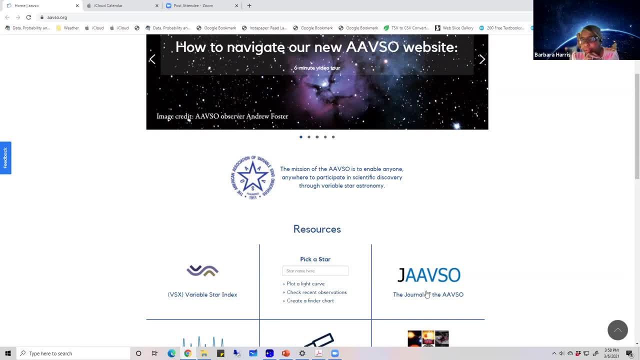 My observatory is all automated. So you know I- it's basically, you know I- control everything from inside the house and it's all automated. So thank you. All right, Like we have a few more technical questions left. 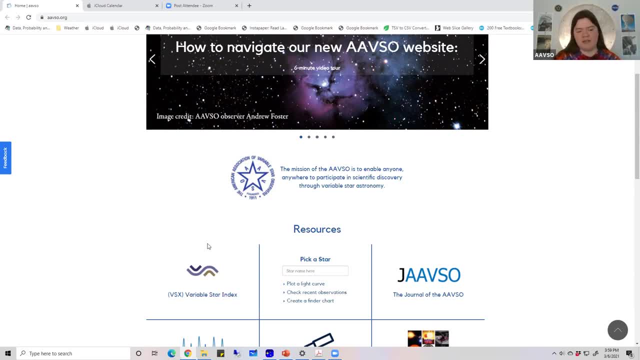 One was someone asking if you have a preference between APS-C or full-frame Size sensors. I use a crop filter. It doesn't matter actually, So whether you use the cropped or full-frame filter. Thank you. We have a question here from Francois Marcoux, who has said first of all: 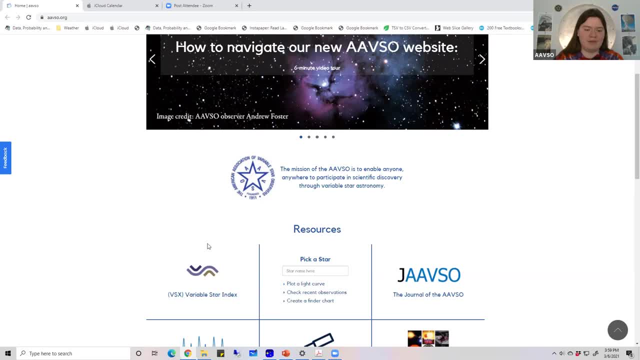 that he enjoyed your presentation and has said that he lives in a light polluted city comparable to New York City And wants to know if it's possible to do decent photometry from there with just modest equipment such as an old 12-bit Canon camera. 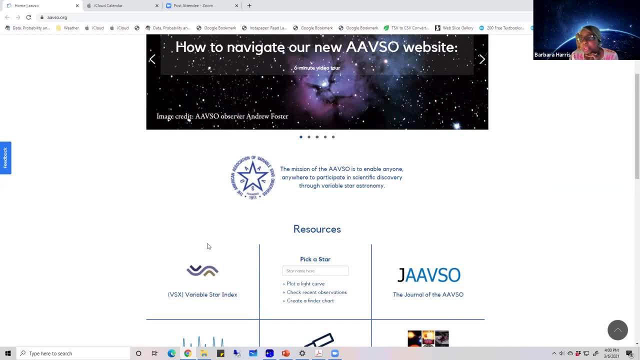 Yeah, it's possible, especially on bright targets. So as long as you can find the star, you can do the photometry. And, like I said, most cameras nowadays are 14-bit camera. but even with the 12-bit camera, 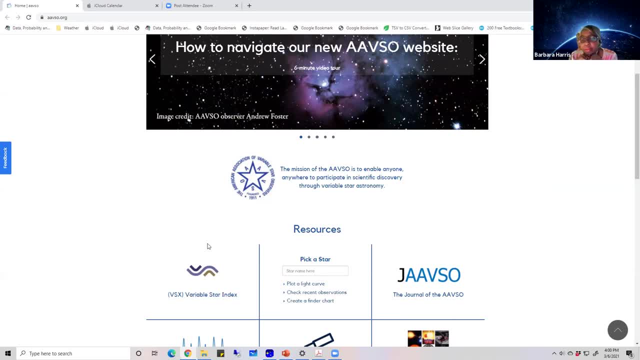 you can do photometry. So yes, it's possible. You just have to choose your target. Great, Thank you, All right. Another location related question came from Bob Neff here, who asked: how many clear nights do you get there in Central Florida? 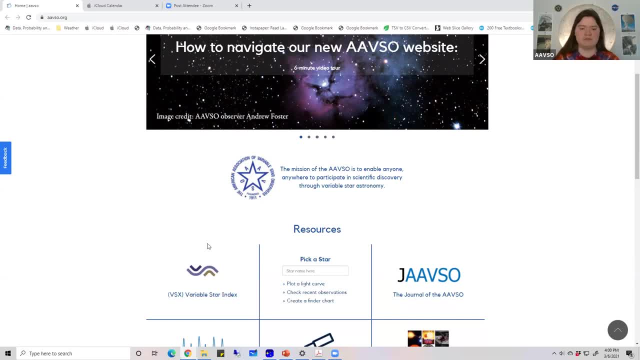 And how often does the weather interfere with your photometry? Let's see, Like, let me. let me look at last year's. One thing I forgot to mention also is take copious notes. I'm a stickler for, like one, I love journaling anyway. 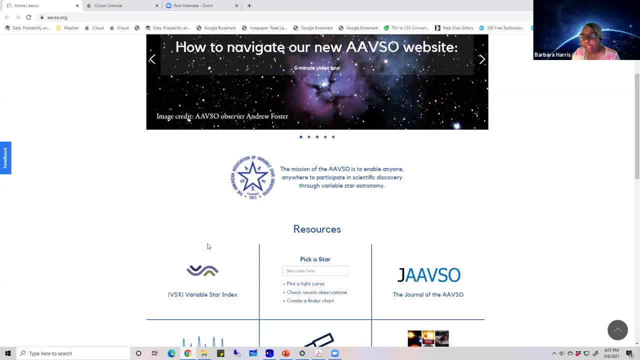 So every night that I'm doing photometry, I take notes. I take. you know what time I started, what the temperature was, humidity, what target I'm. I'm taking images of how long was the exposure, What was the f-stop. 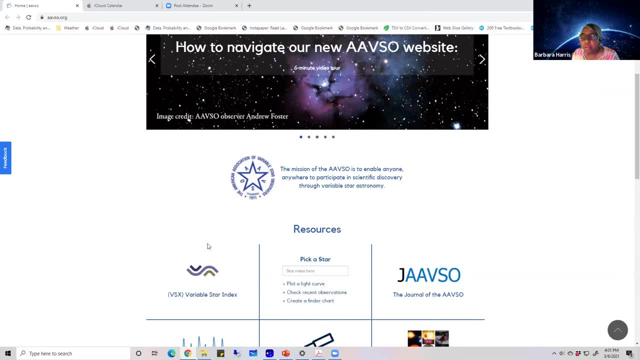 How many images I took. So there, you can't take enough notes. So keep good notes when you're you're doing photometry, because also it's easy for me to go back and say, okay, I when I did that target last month. 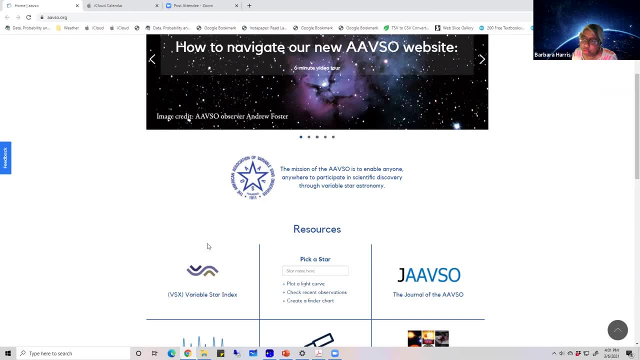 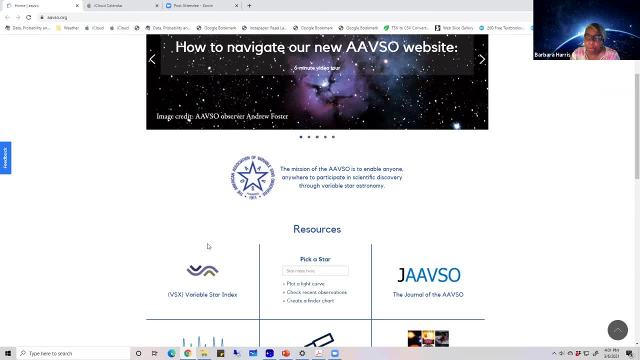 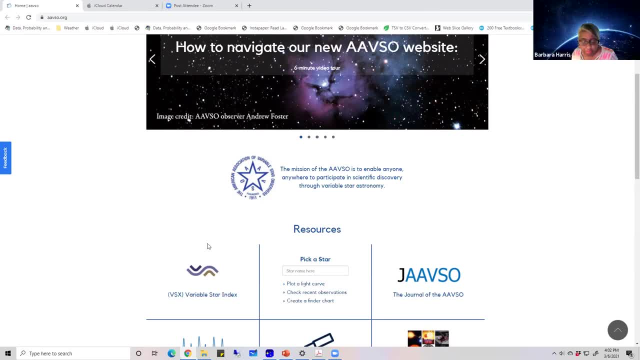 Let's see like let me look at my log for 20.. Like for 2018,, I had 118 nights of data. You know, at least they it was good weather nights. There are times I may not have collected data because I wasn't feeling well. 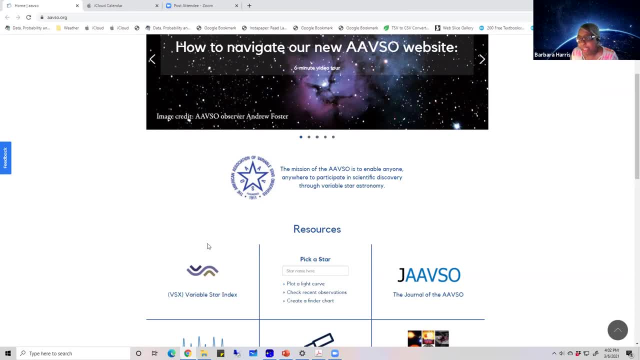 but out of a year I collected data on 118 nights, So at least one-third one-third of of the year I had, I had good enough data to do photometry. Thank you, Okay, So we have a question here from David Marshall. 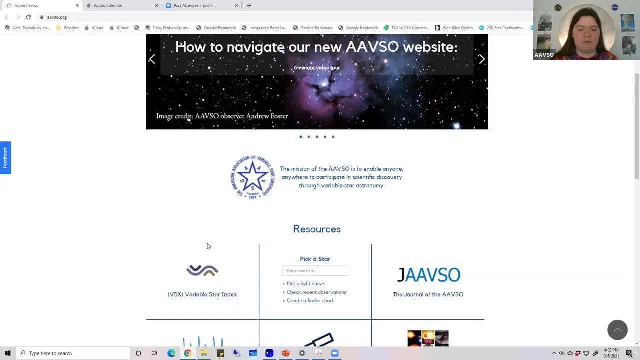 who has asked: in the scenario where a 10-second exposure is too long and will cause the star to saturate, would stacking some shorter exposures be a workaround that would eliminate scintillation? Yes, I'm, I mentioned that, like for Beetlejuice, when it was too bright for 10 seconds. 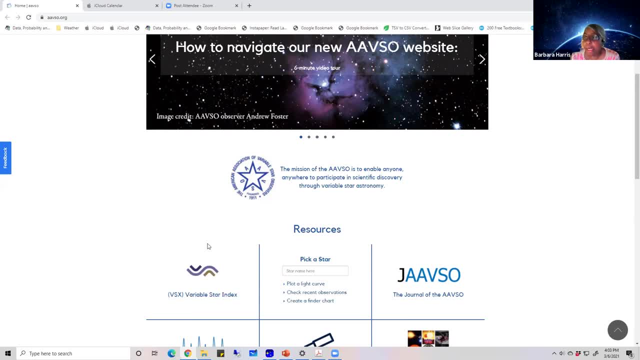 and even going to a lower ISO level and a higher f-stop and 10 seconds was still saturating the star. I would go to like five seconds and then I would take about one minute of five second exposures and stack them and then that would take care of the problem of 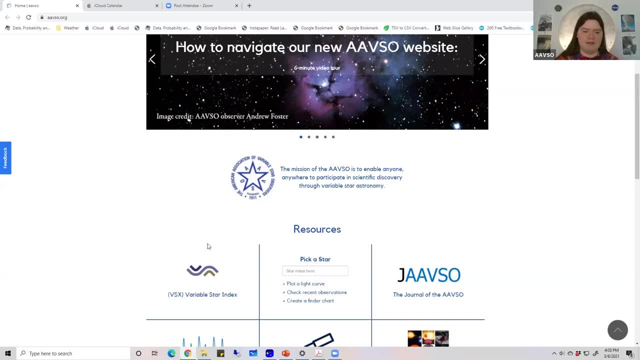 scintillation. Thank you, Gerd. Yes, Yeah, I was. I was just looking at that one from Gerd. Is it necessary to change time to heliocentric time when I transmit data? No, usually when you transmit data. 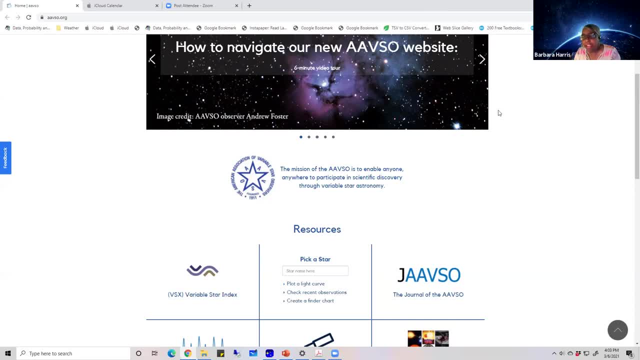 they. they ask for the Julian date. So rarely do I use heliocentric Julian date, but usually you're using the Julian date when you're transmitting your data. Okay, Thank you. Okay, Looks like a technical question just came in from Alva Couch who asked: does a 6 megapixel CMOS camera 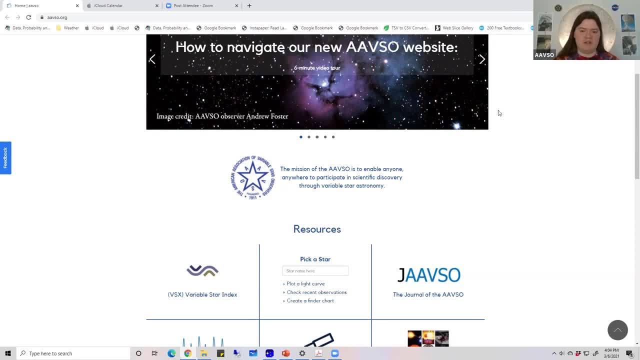 have enough resolution to do photometry. That I'm not sure That. I actually I'm not sure it. It depends on how big of a field of view that's that's giving you. I mean that I really can't answer, Okay. 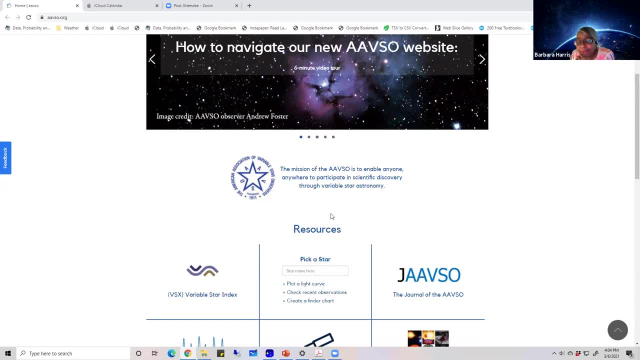 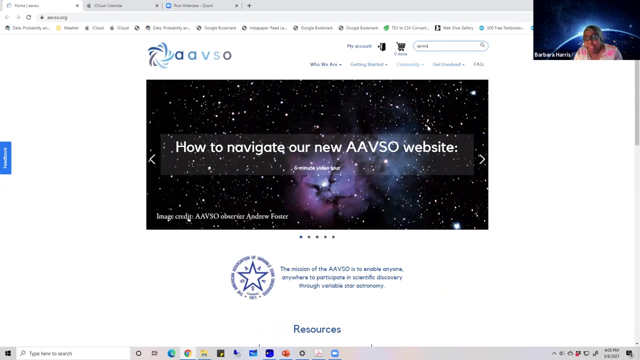 But, but I could imagine that it, that it, it should, you should be able to to get photometry from that size. I don't see why not. Someone asked about the spreadsheet that you can use to transform, And it's somewhere on the AAVSO website. 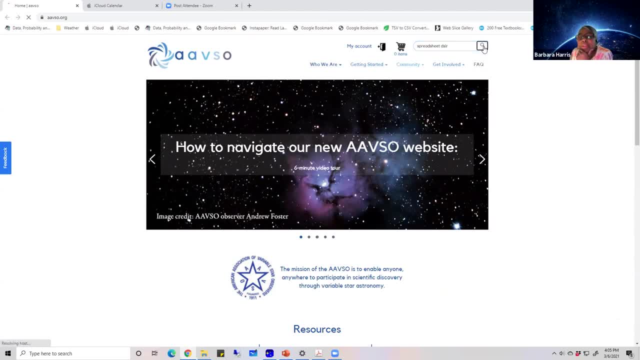 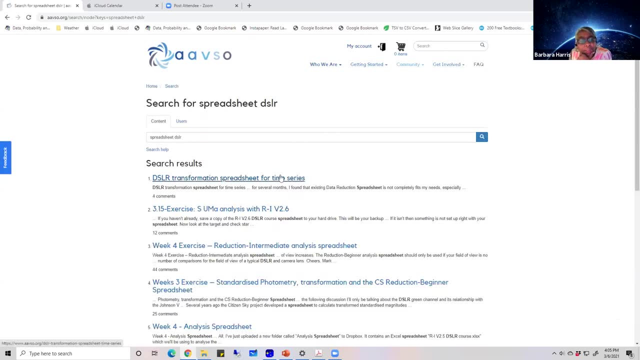 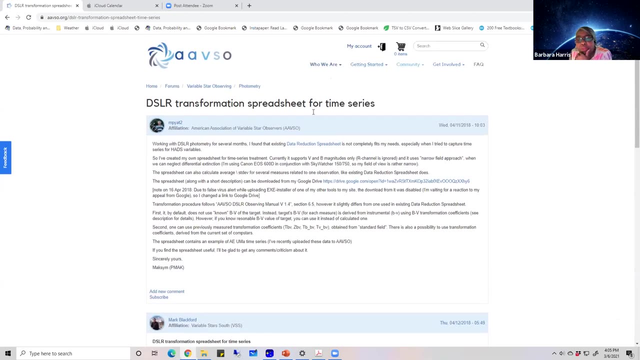 And let me see if I could find where it is. It's probably on the same page as as the DSLR manual. When you find the manual, the spreadsheet is probably on that same page. Perhaps we could include a link to that when we send out the 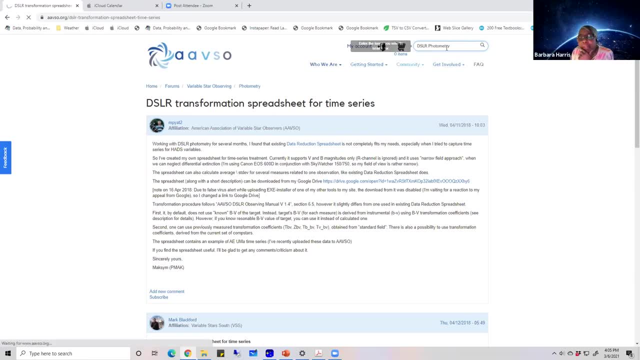 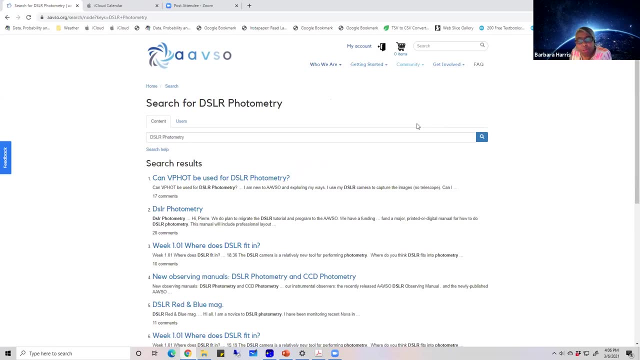 email with your slides in it? Yeah, because I'm not only on on that particular page. Not only does it give you the DSLR manual, but I think the spreadsheet is on that page and it also has instructions for doing photometry and different software packages like AIP. for when? 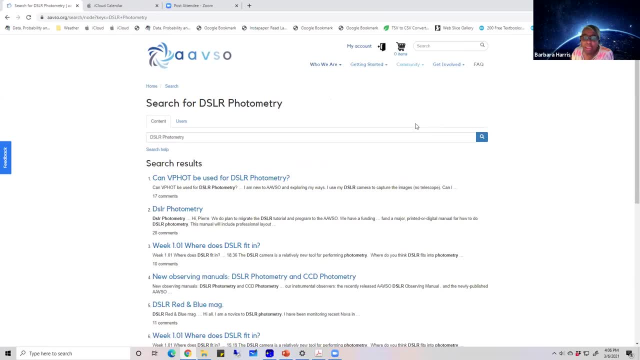 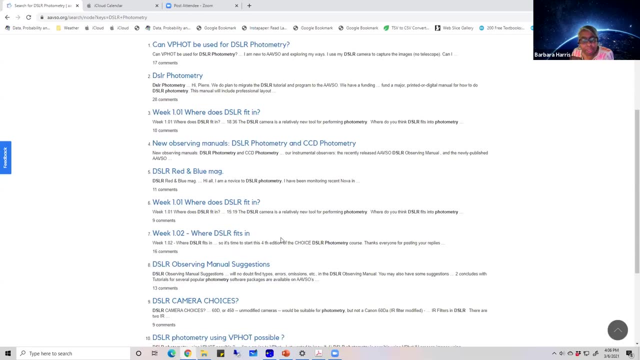 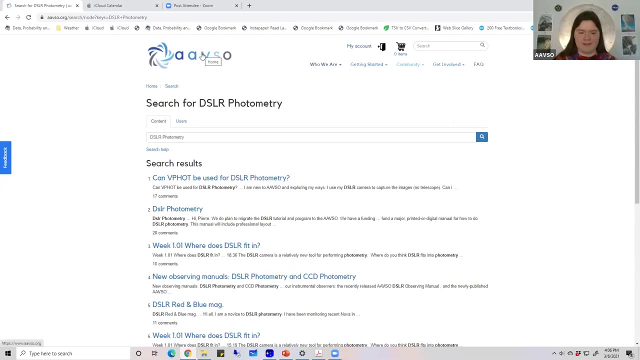 or Iris or Maxim. So if you find that page, I think all of that will be on that same page. So maybe we can provide that link. I think that we can Thank you All right. Jack Stone had asked: can you receive more accurate results when using a plate solver to find the position of the comp stars and science star? 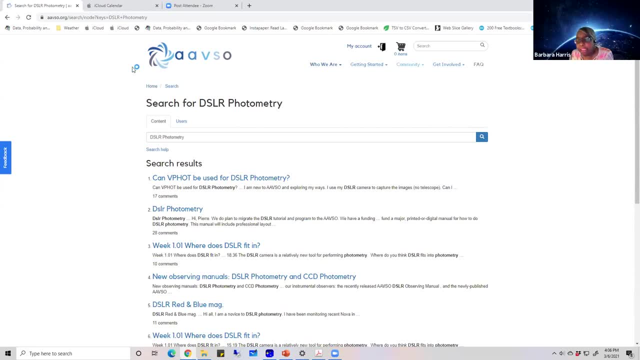 Well, the photometry isn't going to be more accurate, but at least if if you can plate solve the image, you could guarantee that you're getting the correct. you're identifying the correct stars, Like once they're identified, whether the image is plate solved or not. 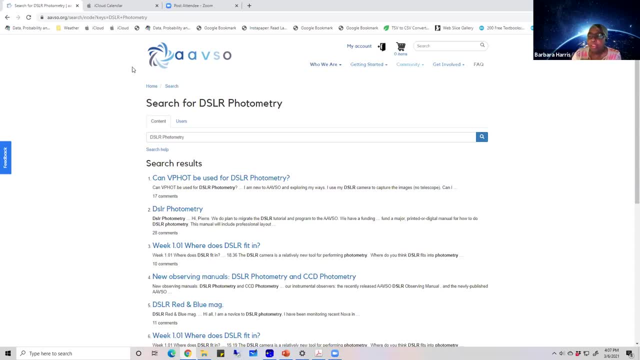 it's not going to help improve the photometry. So the advantage of plate solving is that you know for sure and sometimes like, if I can't be sure, like I look at the AAVSO chart and I'm looking at my image and I'm not sure, like 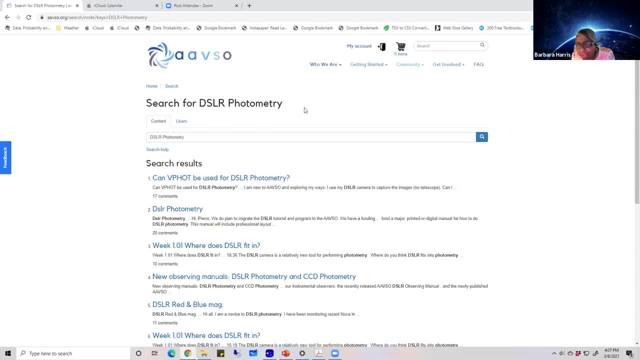 is that the 6.5 magnitude star or is that one the 6.5 magnitude star? So sometimes, if you're not sure, if you could plate solve your image, at least you can put the cursor over the star and determine what the coordinates are. and 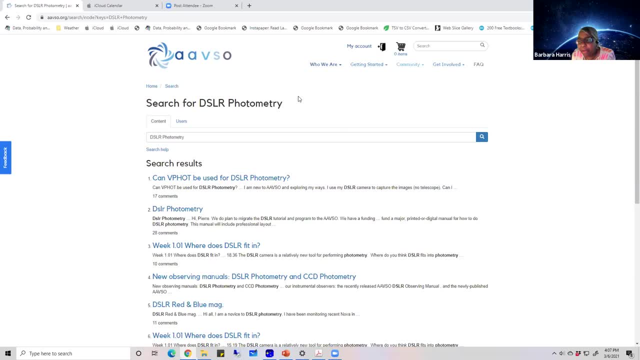 successfully identify what your comp stars and target stars are. But if you could accurately identify them by just looking at and comparing it to the AAVSO chart, then astrometry isn't going to be any more valuable in doing your photometry. Thank you. 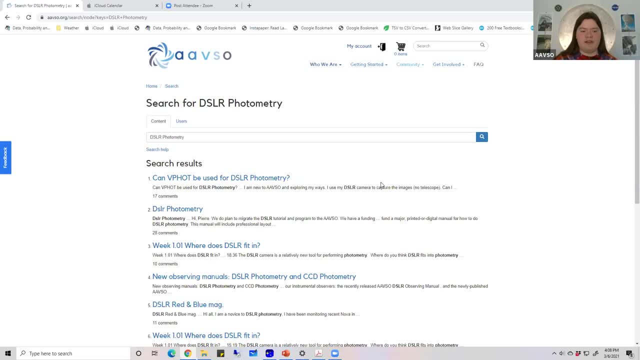 Next question is from Cameron Ewing, who has asked: when you're choosing a lens, for example an 85 millimeter, would it be better to choose a more expensive lens that goes all the way down to f1.4, or is a lens that goes to f1.8 or f2.0? fine, 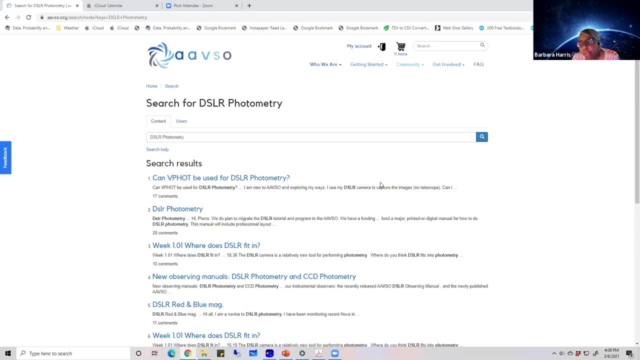 If I had a choice, I would choose like an f2.0 lens, Like I wouldn't go below that if you're doing it for photometry. Thank you, And our last two questions here are from Patrick Cavanaugh, who first asked. 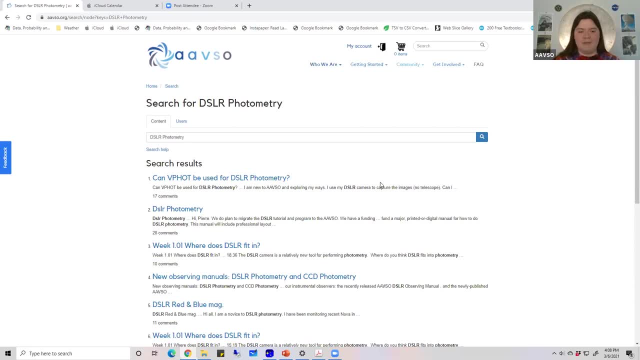 can you tell us about your exciting discovery doing DSLR photometry? There might be a most missing from that sentence. Well, I'm not sure I have any exciting discoveries of doing DSLR photometry. For me, it's just knowing that I'm contributing to and giving additional knowledge about a particular star. 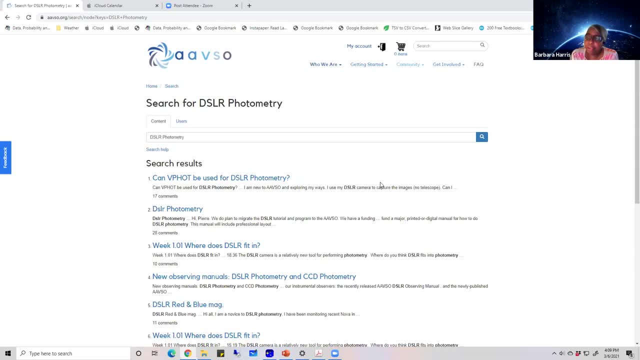 And especially if it's a nova. like I said, I got started in DSLR photometry Because of a Nova and Sagittarius And I was so excited about that Nova and not knowing what it's going to do and how bright is actually going to eventually become. 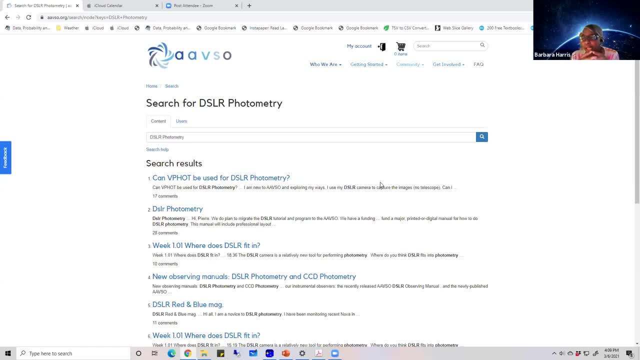 So it's kind of exciting to follow something new like that, not knowing exactly what it's going to do. But every time you do photometry on any star, you're basically just adding to the database and knowledge of that star And you know. 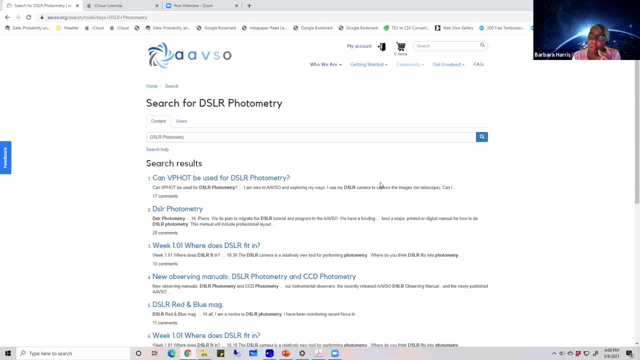 they can figure out things that they didn't figure out before by looking at the photometry over time for that particular star and seeing something that they hadn't seen before. So it mostly is just the knowledge of contributing to science and being able to discover something new. 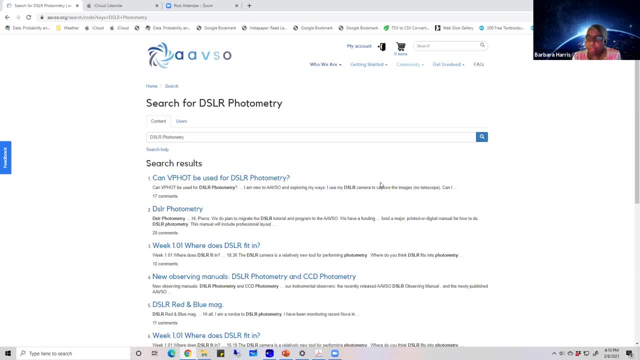 And, like I said, one of my favorite group of variable stars are eclipsing binaries And I like eclipsing binaries And some people say: well, if you know the time of minimum of a particular eclipsing binary, why do you do measure it every? 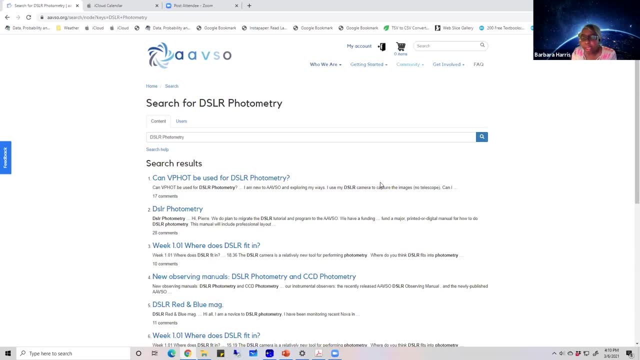 you know, and then calculate the time of minimum And it's like: well, we, we think this is what is the time of minimum, It's supposed to happen at that time. But there are some, there's something called O minus C diagrams or charts for eclipsing binary. 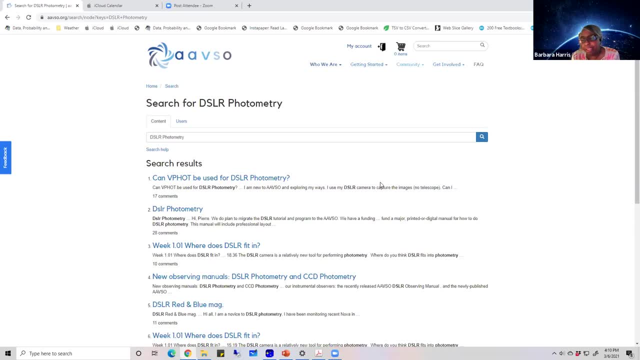 And what they do is every time somebody does a light curve for an eclipsing binary and they calculate what the time of minimum is. it might have been different than what the predicted time was, So I haven't done my light curve for algol that I captured a few nights ago. yet 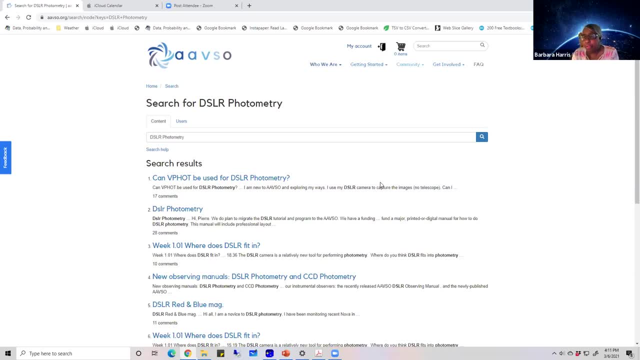 But like the AAVSO, predicted time of minimum was 207 universal time And suppose I have when I get my data, that is 235 universal time. That's the time of minimum. So there's an O minus C, calculation observed minus the calculated value. 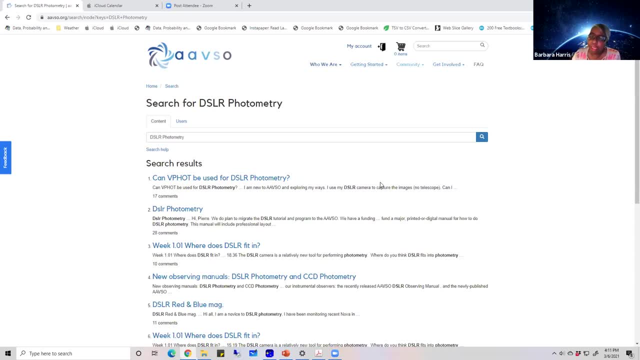 And when they plot that, those numbers over time, the observed minus calculated times, when they start plotting that, there's a pattern That can can be observed with that And that pattern tells us what may be happening Like: why is it off? 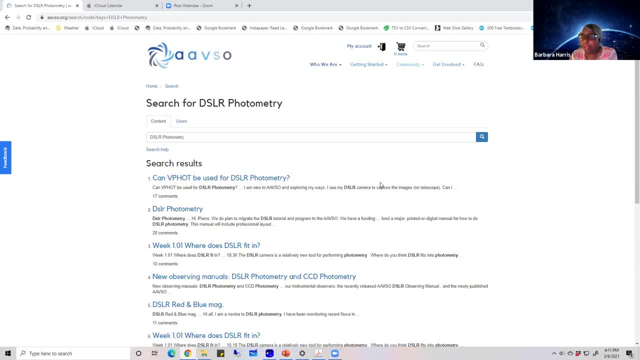 Like why wasn't it at 210?? And why, you know why is it 20 minutes off? And it could be because there might be another star in the system that they didn't know about, Or there could be a planet in the system that they didn't know about. 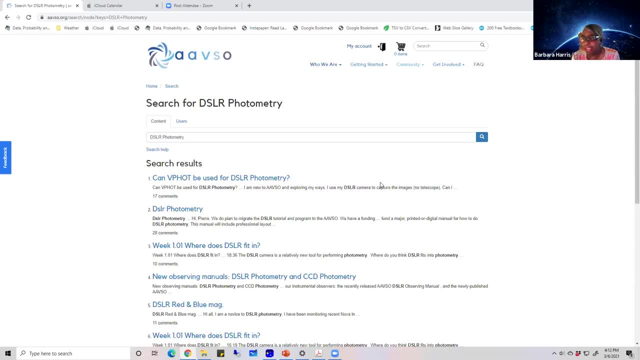 Or there could be mass transfer between the two stars that they didn't know about. So every time you're collecting data, you're adding to the knowledge of what's going on with that star, And to me I find that exciting. That is very exciting. 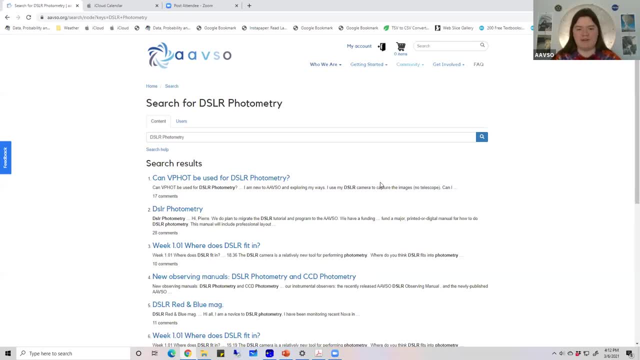 Thank you, And I'd like to mention, while we're on the topic of eclipsing binaries and O minus C diagrams, that there will be a how-to hour which is devoted entirely to those topics. It's scheduled for October 2nd. 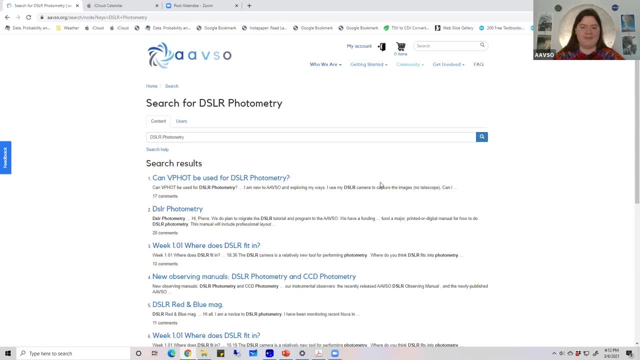 and Gary Billings will be the instructor. So for those of you in the audience who find that topic to be fascinating, make sure you tune in then. All right, So next question here from Patrick Cavanaugh. He said photometry entails a lot of work. 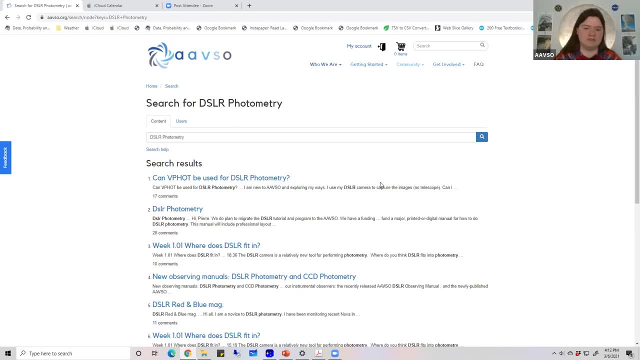 What has kept you personally motivated over the years? And if that was the answer, Kind of just what I just talked about. I just find it exciting contributing to the knowledge of, of what's happening with the star. Like I, have friends that love to do astrophotography. 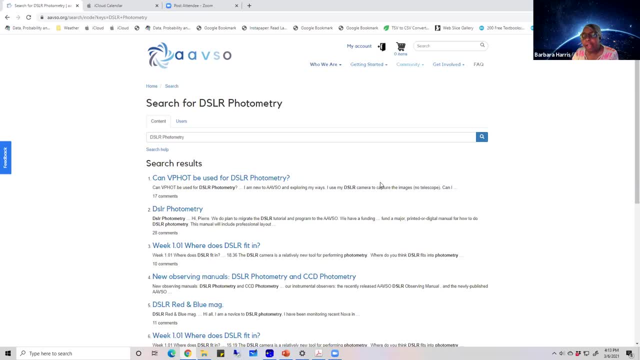 and they love galaxies and nebula, And I look at just an image of stars and I love individual stars, Like each individual star has the tail to tell And I just like that. you know, you see these white dots and everyone is a different person. 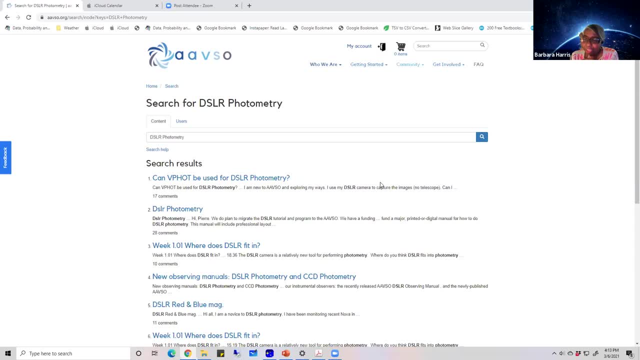 Everyone has a different tail to tell, And I I just find that fascinating. I can see why. Thank you. So we did actually have two technical questions come in while you were answering that one, One from Timothy Weather who asked about coma. 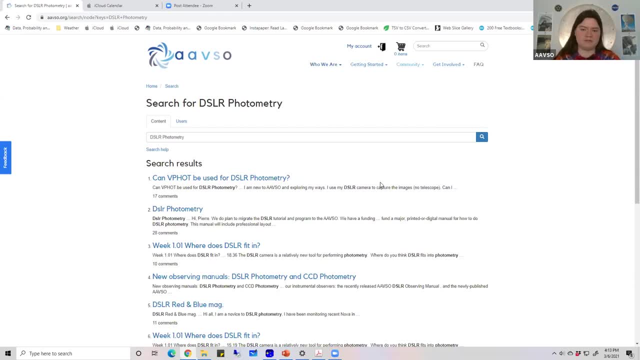 and if that's an issue when you're shooting at a low F ratio, Um, um, theoretically it should not be. Yeah, it really should not be if there's not a huge amount of it. Thank you, And another question came in from Wayne Clark. 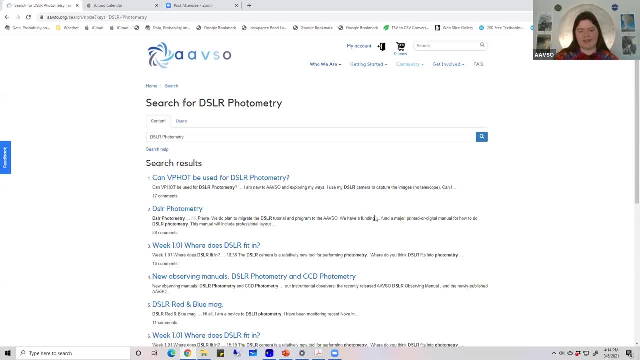 who asked if a skylight filter will affect the photometric accuracy. You really for DFLR photography. you really shouldn't use any other filters Because it will affect the commentary. Ideally, you should just use the the filters that are there on the camera. 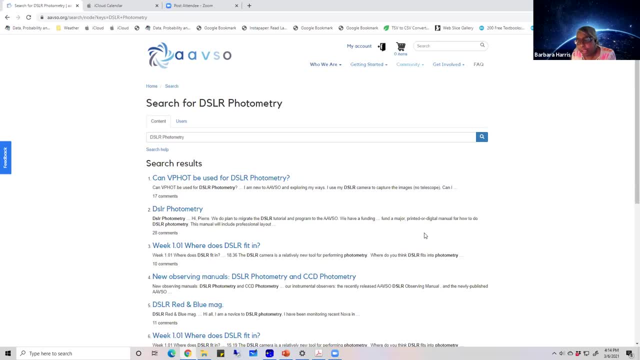 Like they. there's IR blocking filters and just the color filter array. You really shouldn't add any other filters to to the system because theoretically it can affect the photometry. That makes sense. All right, Thank you, And that was the last of the questions that have come in. 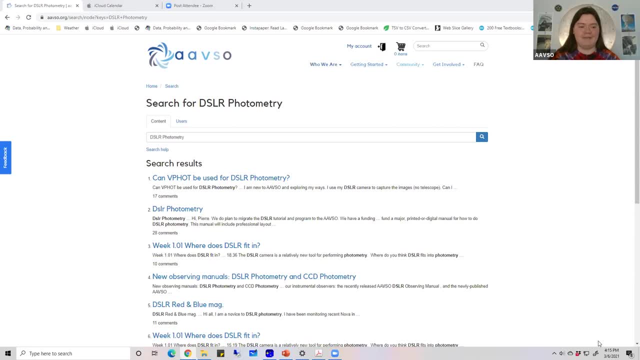 Now we do have two outstanding here that you will see from Thomas Erzinger and Patrick Cavanaugh, saying thank you for an excellent presentation. You're very good at this and extremely easy to follow. I have to second that, and I know that there will be a lot of other attendees who agree, because those 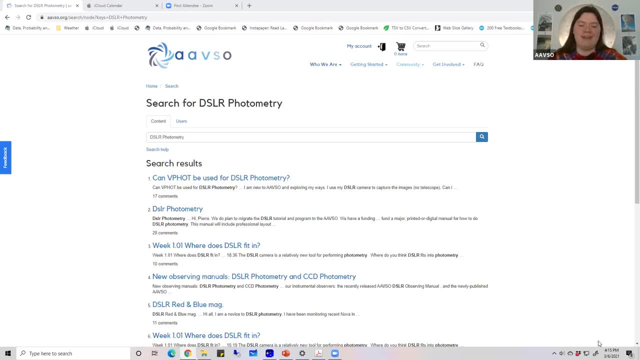 kinds of comments have been coming in in a flood during our Q&A, And I would like to say just thank you so much For sharing your time and knowledge with us today. This was a fantastic session. Well, as you can tell, I love doing this. 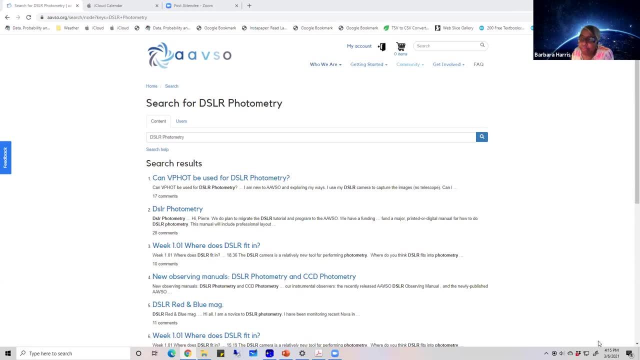 It is basically been like a new career for me. I had to stop medicine because of a heart condition, And as much as I loved medicine and how hard it was for me to stop practicing, What, like they say, when one door closes, another one opens. 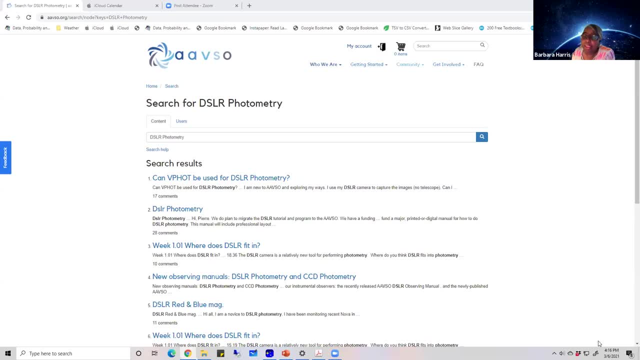 So, even though I can't do medicine anymore, it basically has given me a whole career in doing astronomy and photometry Because, like with my CCD photometry, I do a lot of alert notices and I follow do a lot of campaigns. So if your data 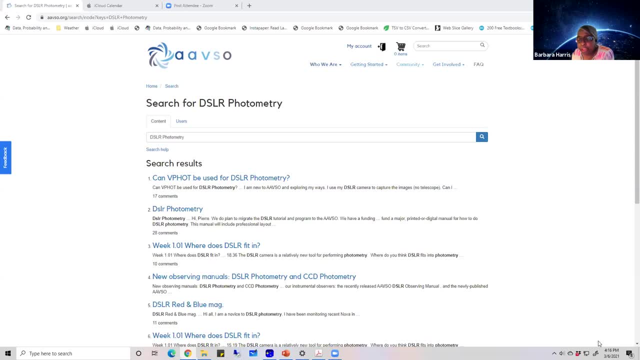 if your work is good enough, you're, you're contributing data For these professional astronomers and I have been involved with many publications And you're, so your name goes on the publication because they've used your data. So I actually have more astronomy publications than I have medical publications. 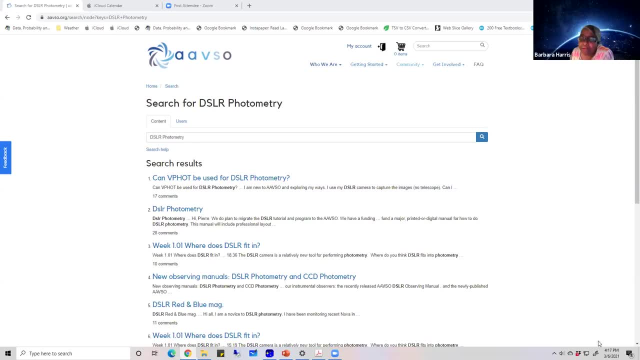 So so it's. it's been a lifesaver for me having to give up a career. It basically has opened up another one. That's that's fantastic. Thank you so much for sharing And for those people that they really want to get involved. 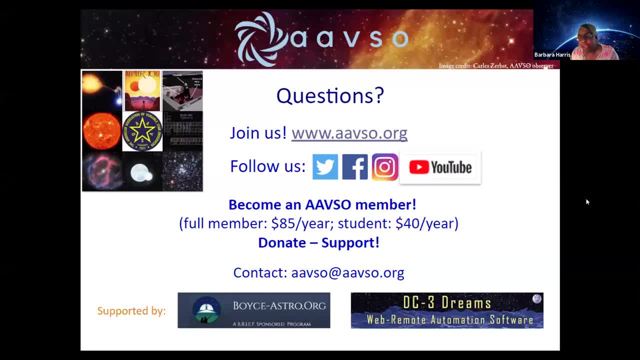 Like I said, it's hard for me to teach the dslr choice course, but I do mentor dslr and theoretically I can do CCD also, but they they have trouble getting enough dslr mentors, So I mostly do dslr mentoring. 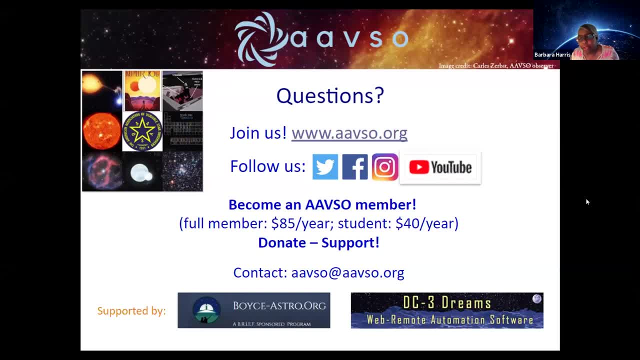 So I don't mind doing individual Mentoring and I noticed what at the beginning- that I saw several people that I had mentored on online here. Very nice, Thank you, We everything that you do for the AVSO Okay, and I'll prepare my slides and send them to you and you could find a place to share them. 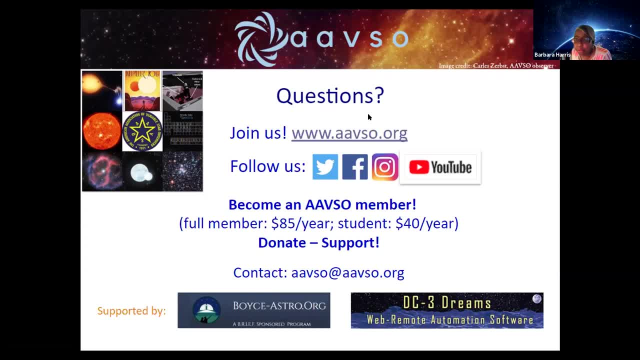 Absolutely, Or or email them to everybody if they're interested. Absolutely, Thank you, Okay, All right, Bye everybody. Thank you, Goodbye, Dr Harris. Thank you, Bye-bye. Okay, Now, before I close the webinar. 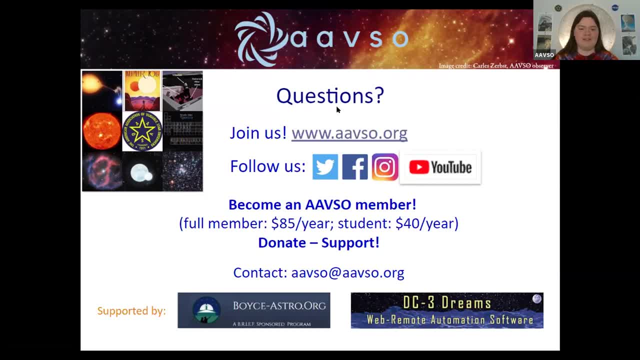 I would like to give a final thank you to our sponsors, DC3Dreams and Voice Astro. DC3Dreams provides high-end observatory automation and web-based multi-user remote imaging. The AAVSO net observatories use DC3Dreams ACP expert for the bright star monitors and other programs. 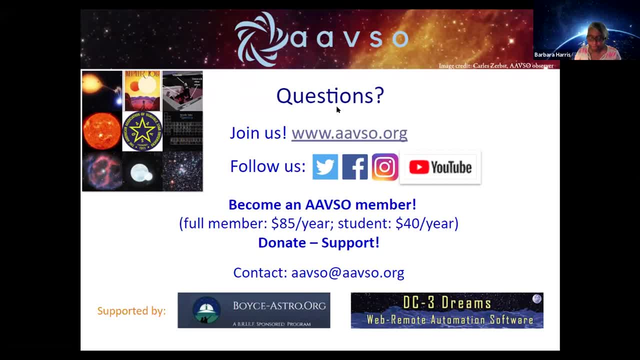 The AAVSO photometric all-sky survey project, also known as APAS, has used ACP experts AI scheduler to automatically acquire over 500,000 star fields hands-off, at a rate of a thousand square degrees per night. This has resulted in photometry for over 128 million objects in about 99% of the sky. 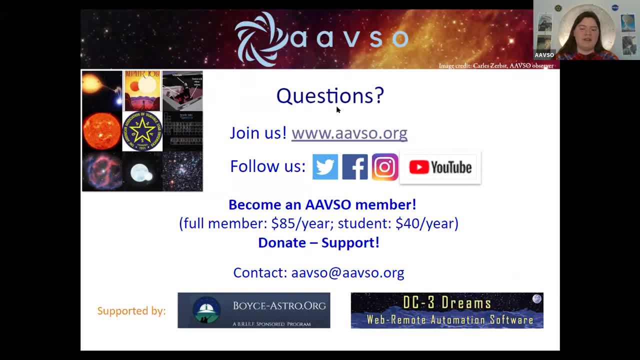 The Boyce Research Initiative and Education Foundation provides online astronomy education, observatory resources and research experiences to students, student teams and schools in order to learn how to perform observations, conduct research and publish their results in scientific journals such as the Journal of the AAVSO. 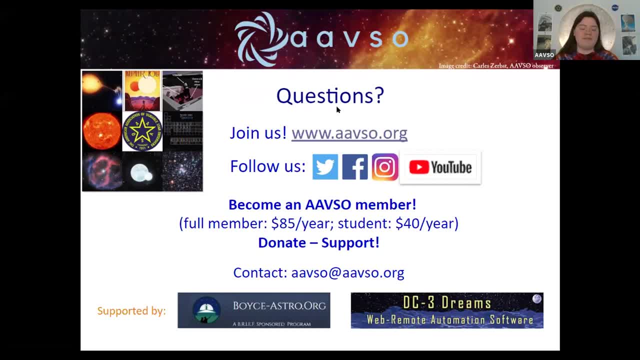 Today's webinar has been recorded, and this recording will be made available for free on the AAVSO's YouTube channel. You can find a full library of webinars just like these on our YouTube channel. Go check it out While you're there. 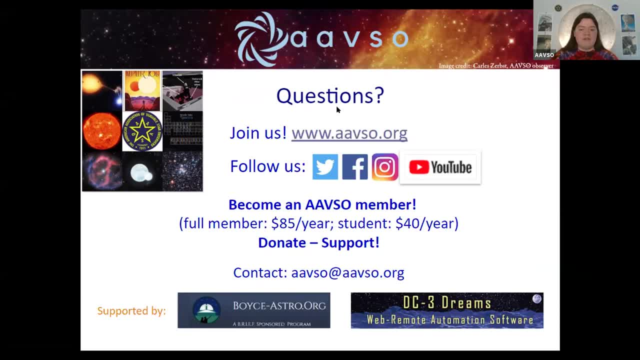 consider subscribing to our channel, because then not only will you get notified every time a new lecture is posted, but by hitting that little subscribe button you will be increasing our educational reach and making YouTube more likely to suggest our videos to others. So this is just one more way that you can help support the AAVSO. 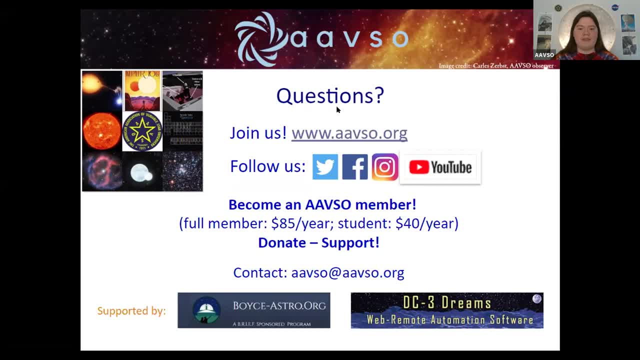 Speaking of support, this webinar series is being supported by you, the viewer, So please, if you're not a member, join the AAVSO. AAVSO membership comes with a wide array of benefits, including free access to the mentorship program. 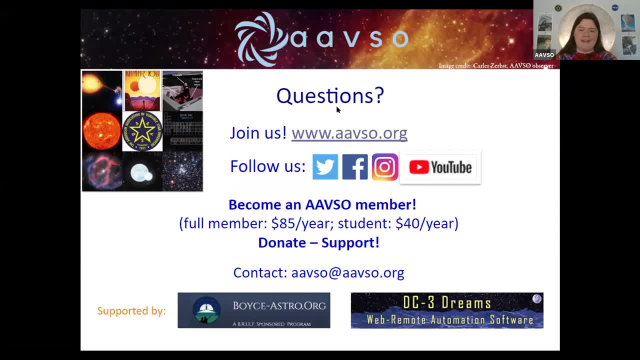 as we've been discussing tonight, And that is absolutely a great place to go if you're wanting to get really involved in DSLR photometry And maybe, if you're lucky, you'll get Dr Harris as your mentor And if you are already an AAVSO member. 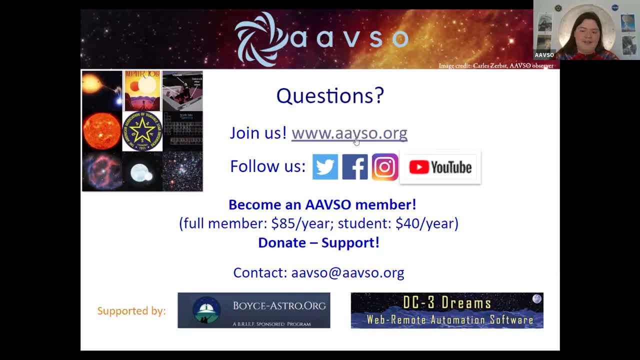 don't forget to renew your membership And, of course, we would be grateful if you would consider donating to the AAVSO. Every donation matters and goes towards making programs like this come to life. One last thing before you go, After you leave the webinar. 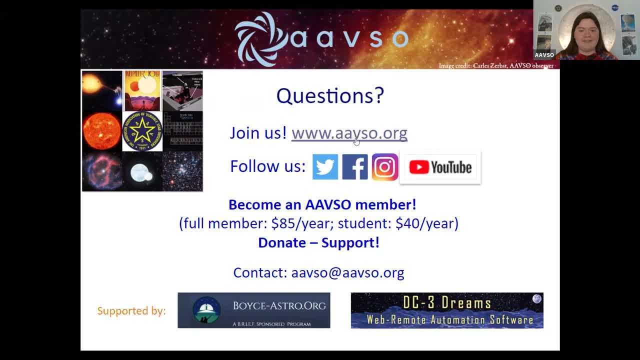 you will be automatically directed to a survey. Please do fill it out. We want to hear your feedback. You are more than welcome to fill it out, even if you've already filled out a survey at a past AAVSO webinar. We do read every single response.